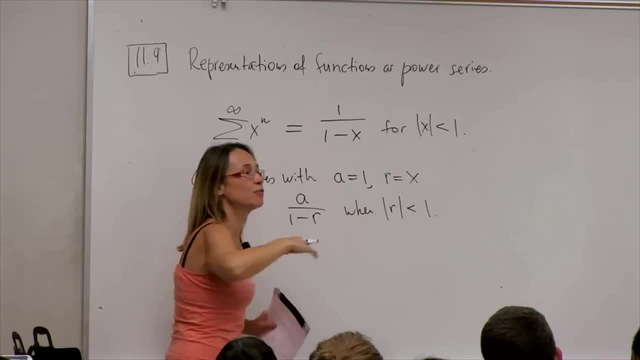 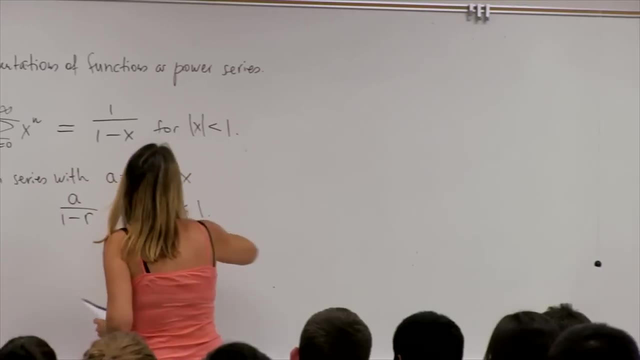 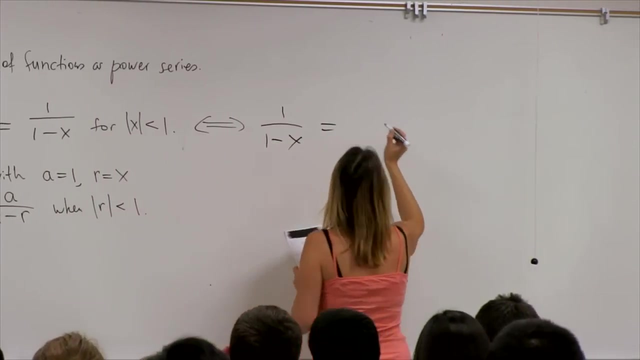 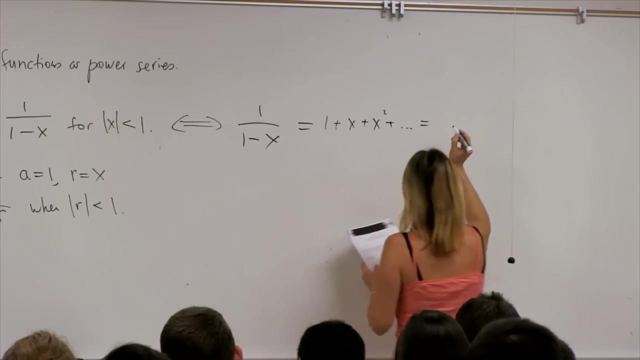 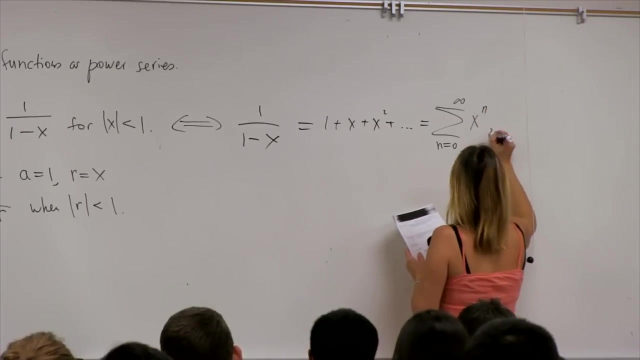 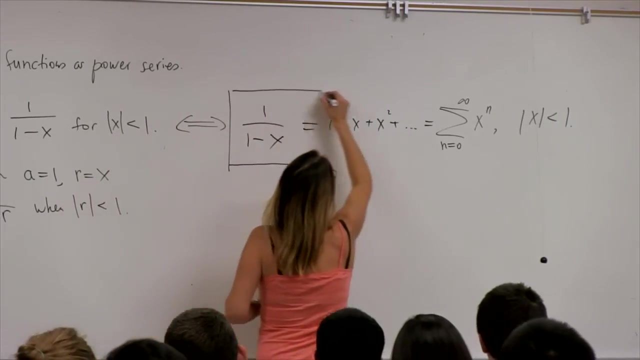 for x less than 1.. just, otherwise okay. so we cannot say what it's equal to. fine, this is an old result. we've already seen that. I'm going to rewrite it in a different way. very similar, though okay. so this is probably the most important formula for today: a very 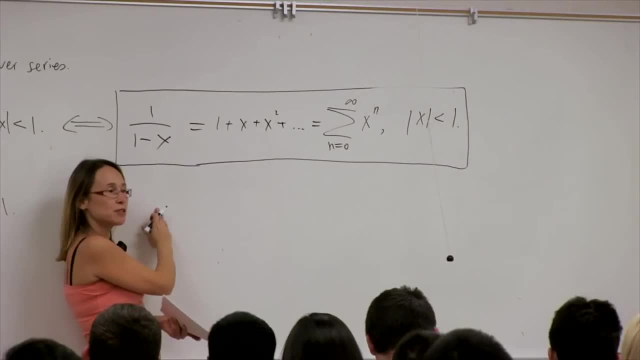 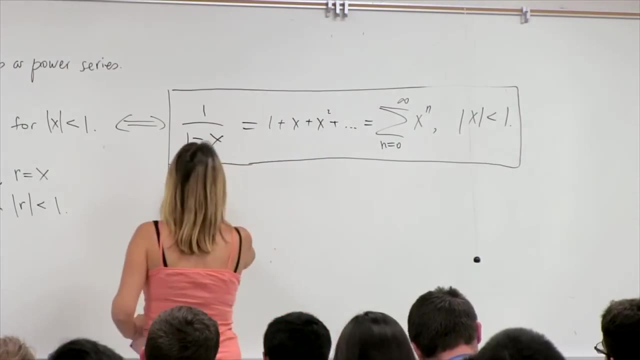 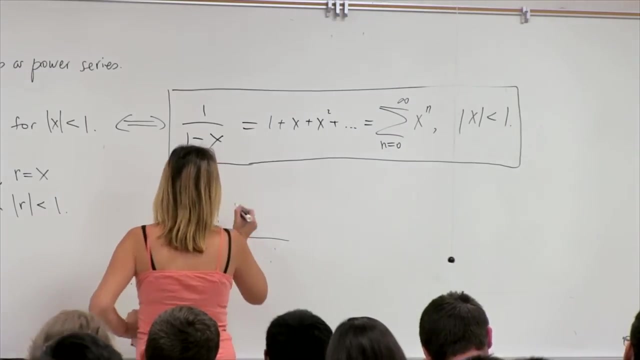 simple one. so we're going to think of it in the following way: on the left I have a function of X, the function everybody knows what it looks like. right it's 1 over 1 minus X, so somehow here it has a discontinuity. looks like this: 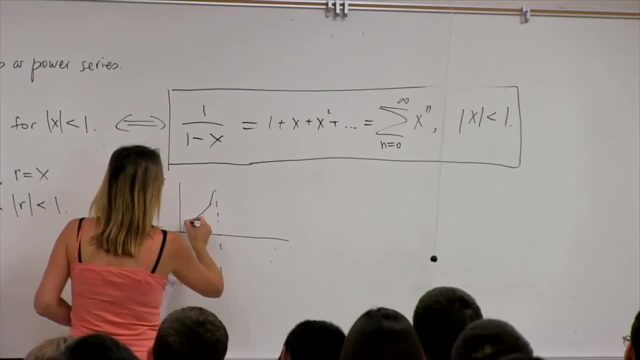 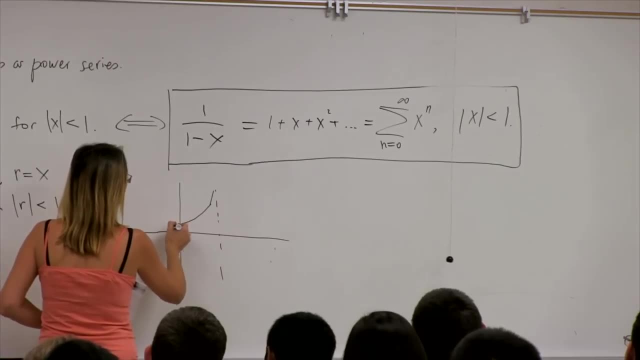 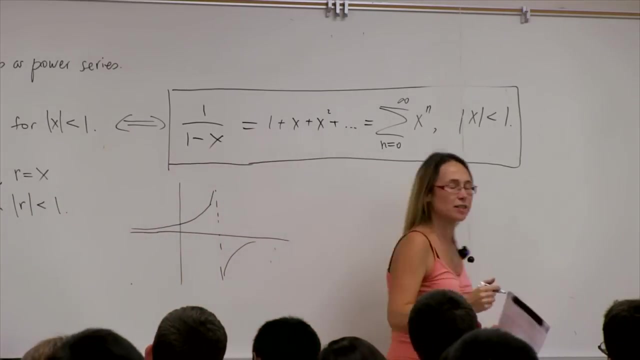 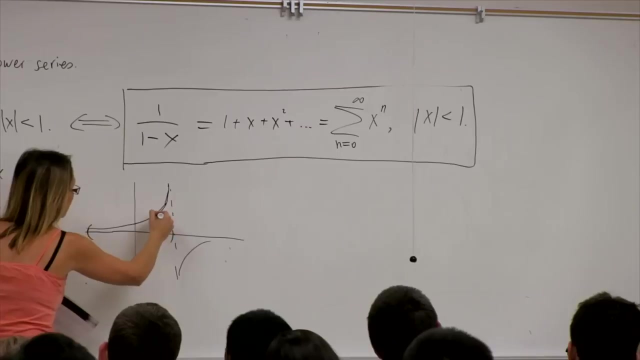 so when X is equal to 0, it's equal to 1, and then it continues here like this. so a function like this: okay, we restrict ourselves to the values of X between minus 1 and 1. okay, not including. so we have a function that looks like this: 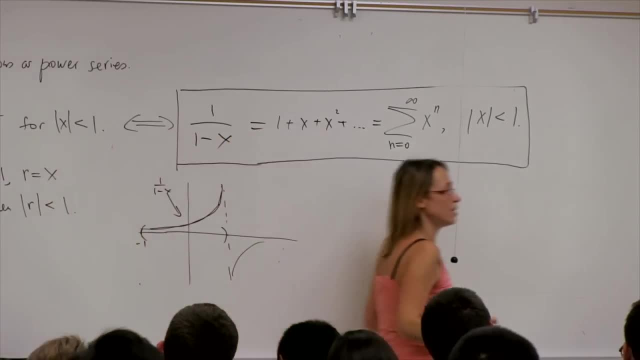 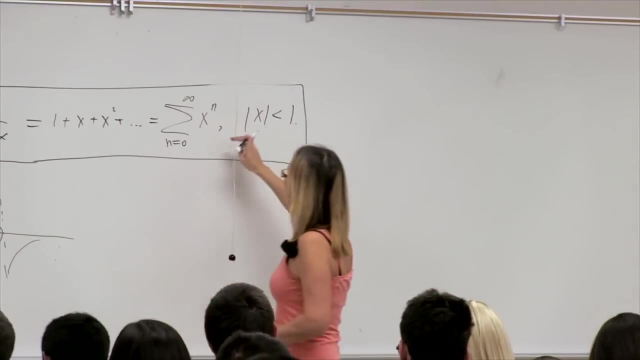 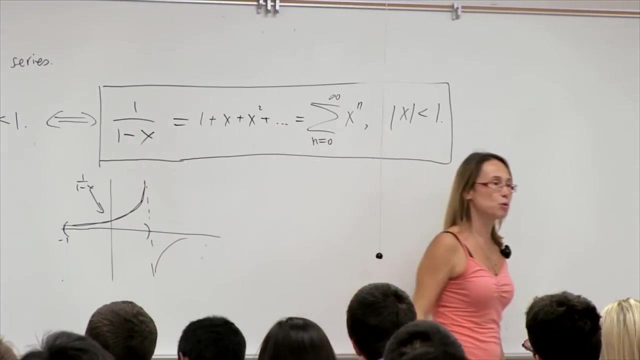 that's what we have on the left. on the right, we have an infinite series, we have a power series, so somehow a function is equal to a power series. so it turns out that many functions can be represented in terms of power series. this is not the only one, okay, and 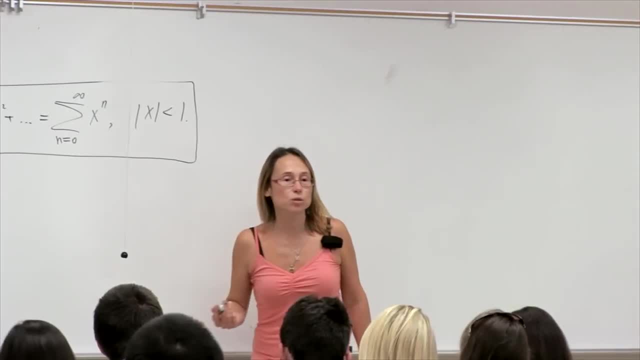 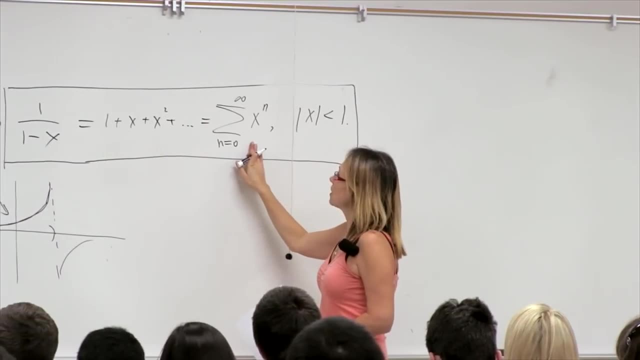 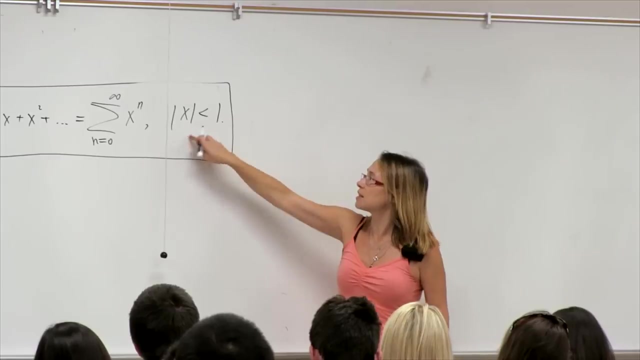 whenever we can do that, we can also calculate the radius of convergence, so it's not like I can always say that the left hand side is equal to the right hand side. this equality only holds for a restricted domain of X, but when the absolute value of X is less than 1. 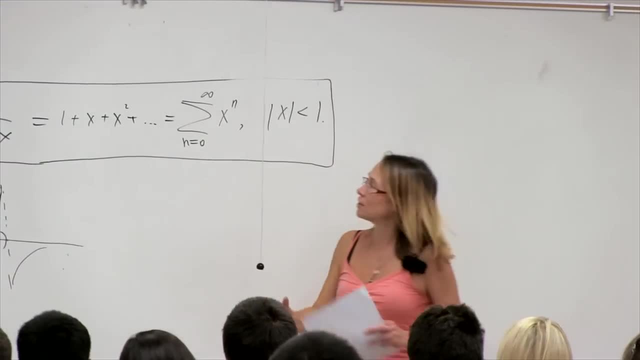 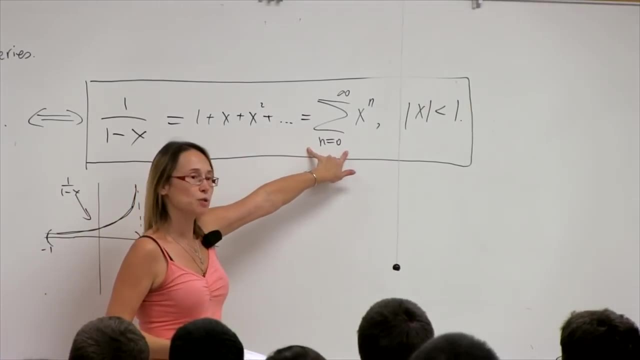 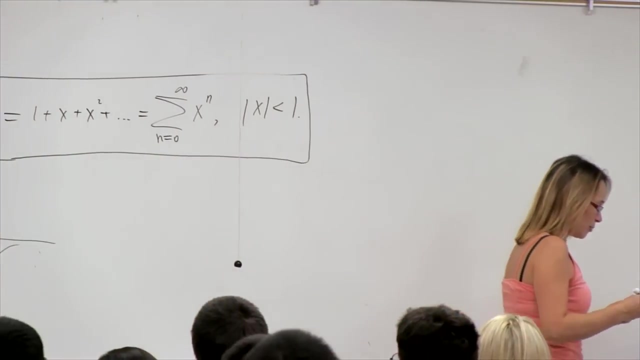 the left hand side does equal to the right hand side, and you can see that philosophically it's not easy to grasp. on the left, I have this really easy thing. on the right, I have an infinite number of terms summed up, but somehow they are one and the same. so let me show you what other functions can be represented in a. 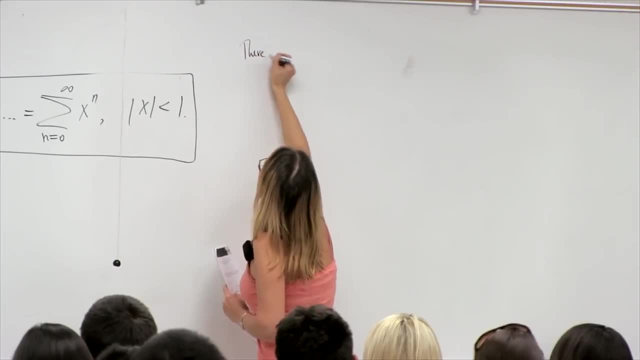 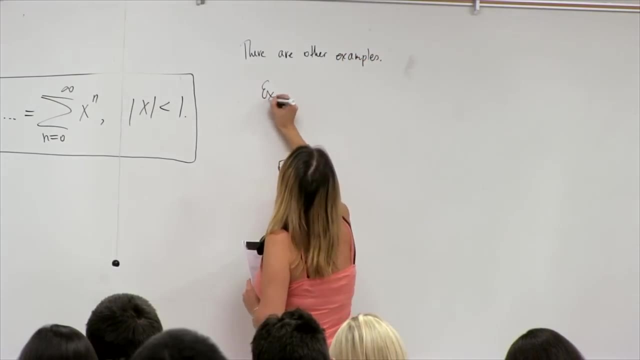 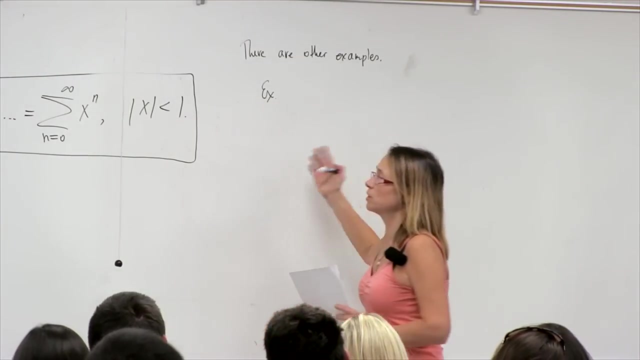 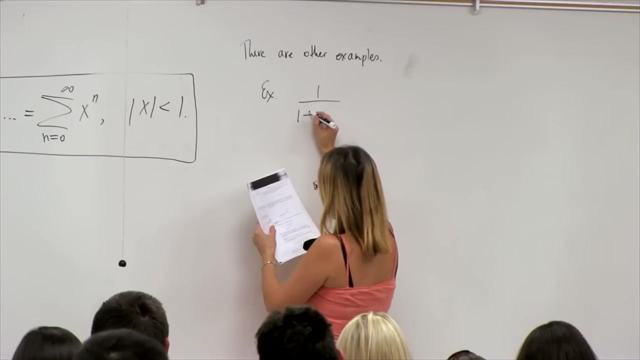 as power series. There are other examples, so very often, or sometimes at least, you can make a connection between the new example and this old example, so we'll keep coming back to this one. so let's suppose that my function is given by 1 plus x, squared like this: Can we represent this? 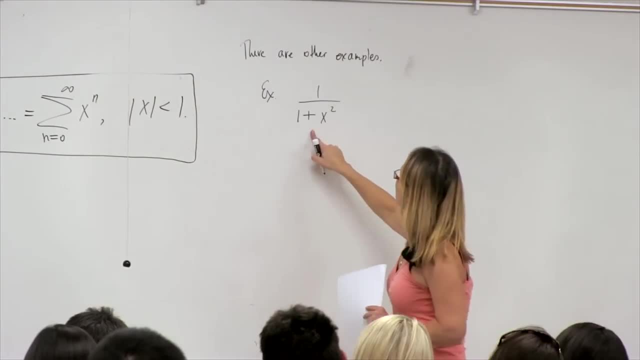 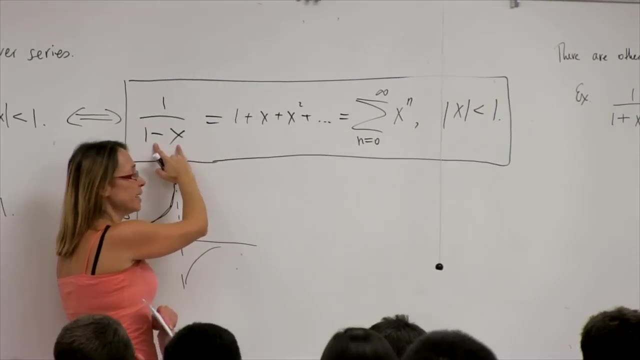 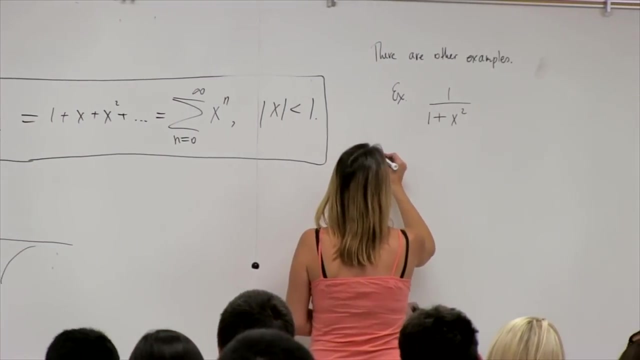 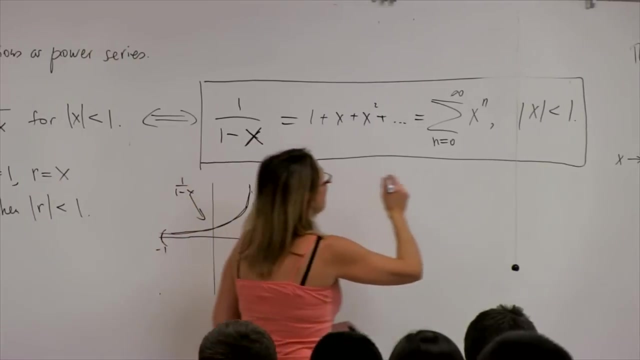 as a power series. Well, look at this function and compare it with this one. So if I, if I replace x with negative x squared, this becomes the same as this, right? so if I replace x with negative x squared, this known function becomes the same as this. 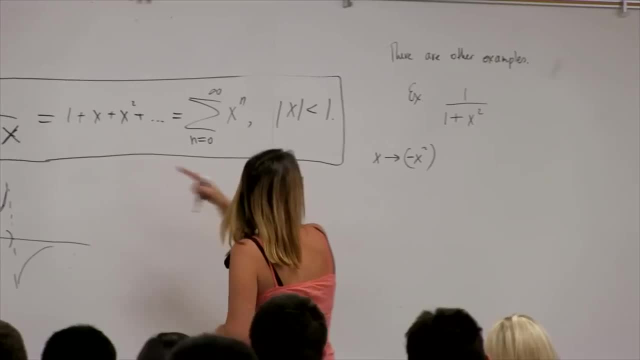 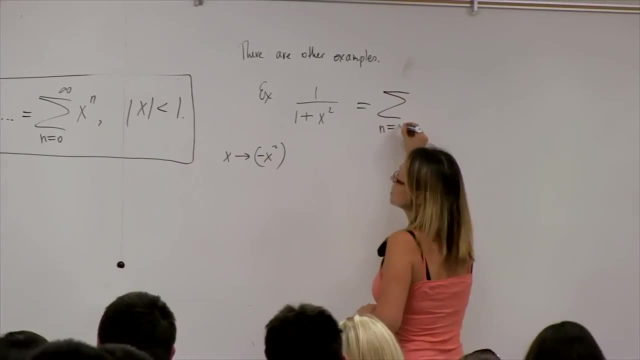 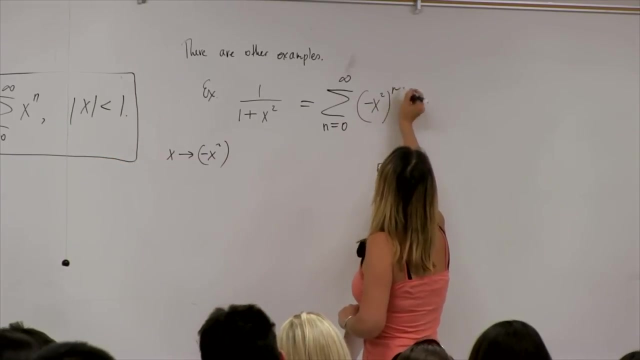 okay, so the left and side becomes like this. What happens to the right hand side here? I have again the infinite sum and instead of x I have to put negative x, squared right. so I'm just taking this formula: the left hand side and the right hand side. 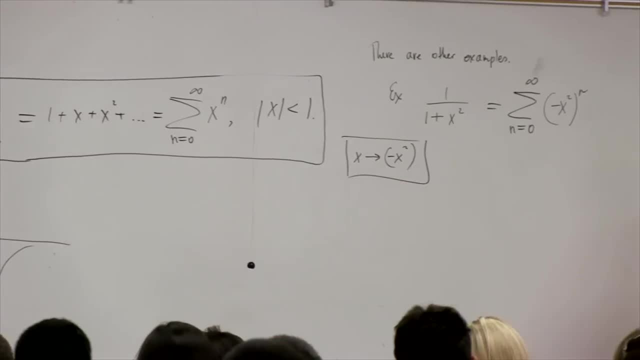 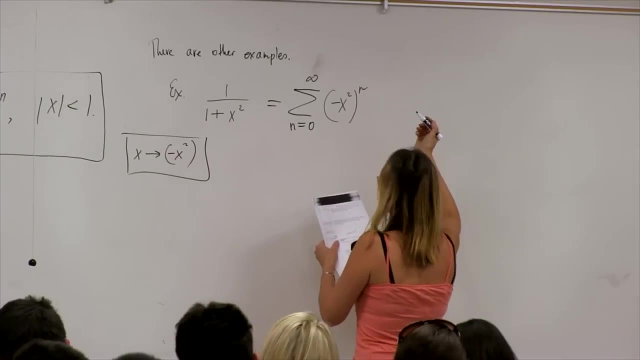 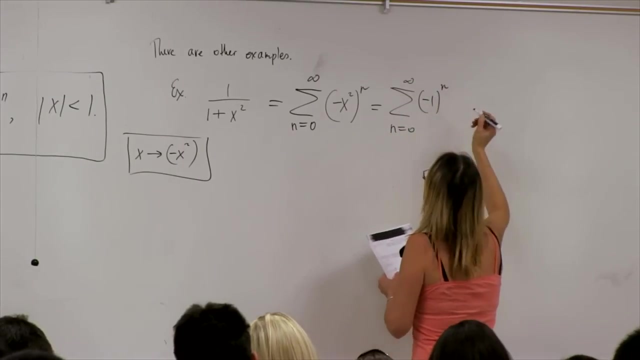 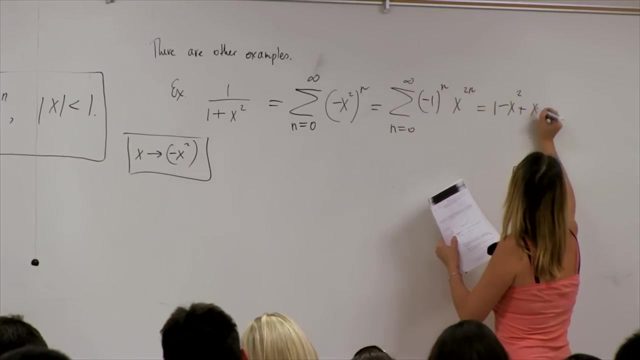 and I'm replacing x with minus x squared, and then on the left I get the given function and on the right I have this series representation and actually I can rewrite it a little bit differently to make it look more like a standard power series. so this is 1 minus x squared, plus x. 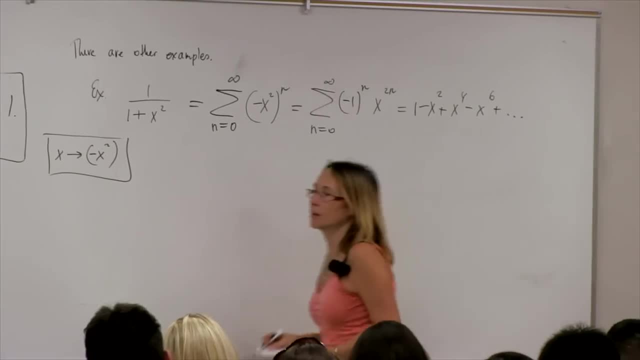 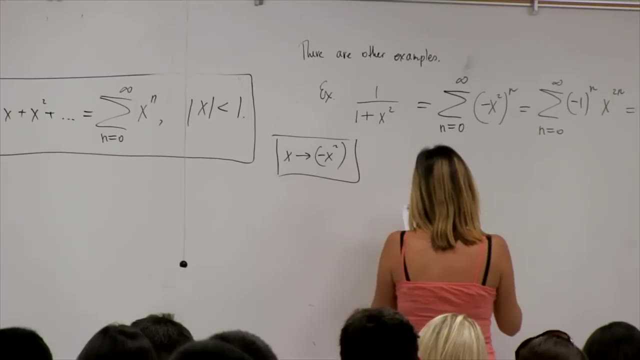 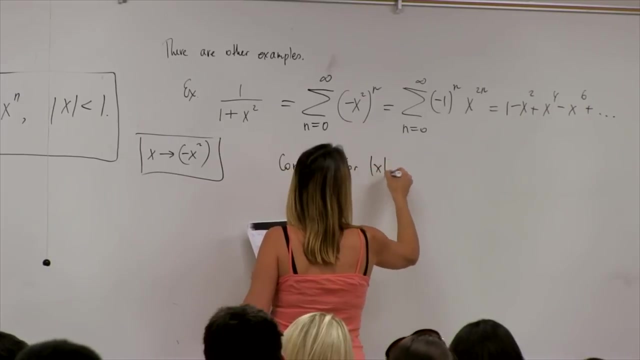 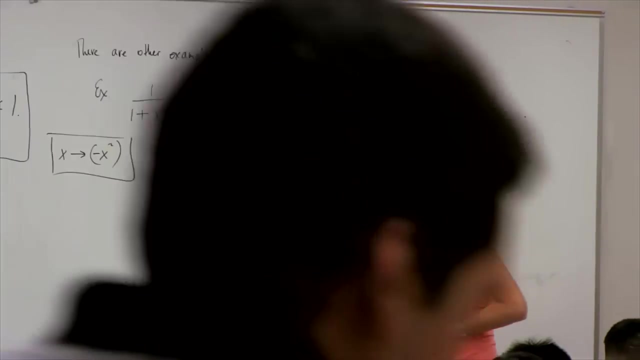 to the 4 like this: when does it converge? it converges, it has the same radius of convergence, converges for x less than 1, the same as the previous one. we can either apply the ratio test or think of it as a geometric series again. 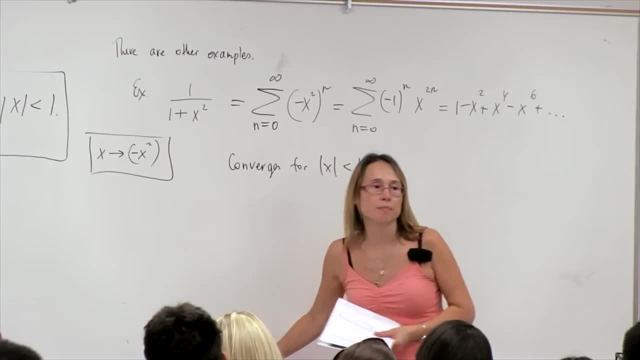 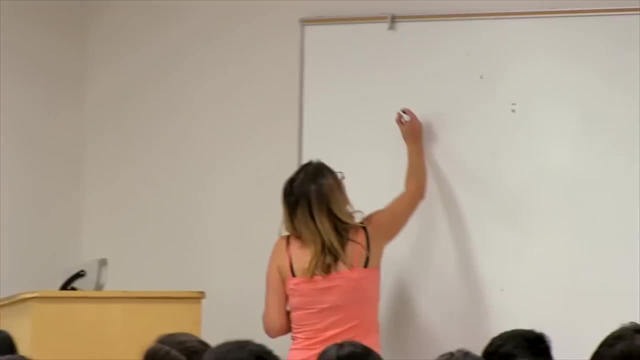 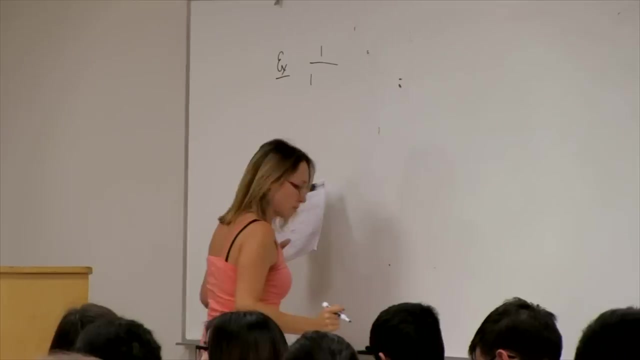 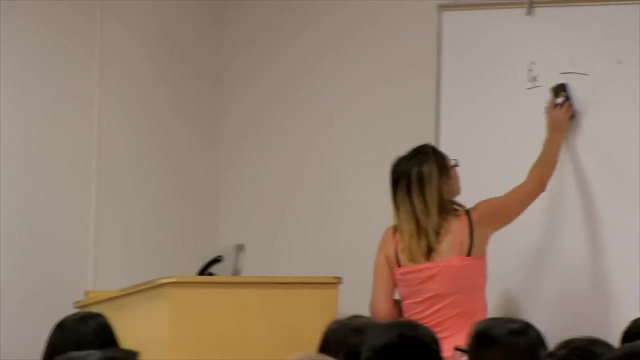 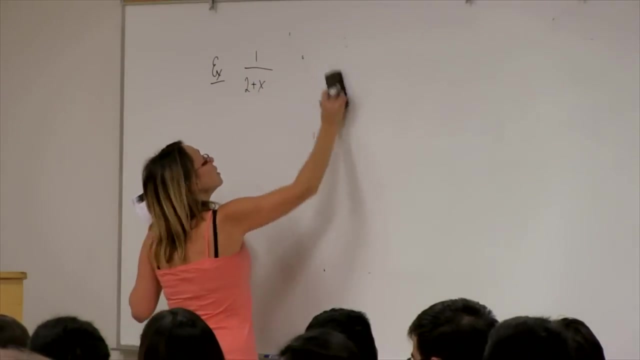 same thing. okay, questions. so I'm going to give you another example, which again will convert to that old one we can. let's consider the function x plus 2, 2 plus x. so somehow I want to make this look like the framed example. question. 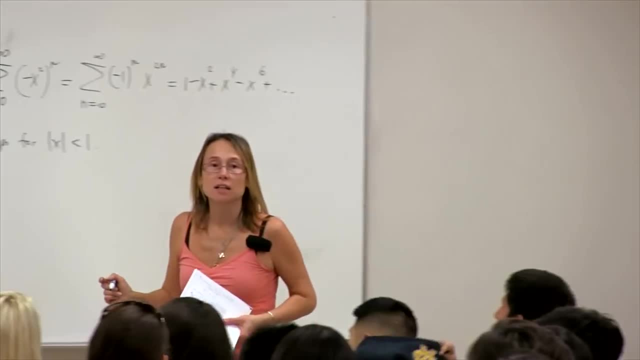 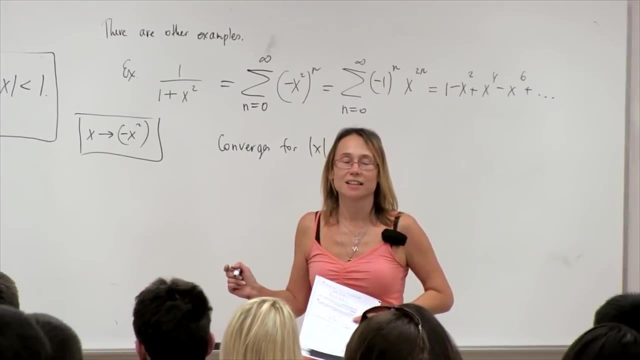 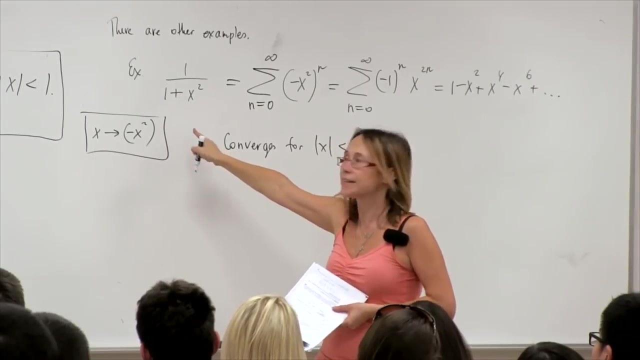 how are you doing that? are you just using no or smart? thank you, but what is the question? well, we need to be able to know like 1 over 1 plus x squared equals that, no, no, you don't have to know this, that that would be too many to memorize. 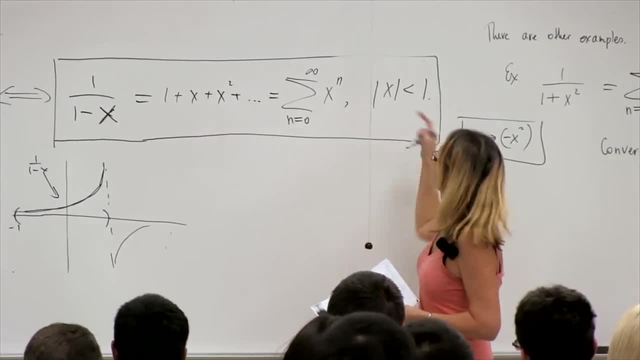 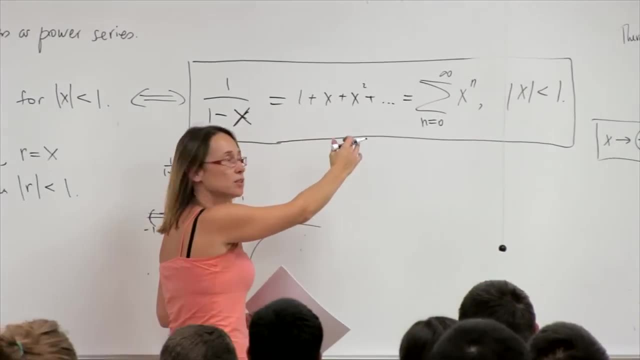 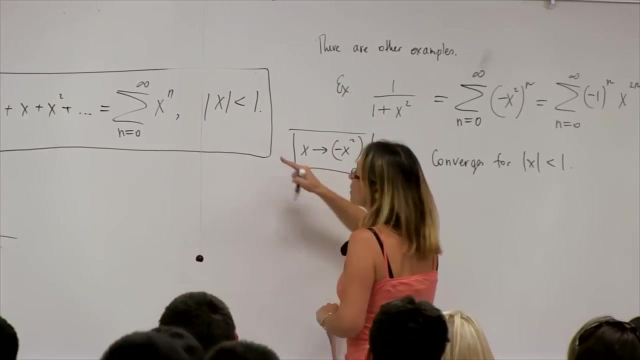 this one is easy to memorize. you should be able to sum this up as a geometric progression, as a geometric series- and this is one of the more important ones- and you can reduce this one to that one by identifying this term with this term. okay, here I 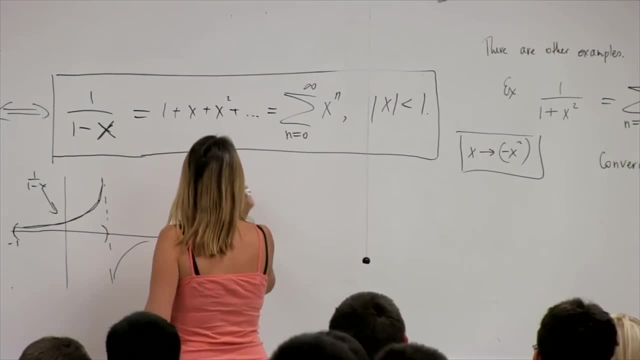 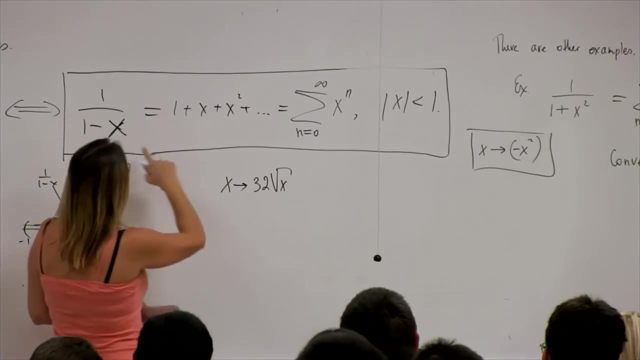 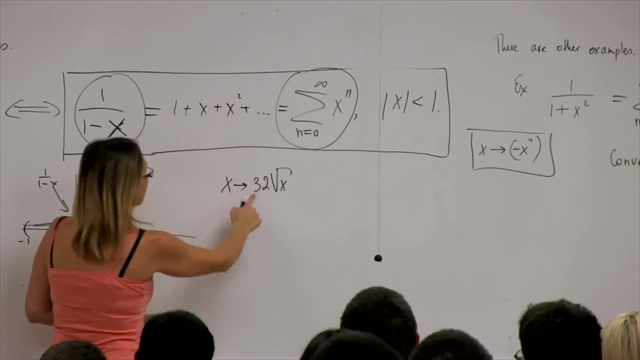 for example- I give you another example- we can replace x with 32 squared of x. okay, so let's do that. I take this equality this side and this side, and I replace x with this. okay, so what do I get? 1 over, 1 minus. 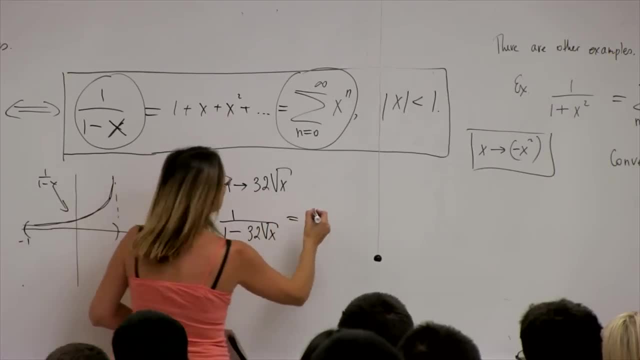 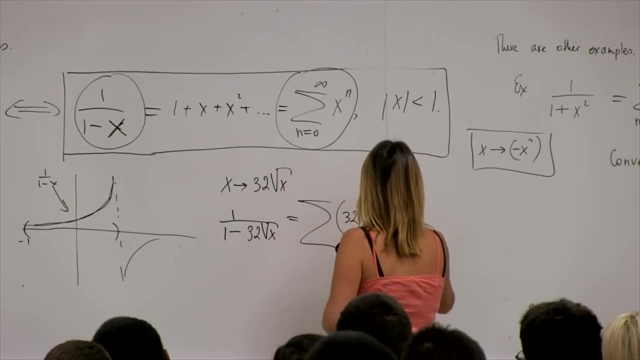 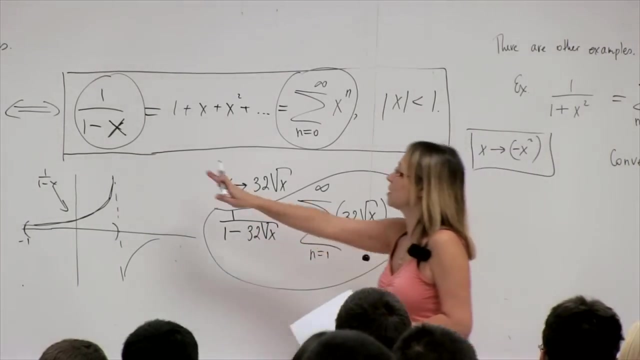 32 squared of x on the left, right is equal to, and here, instead of x, I put 32 squared of x to the n. okay, so this is how I can represent this function as a power series. okay, so this operation of identifying, of replacing. 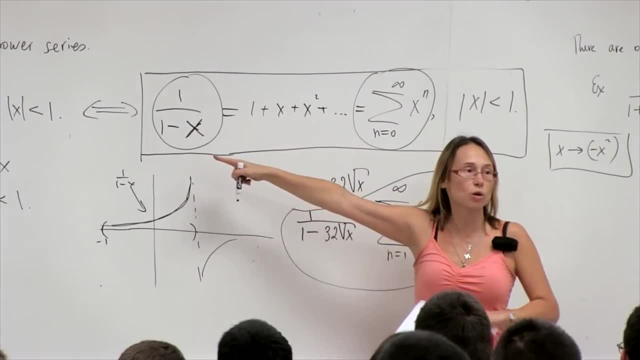 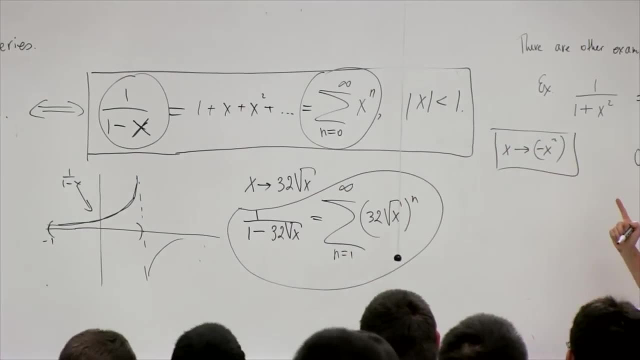 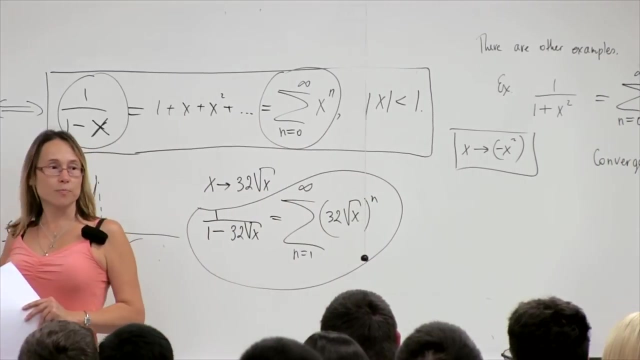 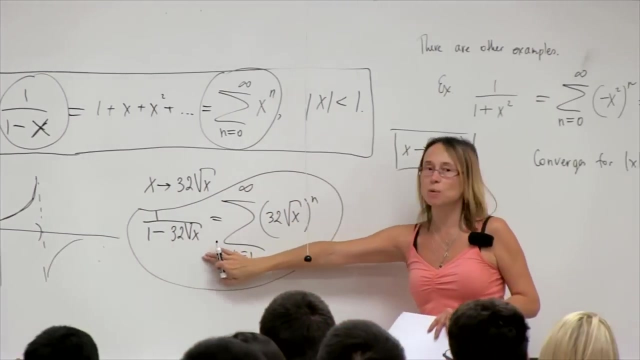 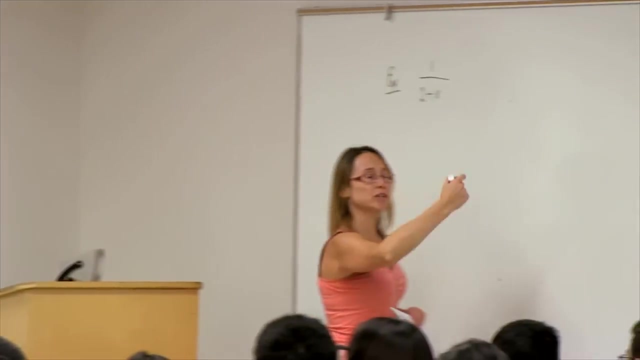 x with another variable. I could replace it with a or b or another letter, or with 32 squared of x or anything like this. right, it would still work. I just have to be careful about the radius of the x-axis. okay, and these are raining, yes. but again, we can do this equation- and we're going to use it previously, which we don't always do- to this issue- right, but again, we can imagine a series of convergence. this is again a geometric series and it only converges when r1 less than 1. okay, but I can perform this operation and get a lot of different functions and, of course, you cannot memorize them all. so, for instance here- okay- 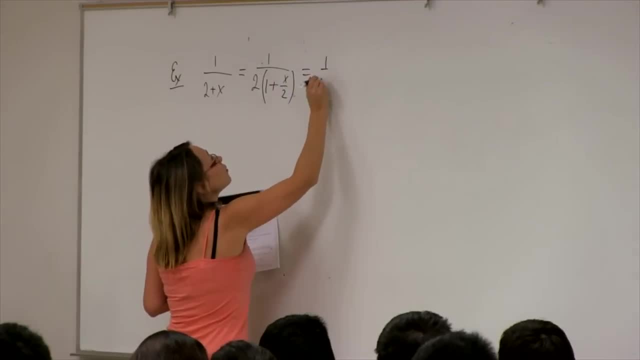 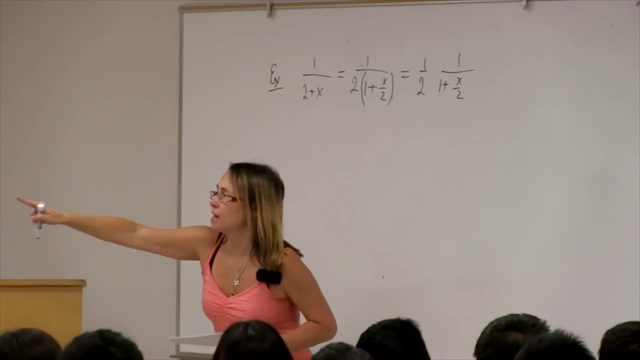 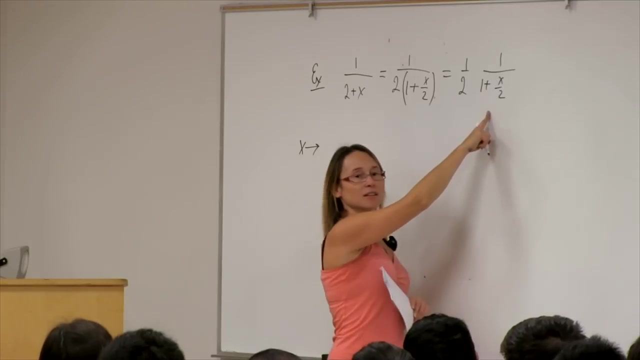 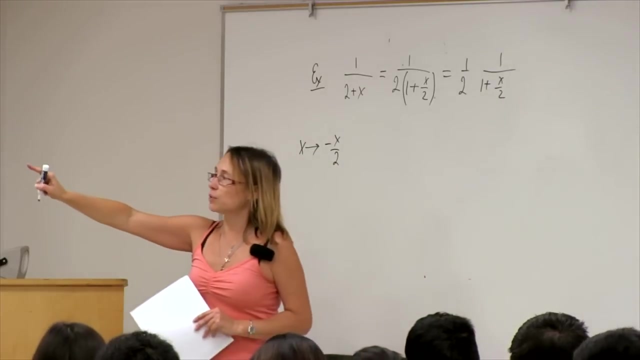 this. okay, then they have one half one plus X over two. so when I go back to my own old example, what replacement should I make? I have to replace X with what to make that example look like this: negative X over two, exactly. so this operation brings my old example to the new one, and I shouldn't forget about one. 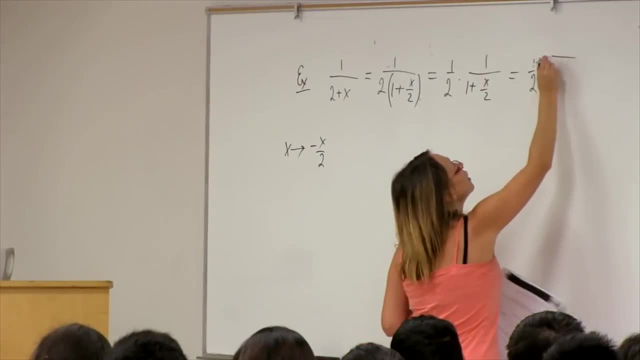 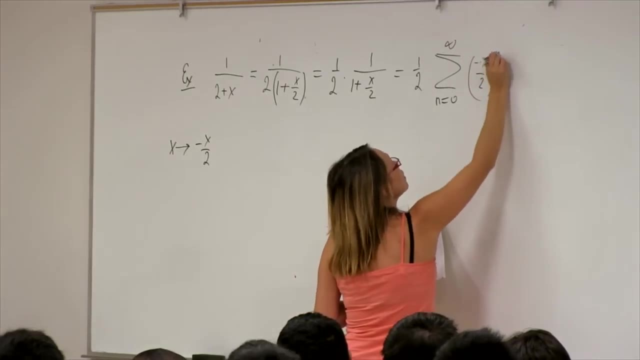 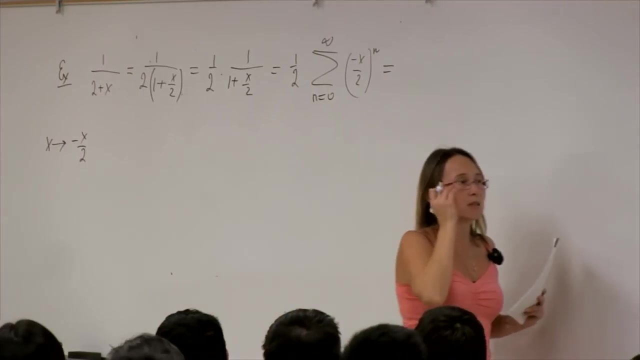 half. right, it's multiplied by one half, so I have one half. and again, instead of X, I put minus X over two to the N. okay, and I want to make this look like a power series. what's the power series? I should have coefficient CN like this: 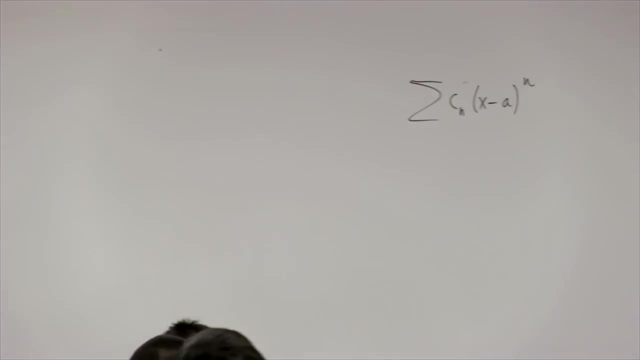 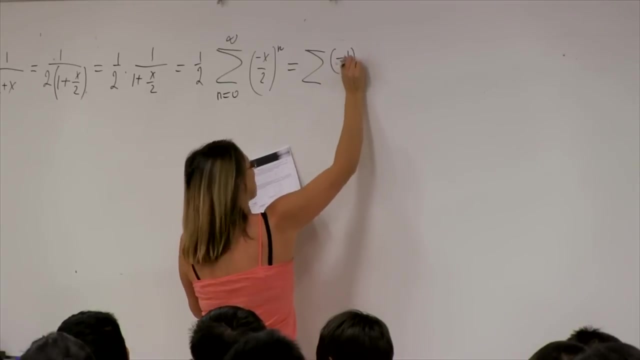 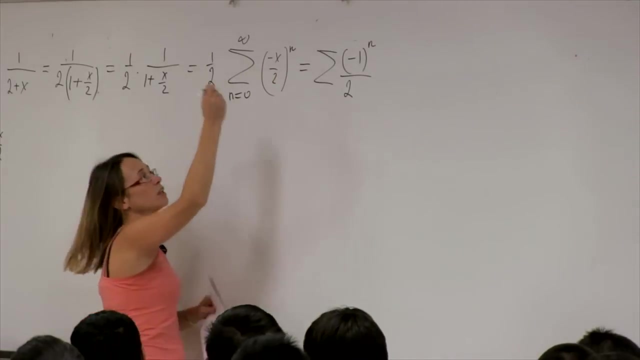 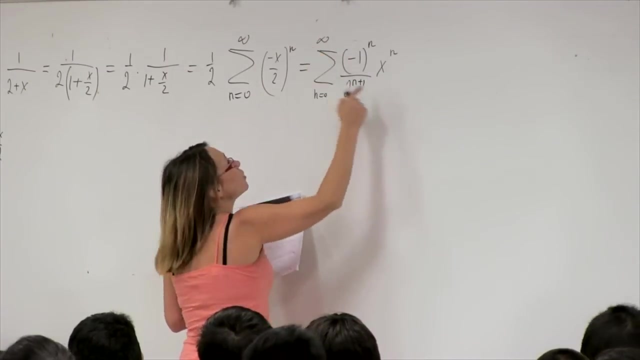 right, so this is not quite in that form, so I'm going to rewrite it like this: so I have minus one to the N, I have two to the N, plus one, I have an extra two here and I have X to the N. okay, so now it, it is a power. 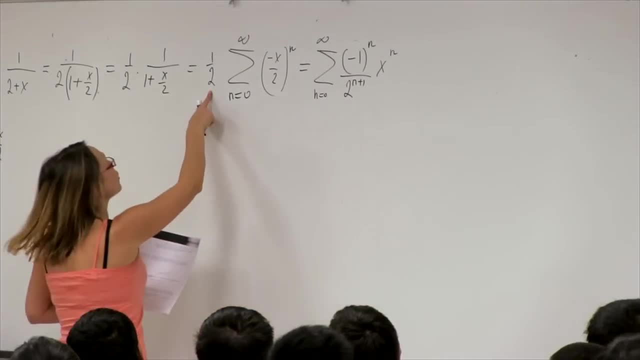 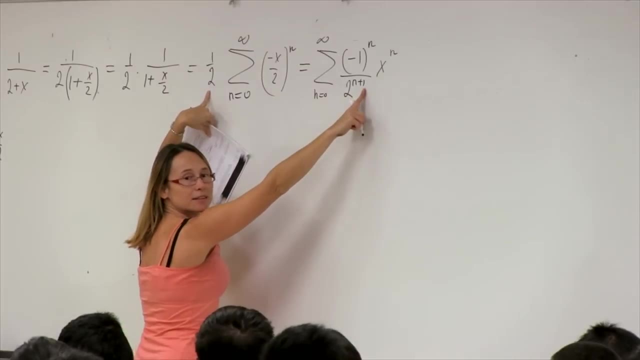 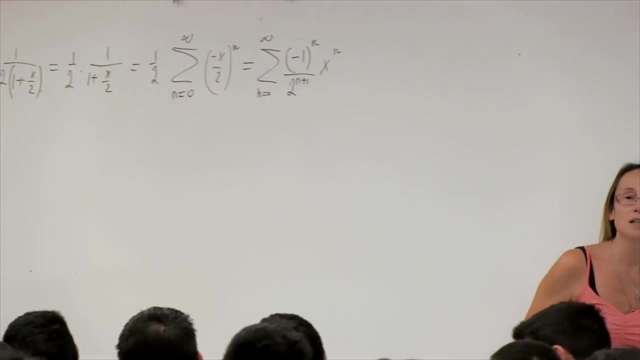 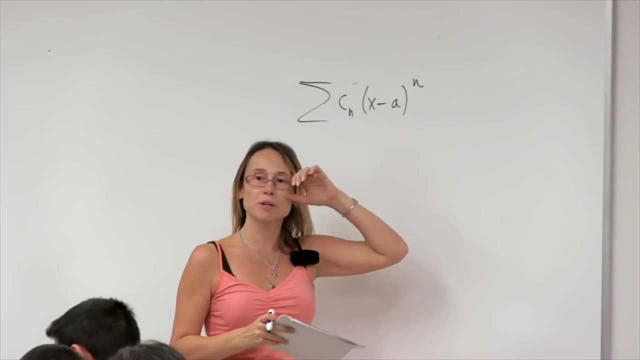 thing. second, no, you see, one half is here, two to the N, and this is two to the N plus one, so one half is hiding here. an extra. the next: I think if it says present as a power series, then it will have to make it in this form, okay, and this is not hard, you see. so 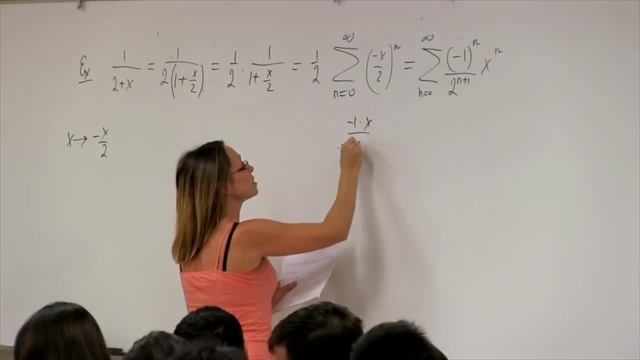 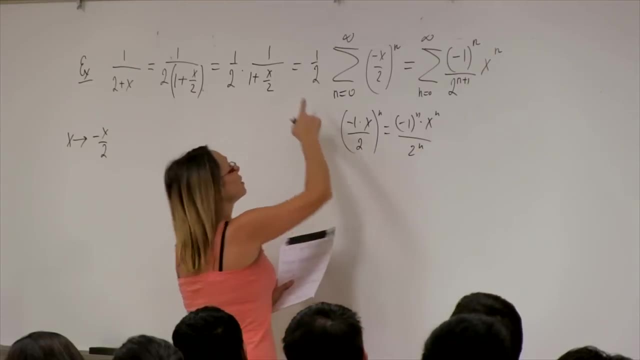 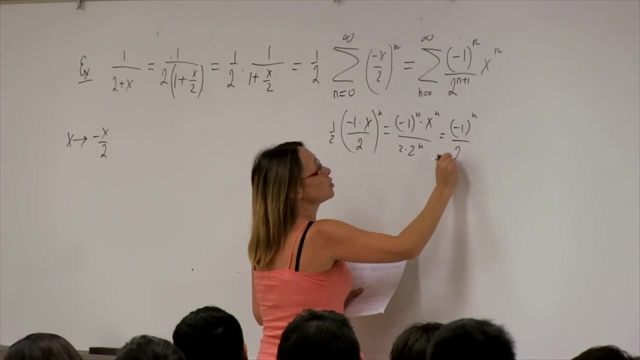 this is nothing but minus one times X, divided by two to the N. so it's minus one to the N, x to the n, two to the N. we have a weight that's going to be integral here, and this is another 2, so I just rewrite it as minus 1 to the n, 2 n plus 1 x to. 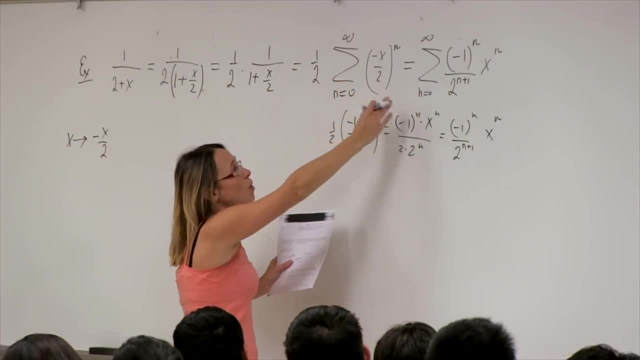 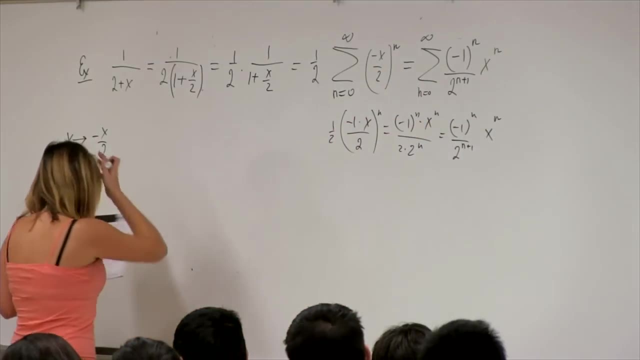 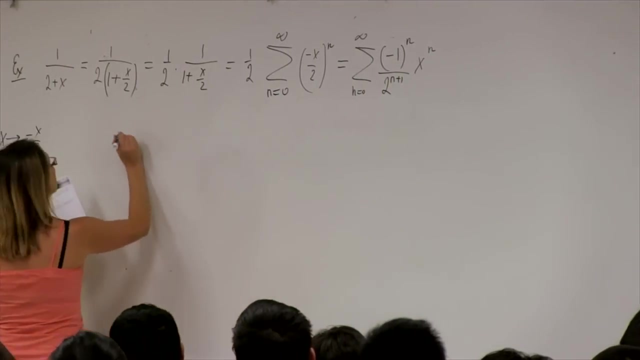 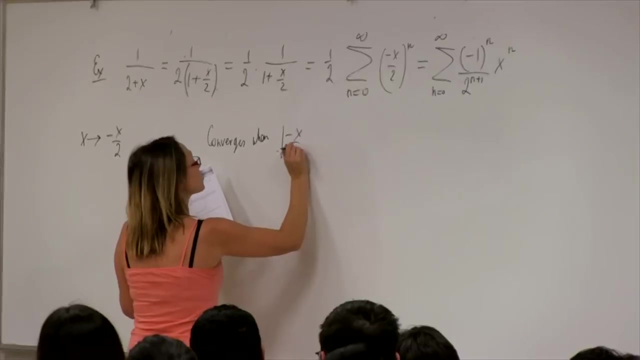 the n. so if I just break it into components and so I want to separate away X from everything else, okay, that's all okay. and what's the radius of convergence? right, so converges when minus X over 2 is less than 1. how do I? 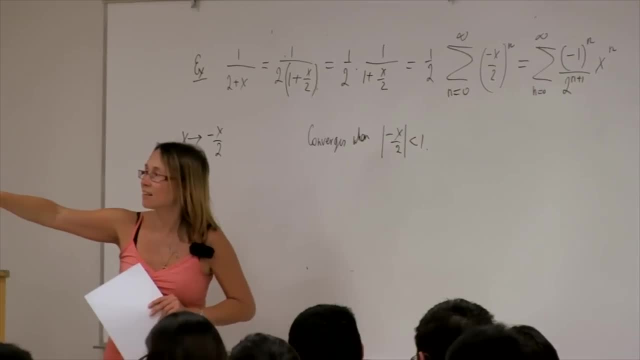 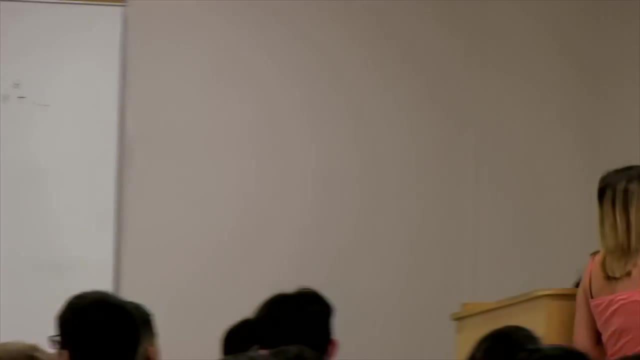 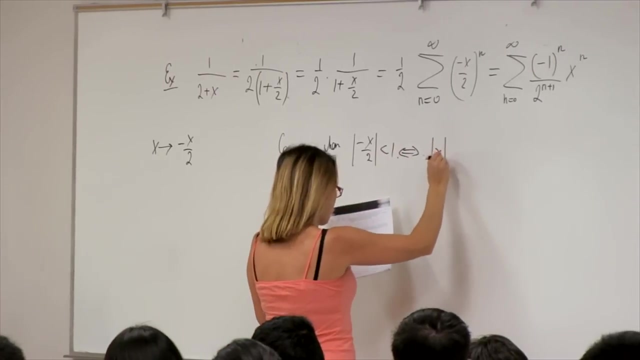 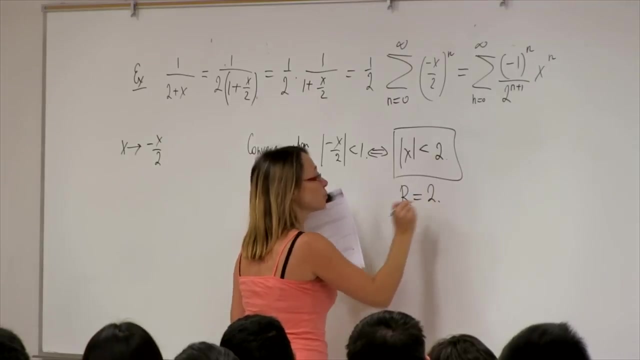 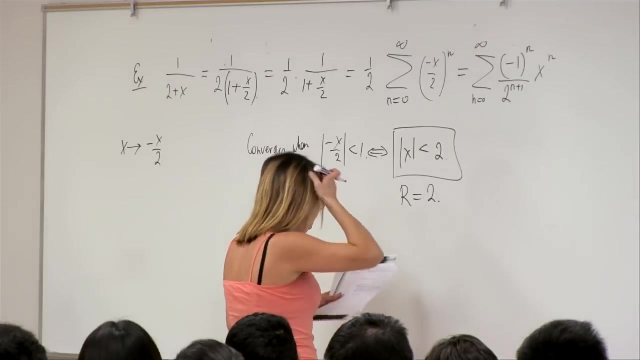 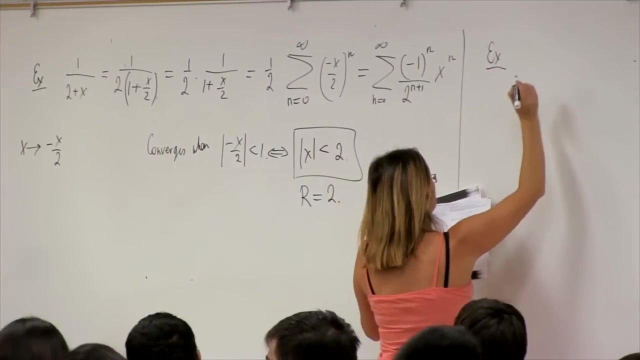 know that the old one converged when X was less than 1. now, instead of X, I take minus X over 2. so this is my new condition and this is equivalent to the absolute value of X being less than 2. so the radius of convergence is 2. okay, one more again. I'm going to bring it back to that old. 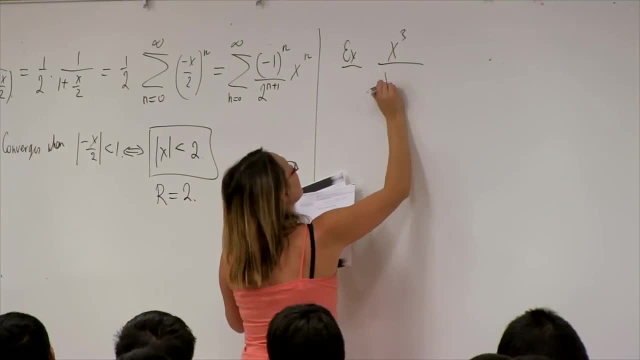 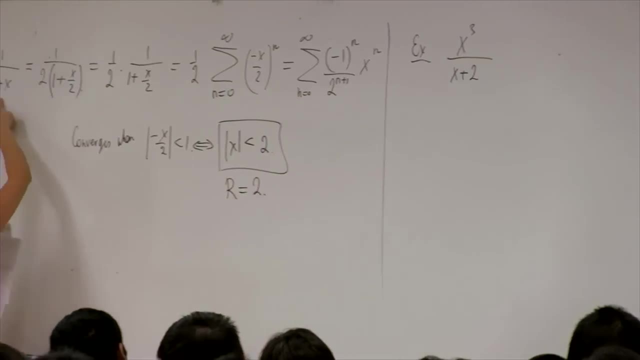 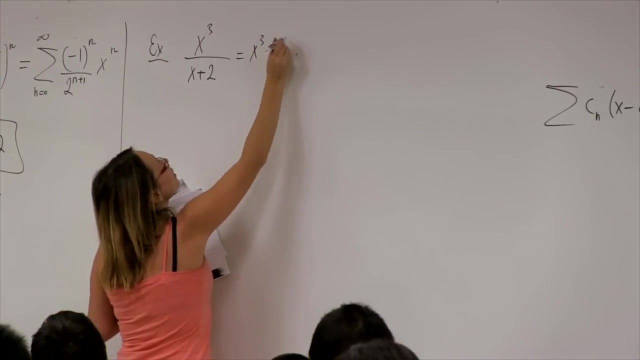 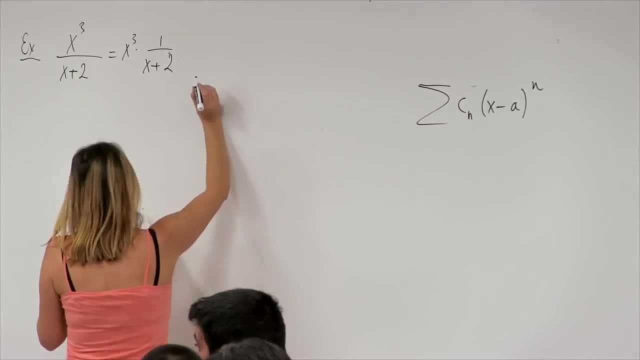 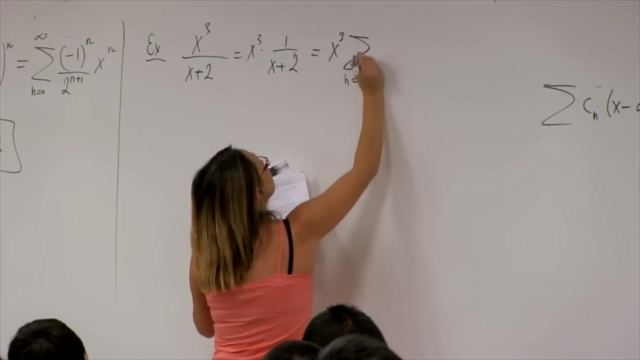 example. so we have X cubed over X plus 2. so, returning to the previously solved problem, I have this component, X plus 2, and it's multiplied by X cubed, so this is X cubed times this, and I already know a power series representation for this, so this is equal to X cubed times this. 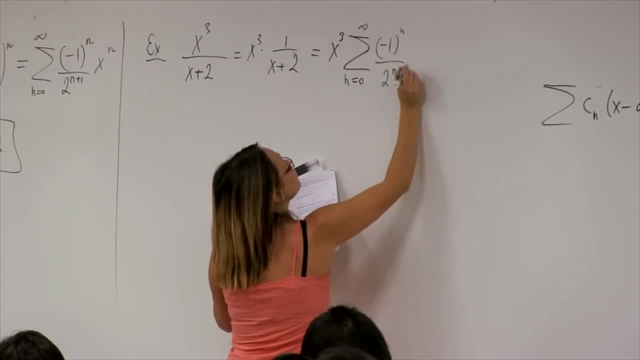 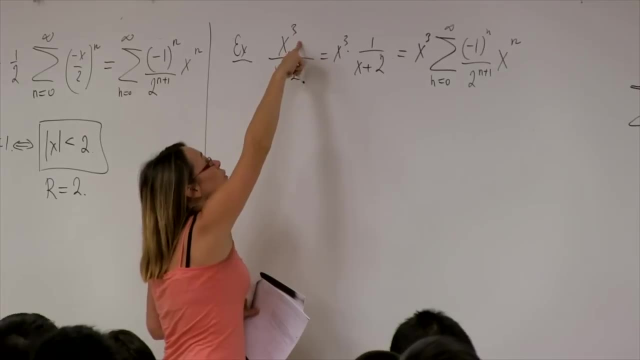 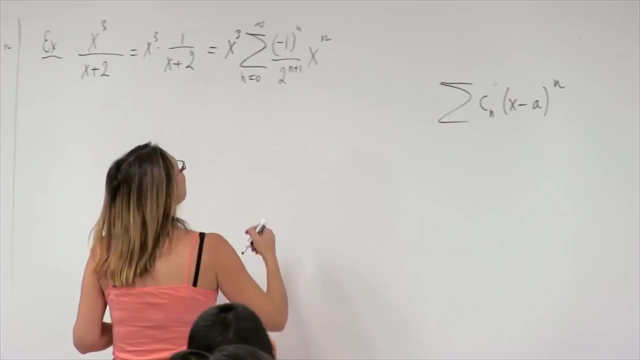 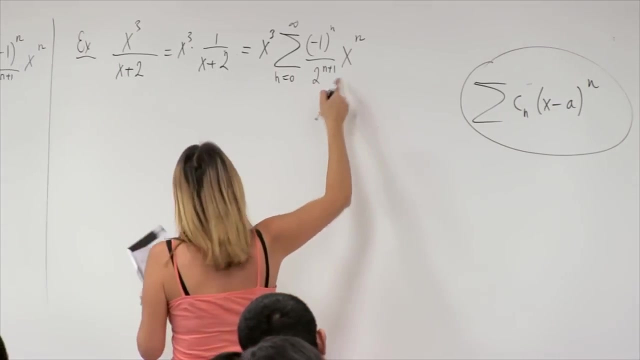 and this is equal to X cubed times this- I just read this off from here- and X cubed multiplies the whole thing. so I keep it okay, and now this is my goal. it has to look like this: okay, so I cannot have X cubed multiplied, so I have to multiply it through. so let me do that. 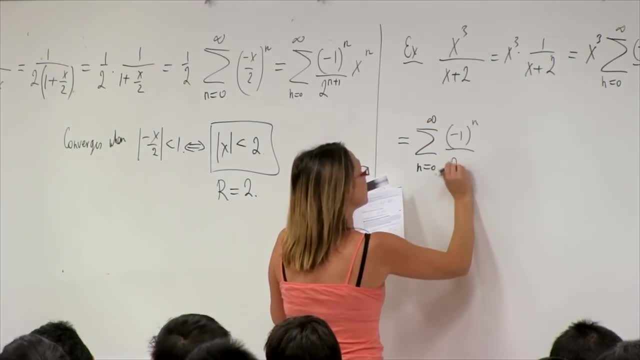 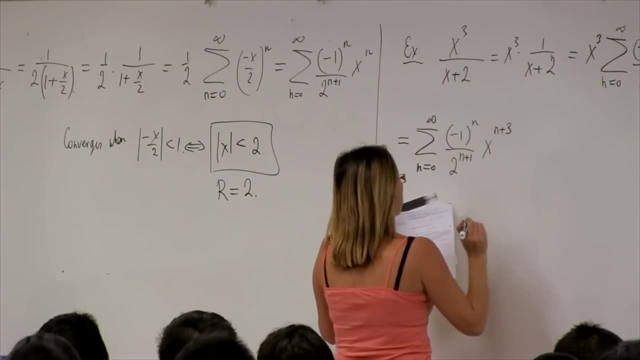 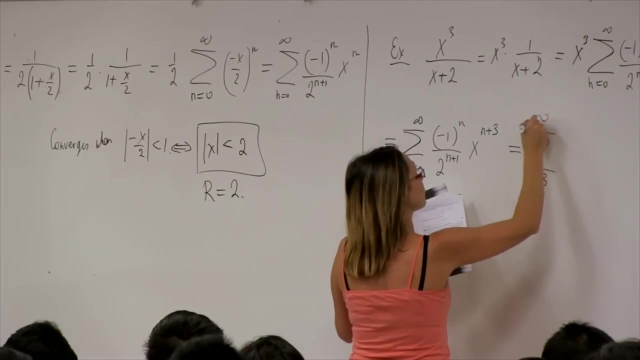 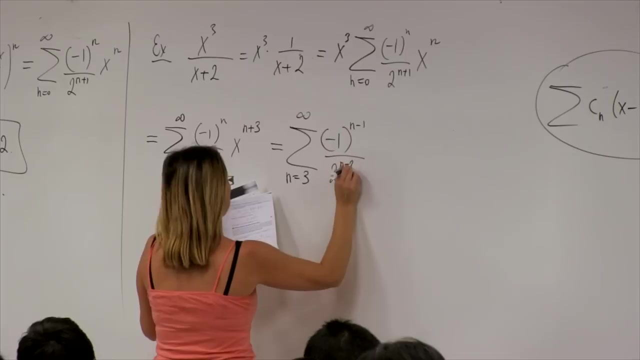 you minus 1 to the n, 2 to the n plus 1, and here I have x to the n plus 3.. And finally, what I can do, I can start enumerating from 3.. I don't know if this operation is necessary. 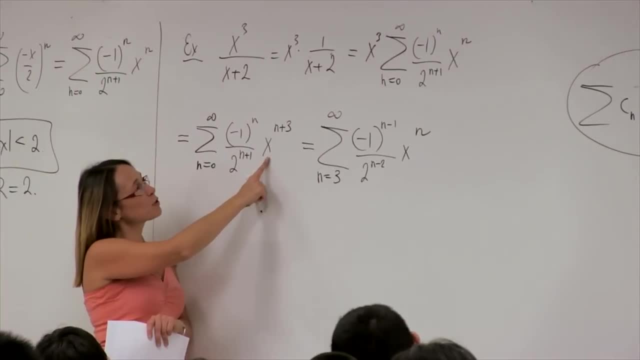 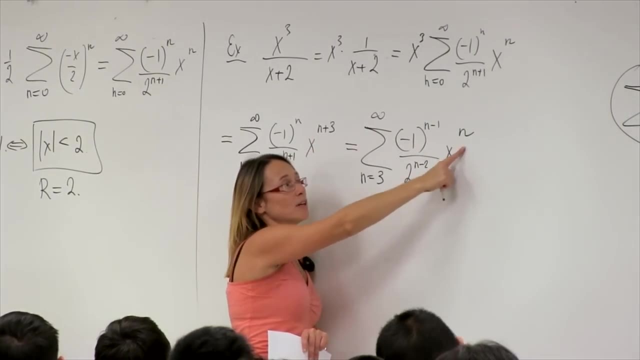 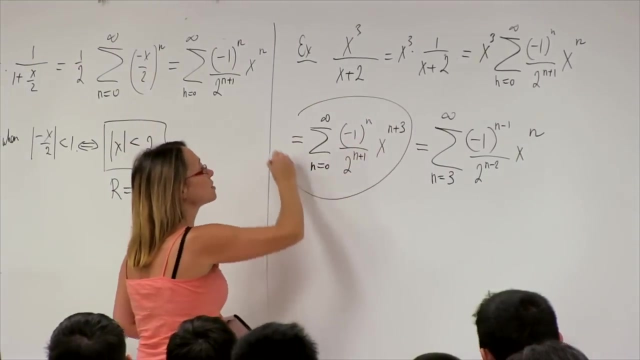 So here I start from: n equals 0, so the first term is x to 3.. Here I start from n equals 3, so the first term is x to the 3.. So these are the same thing, But in principle this would be OK. 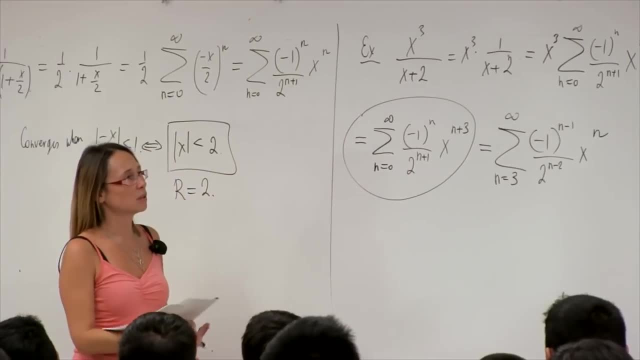 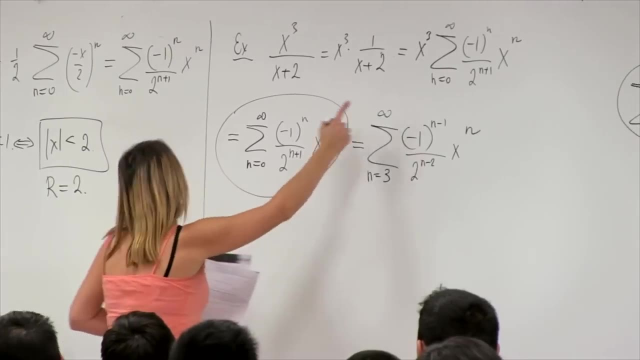 This is enough, So we don't need to? I don't think so. I don't think so. OK, And it has the same interval of convergence, Because it's nothing, but It's nothing, but this power series multiplied by x cubed, which doesn't influence the convergence. 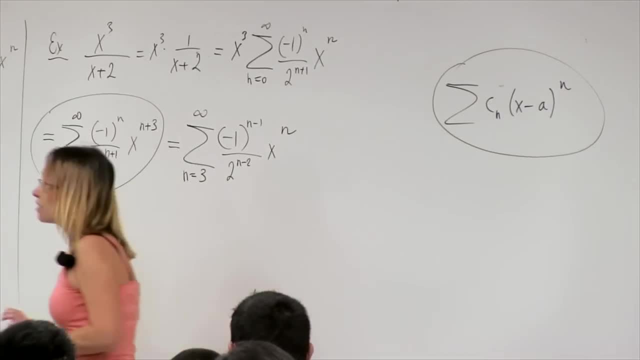 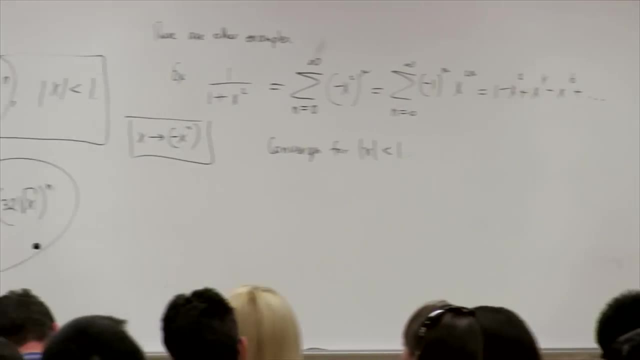 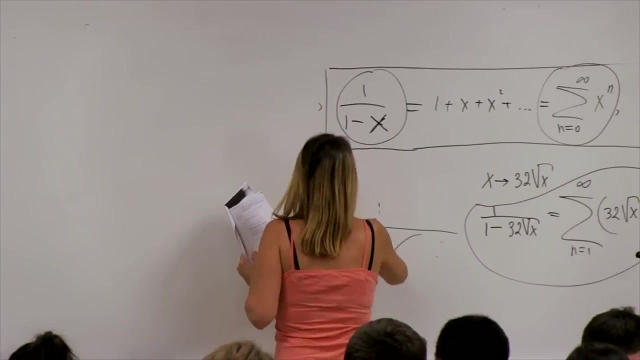 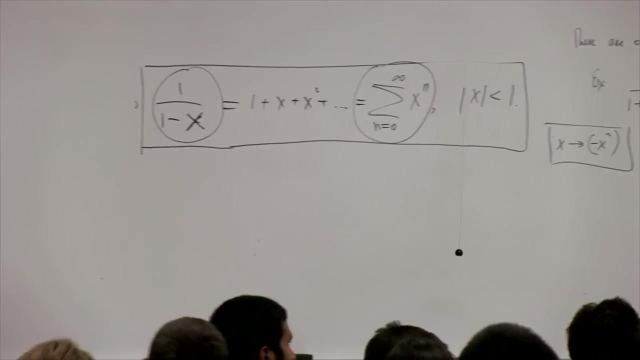 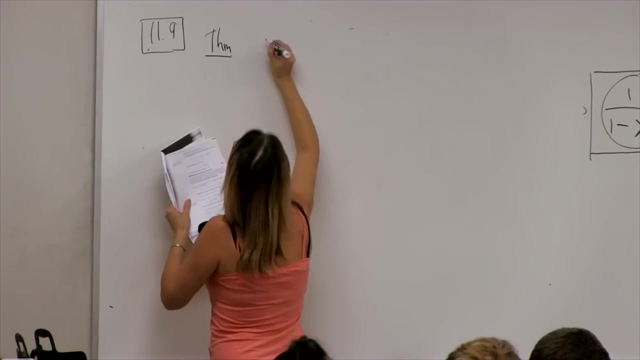 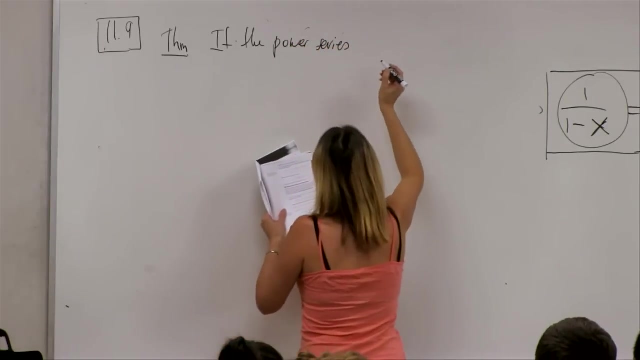 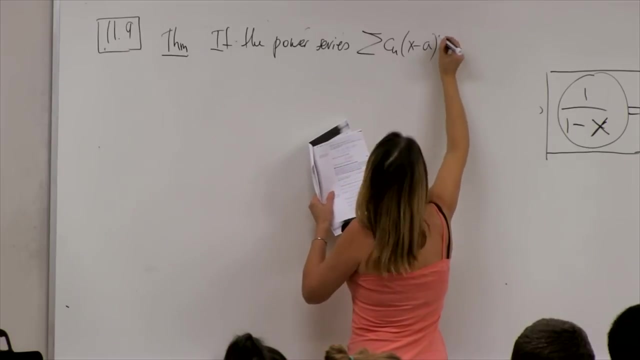 OK, Fine, So there are things that you can do with power series, And let me show you a theorem. Maybe I should keep this OK. So the theorem states the following: If the power series has radius of convergence r greater than 0.. 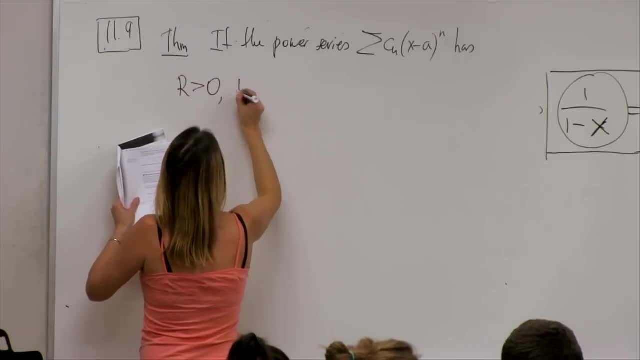 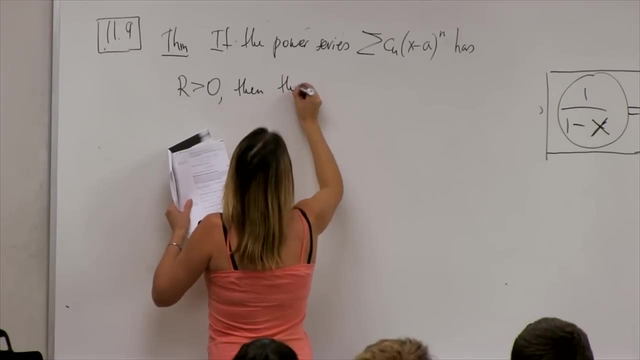 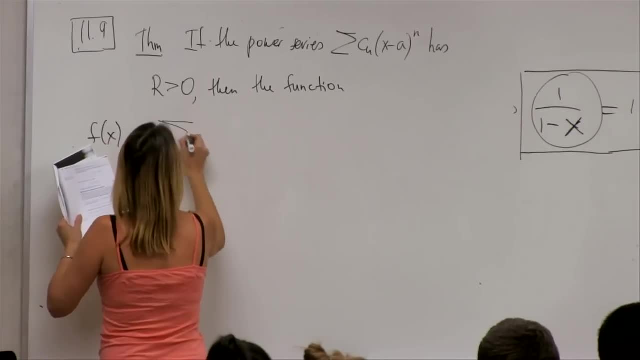 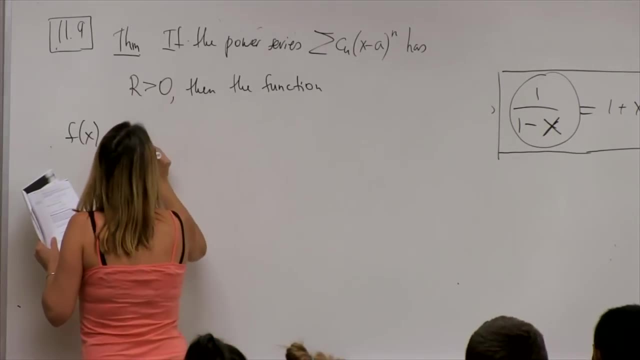 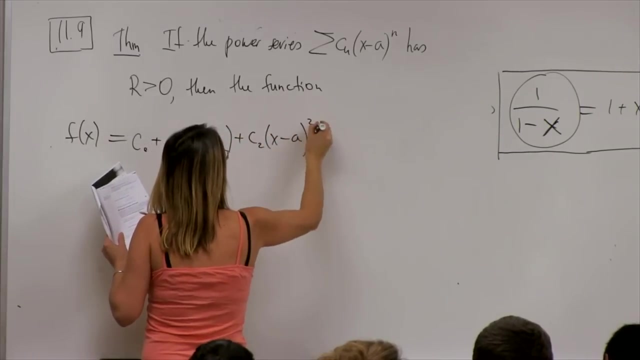 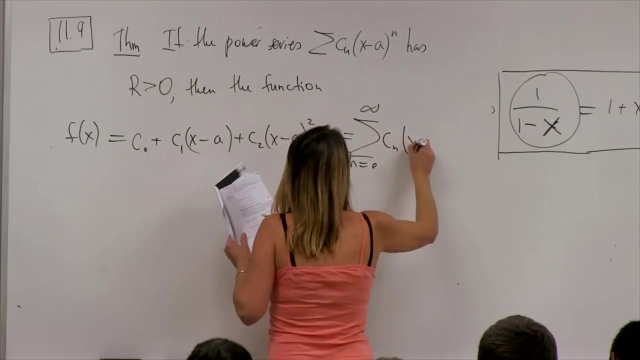 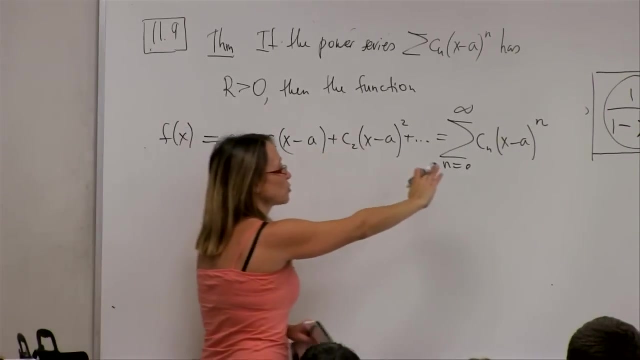 than than F of x defined by the power series. Actually, let me write it down term by term. first, C naught, plus C1 x minus a, plus C2 x minus a. squared, OK, Closed. So you see I'm talking about a function f of x which is equivalent to some power series. 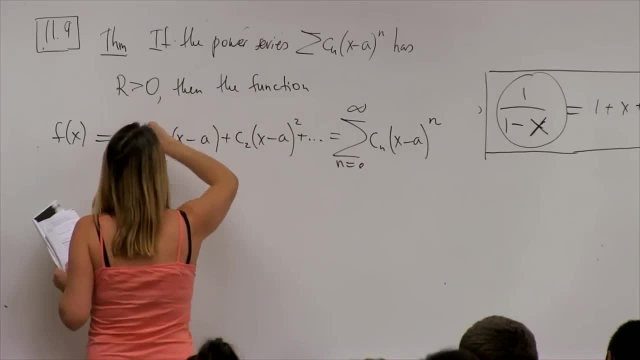 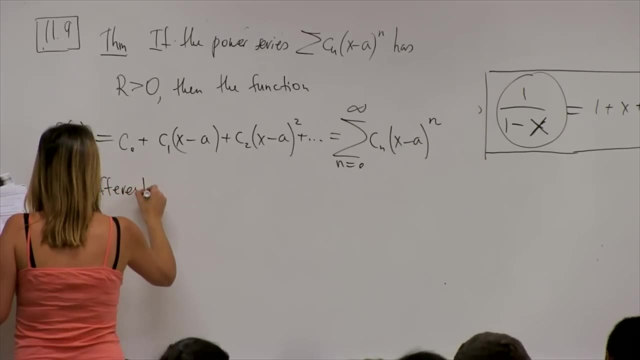 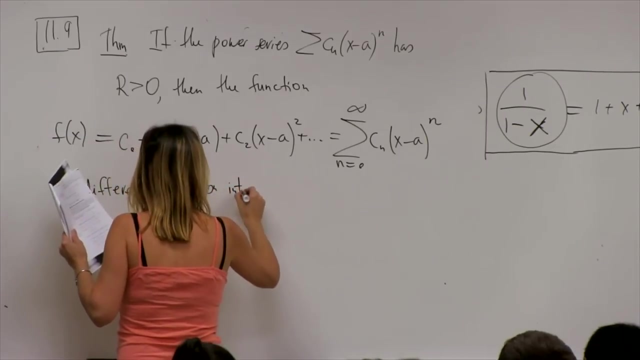 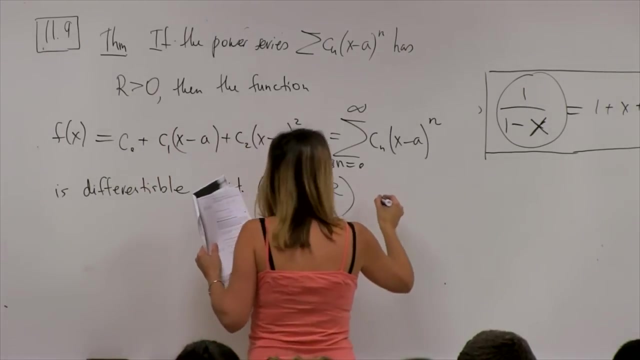 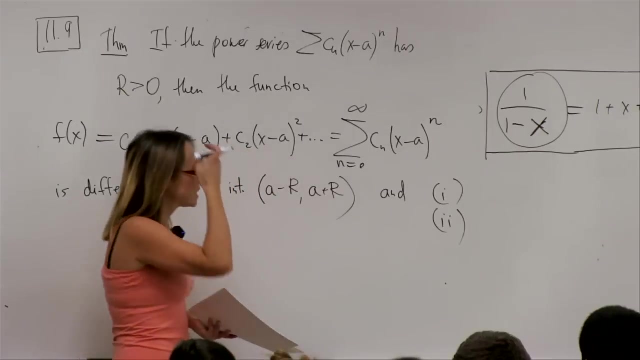 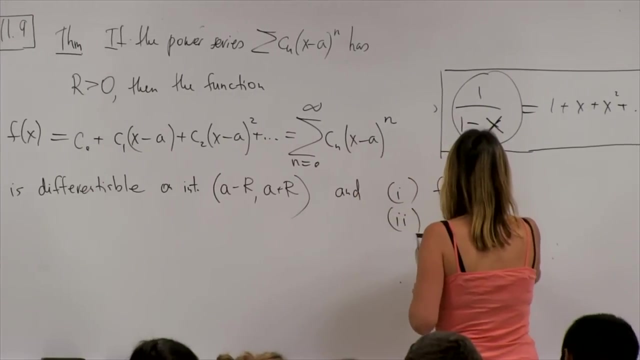 If the power series has a radius of convergence r, then this function is differentiable on interval- a minus r, a plus r, And we have two items which talk about differentiating and integrating this function. So the first result states how we can differentiate this function. 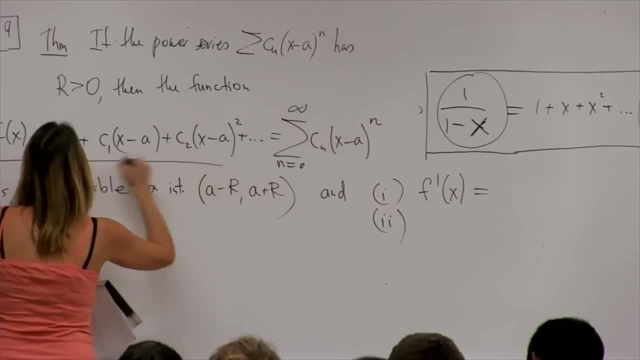 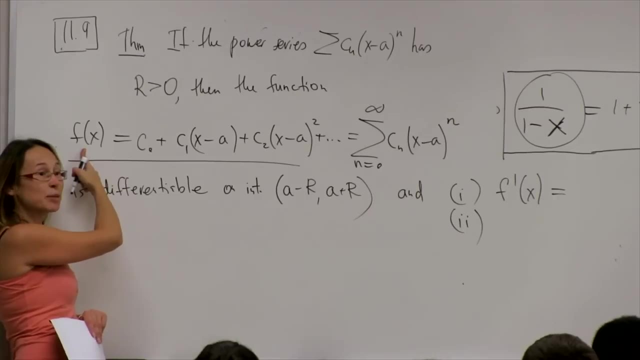 So let's look at this line f of x is c0 plus c1. this, Let's suppose that this is some really horrible function whose derivative you can't remember or don't even know, Some special function, hyperbolic sine, for instance. if you don't know what it is, 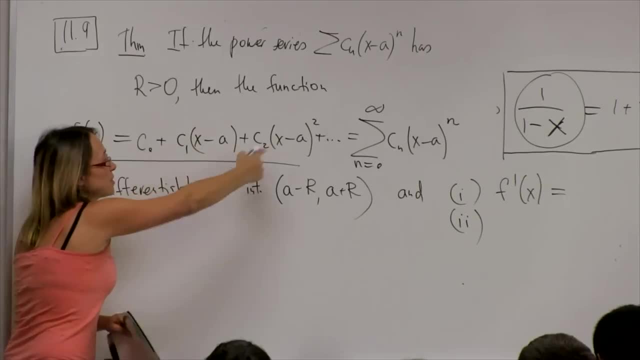 Or there are other functions, And let's suppose you can represent it like this: You don't know how to differentiate the left-hand side, but surely you know how to differentiate any of these. This is a linear function of x. This is quadratic. 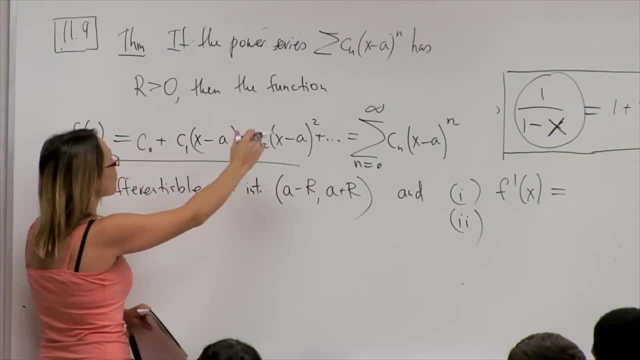 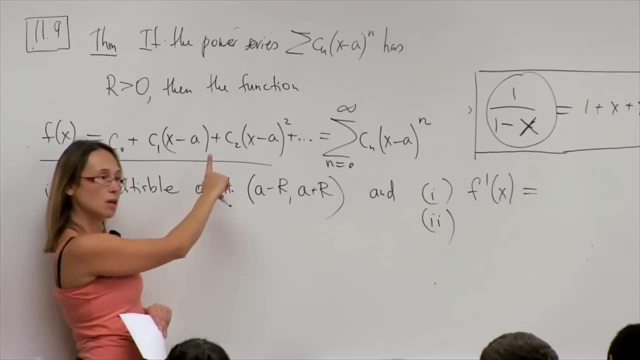 function of X. this is really easy, okay. so what this theorem states is that you can calculate this complicated derivative by simply differentiating each of these terms and each of the derivatives. is very easy. so, for instance, the derivative of the first term is 0, it's a constant. the derivative of the 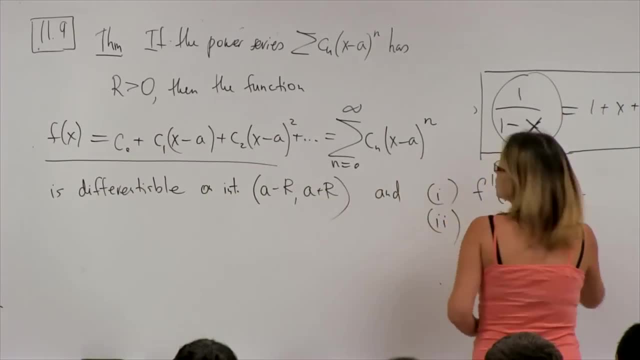 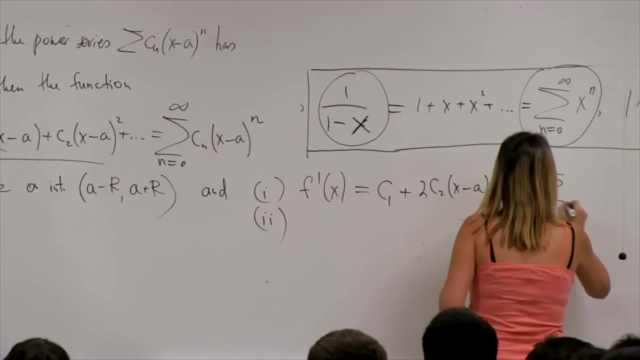 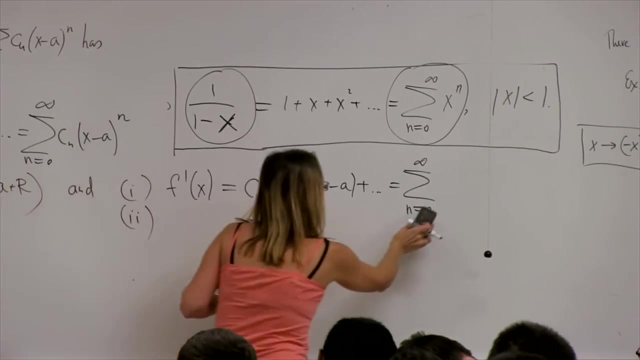 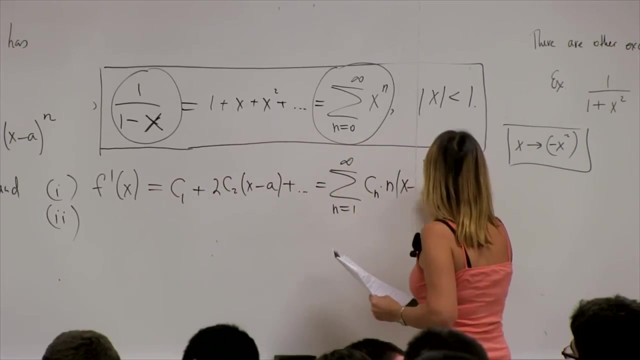 second term is equal to C 1. the derivative of the second term is 2 C, 2 X minus a and so on, and in fact you can write it like this: starting from 1, you have this C n times n X minus a to n minus 1. where does this come from? I go. 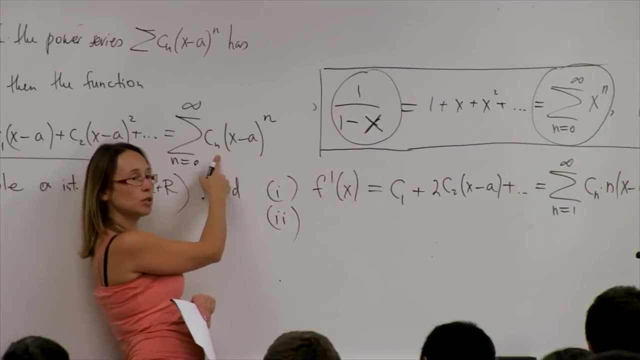 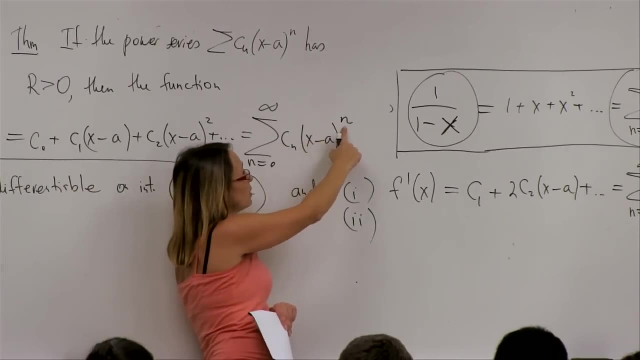 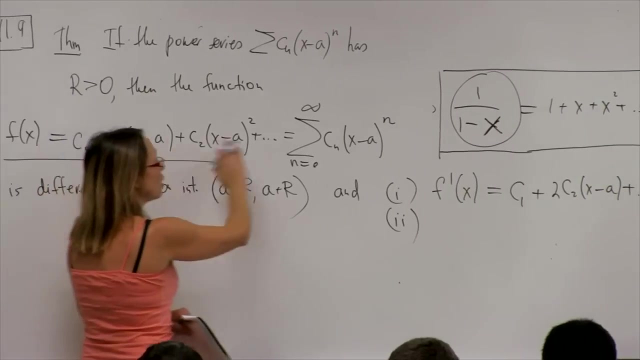 here and I differentiate each term. each term is very easy to differentiate, it's constant C, n. then I have to differentiate this with respect to X, I have n times X minus a. to the power n minus 1. okay, so on the left I have something I don't know how to differentiate. on the right I have a. 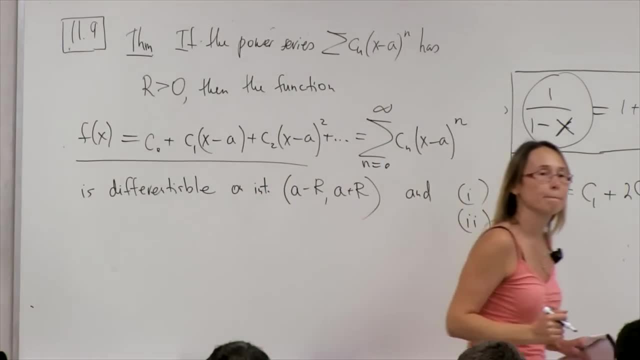 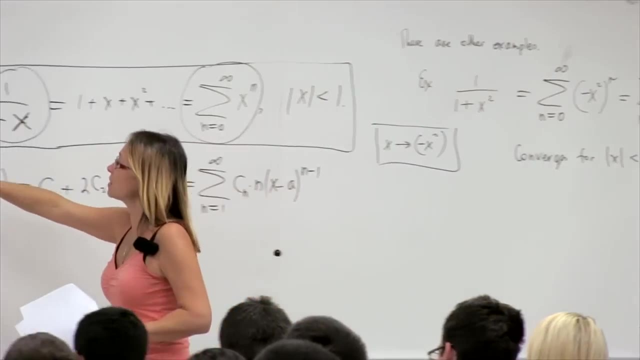 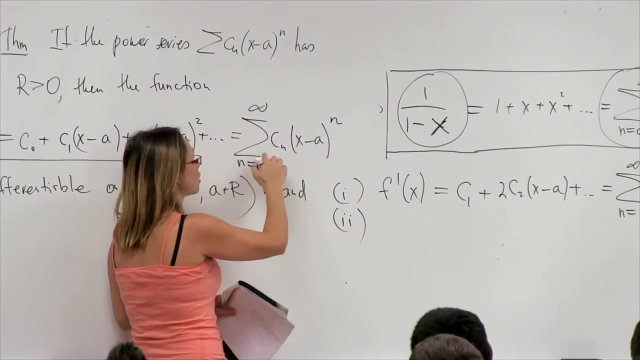 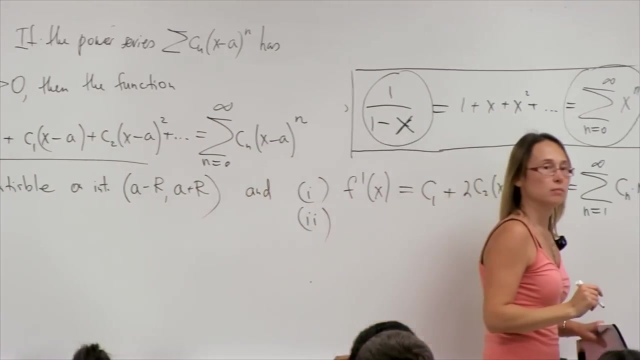 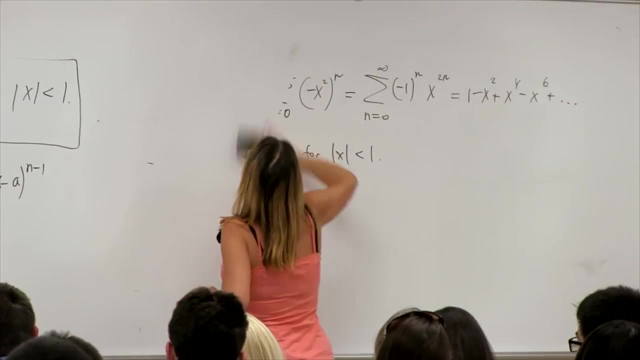 bunch of powers. question: yes, you can differentiate this function inside the sequence. basically, what this means is that you can interchange the operation of differentiation and summation. the derivative of the whole thing is the sum of derivatives of each mem, and I can write it like this. let me show you this is a different way to write it: F prime. 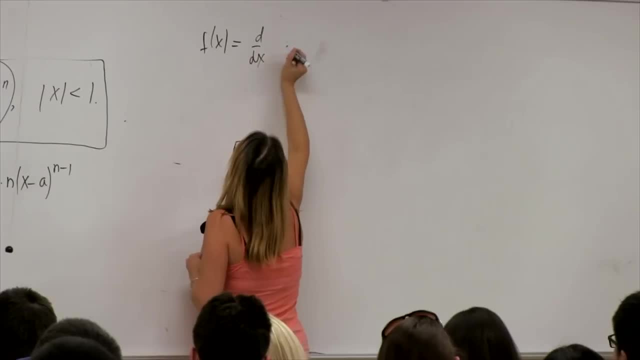 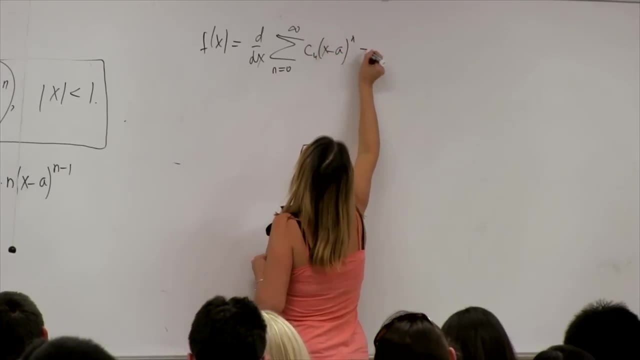 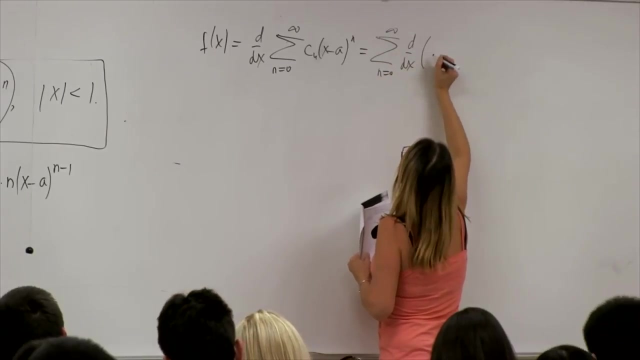 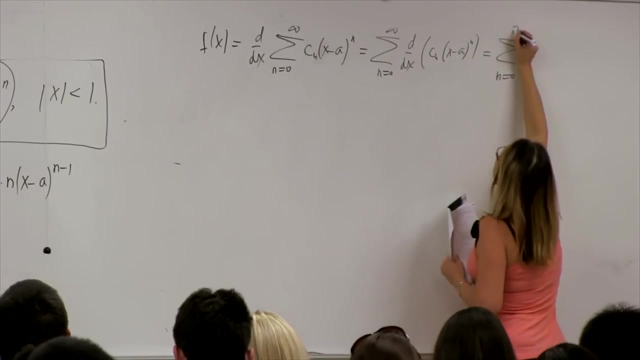 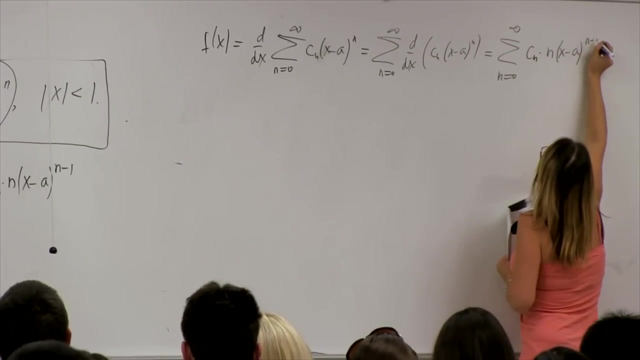 of X. so basically d, D, x of this power series. oh, what I'm doing here is I'm calculating the sum of the derivatives, and these are very simple to calculate. when I differentiate this, I just get cn and x-a to n-1. so instead of 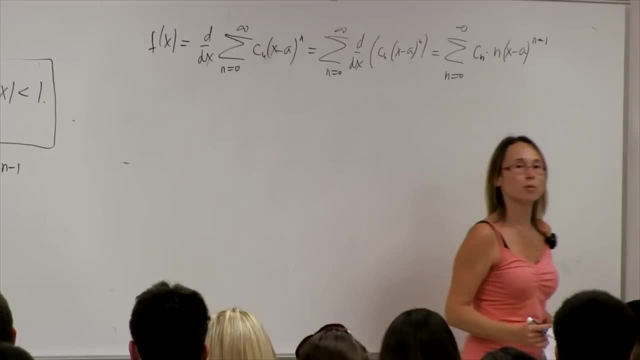 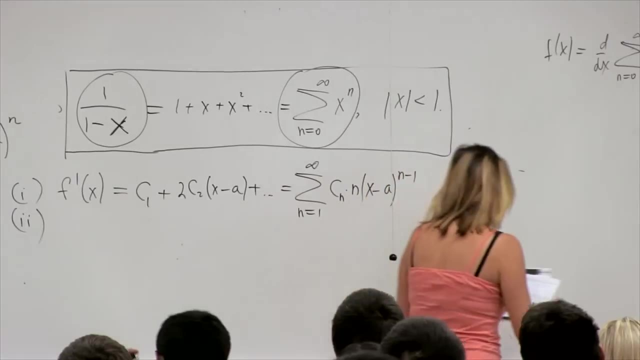 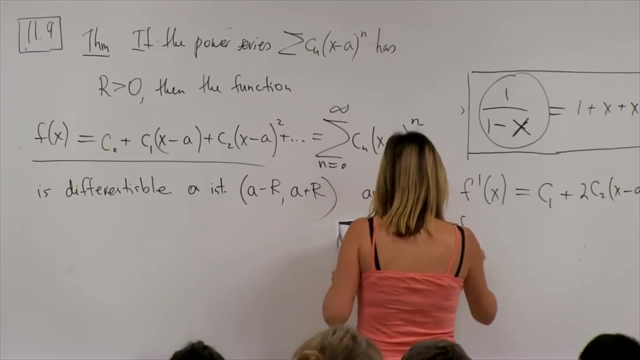 to differentiate the whole thing. I differentiate each term and then I add them up. that's what this first part of the theorem states. the second part deals with the opposite operation, which is integration, or taking the antiderivative. so what's the antiderivative of f over x, dx? 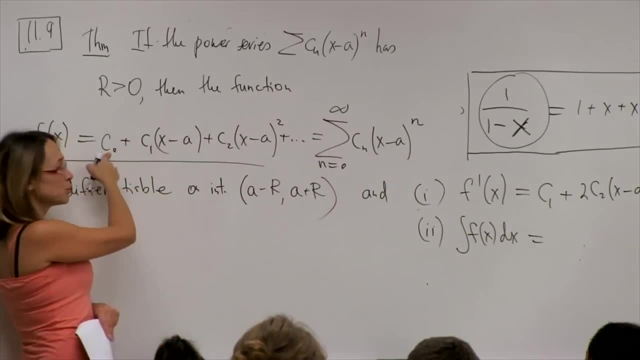 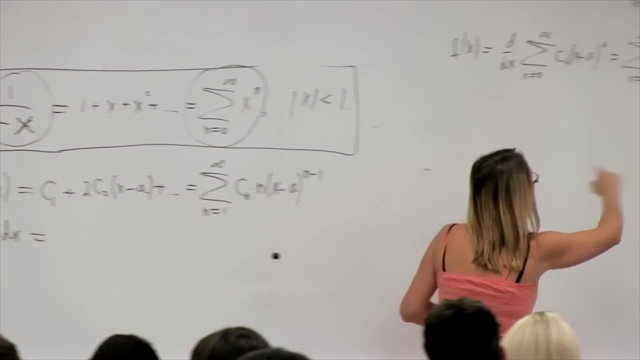 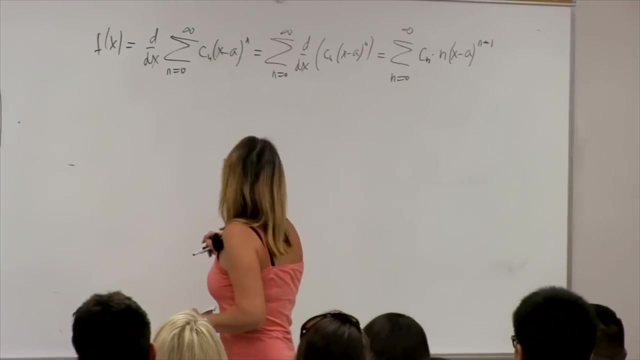 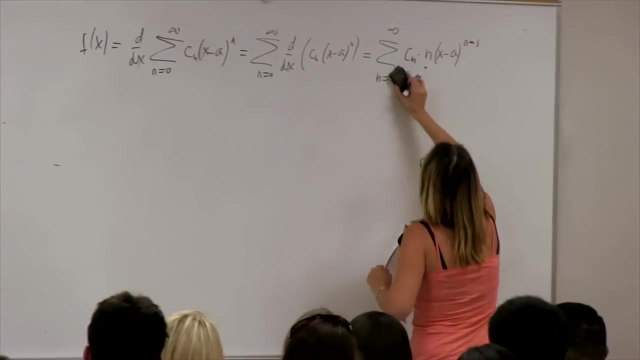 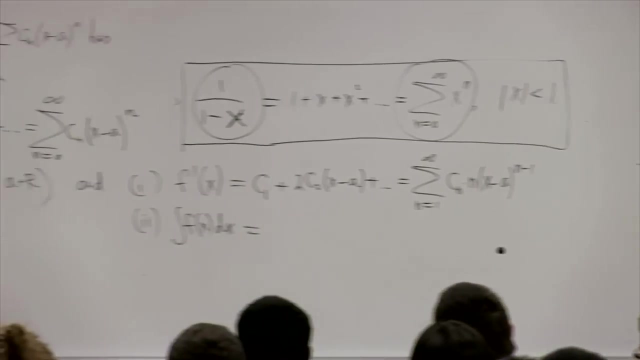 the same thing, so I have to take the antiderivative of each term question. oh so yes, for the first term. yeah, you're right, I should start with 1, because the first term is a constant. the term corresponding to n equals 0 is a constant. 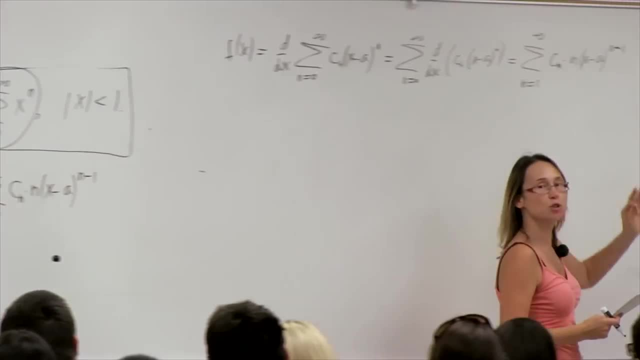 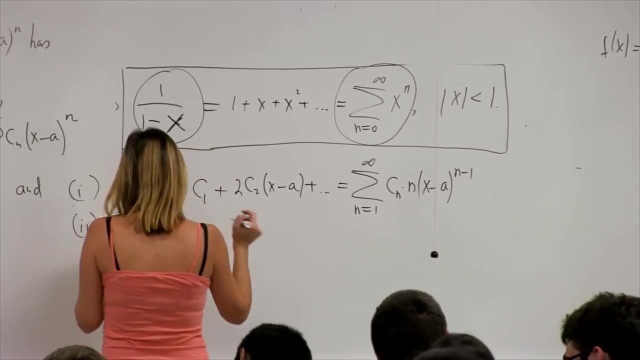 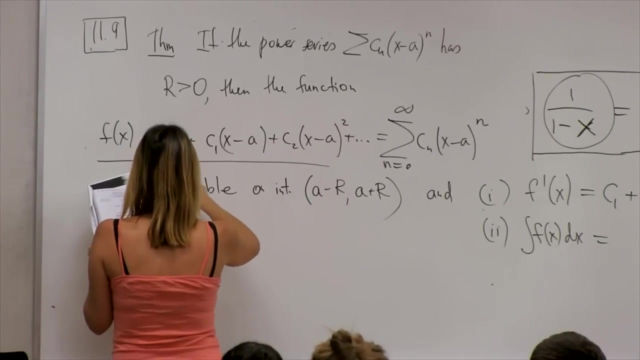 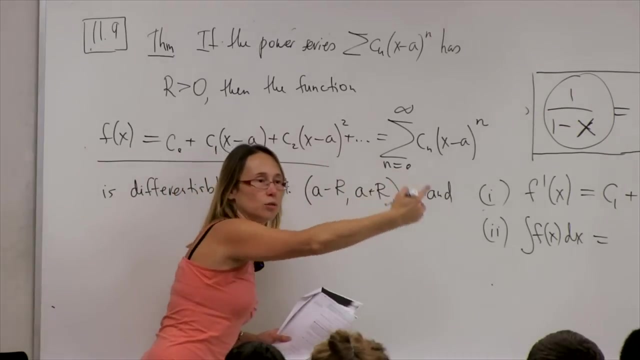 so it doesn't even show up here. its contribution is 0. so so, with integration, what do I have? the first term gives me a linear function, this will give me a quadratic function, this gives me a cubic function, and so on. ok, I can just take the antiderivatives. 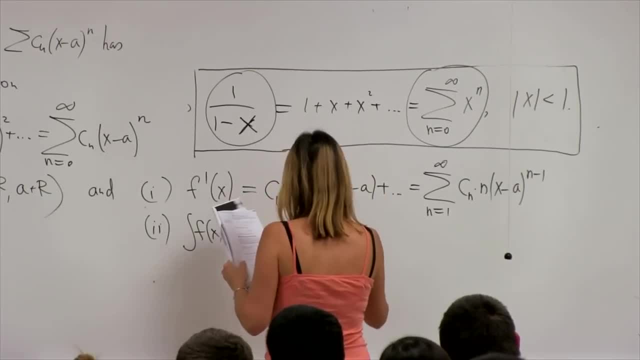 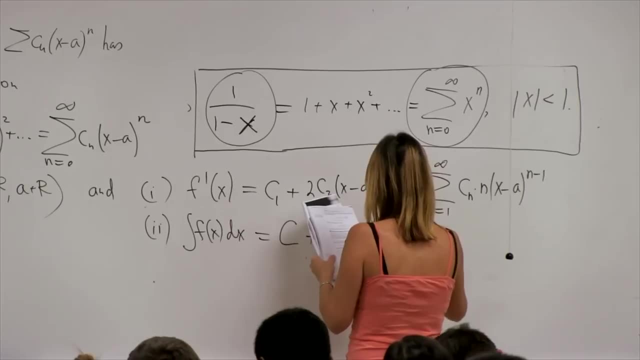 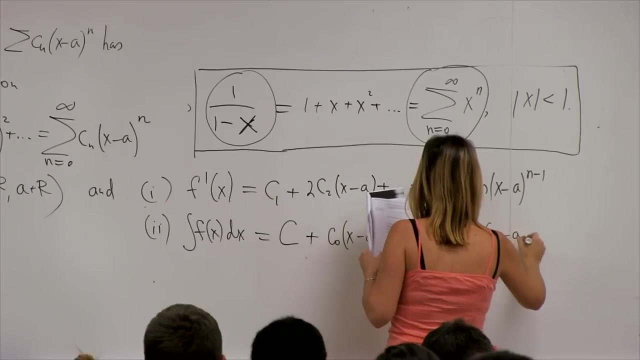 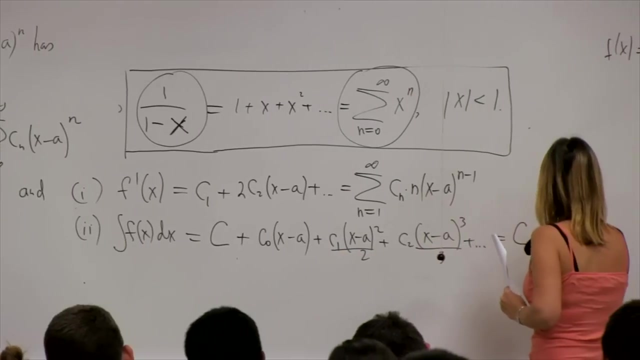 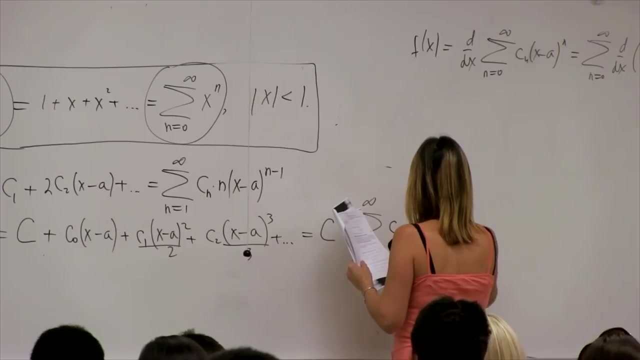 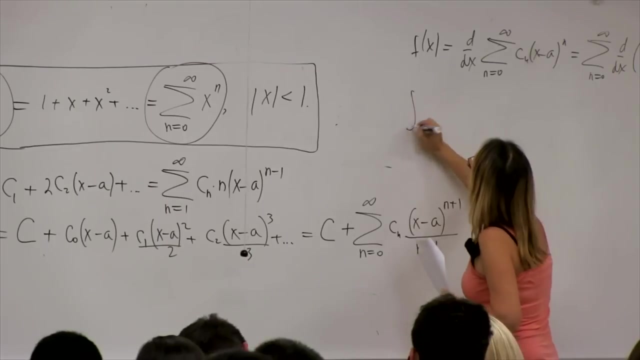 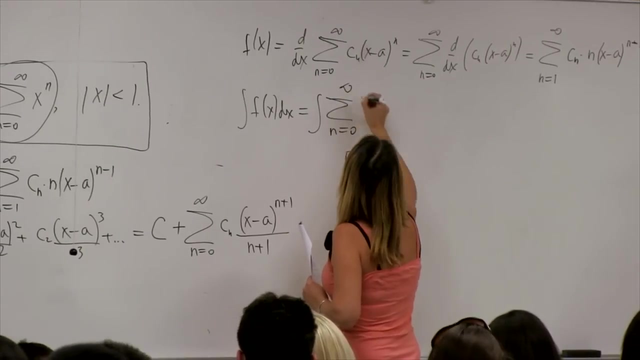 and I will have a constant of integration, c. so I'm going to write it like this, or more concisely: I have a constant c plus an infinite number of terms- c, n, x minus a, n plus 1, n plus 1- and here I have the following operation: 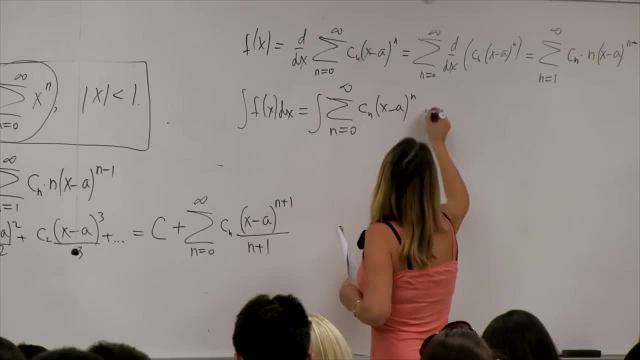 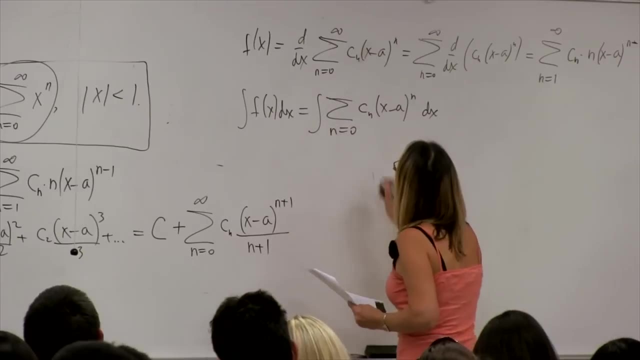 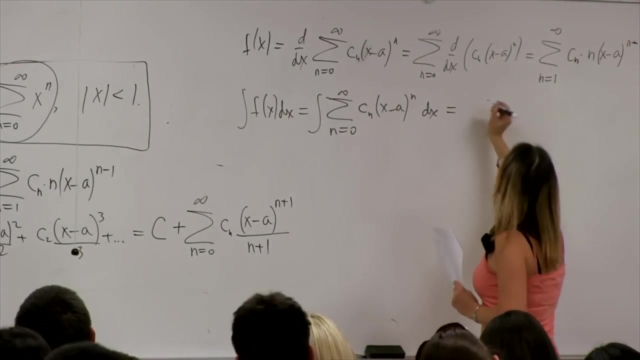 so, basically, I'm taking the infinite series and I need to integrate it. what I'm going to do as the next step? I'm interchanging the sign of integration and the sign of summation, so I have the sum of little integrals of the integral of each term. 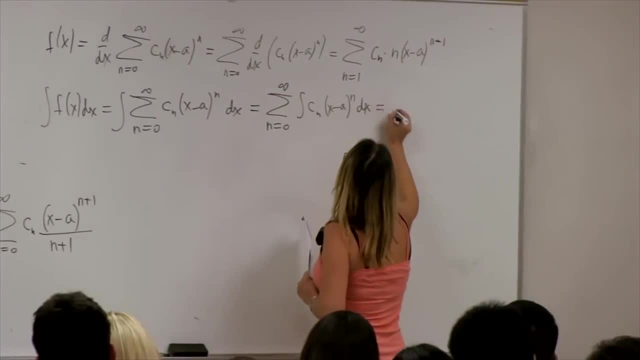 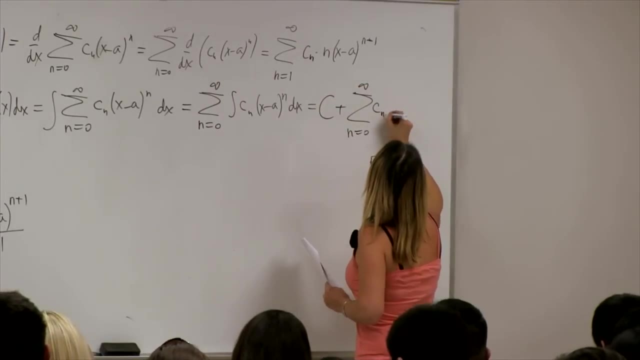 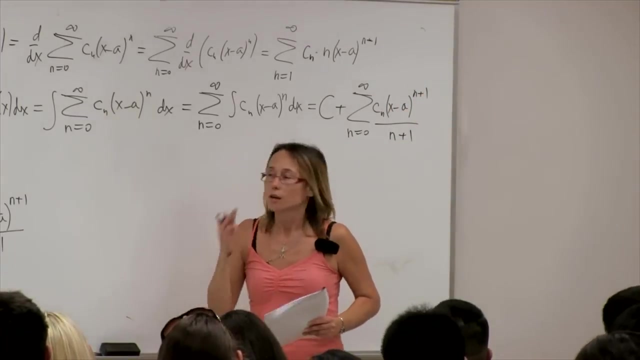 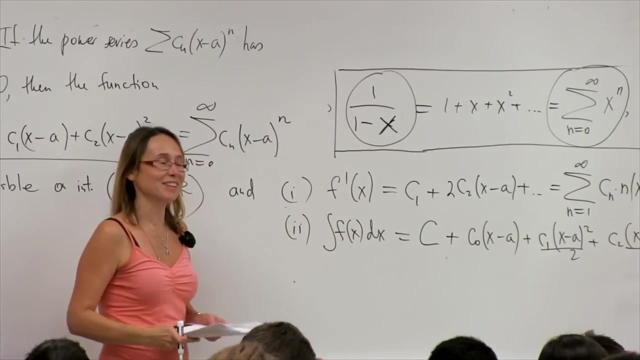 and then I can write it like this: these are the antiderivatives of each term. and again, ok, I know how to differentiate many functions. integration is a lot worse. most functions we don't know how to integrate. however, if I know how to represent my function, 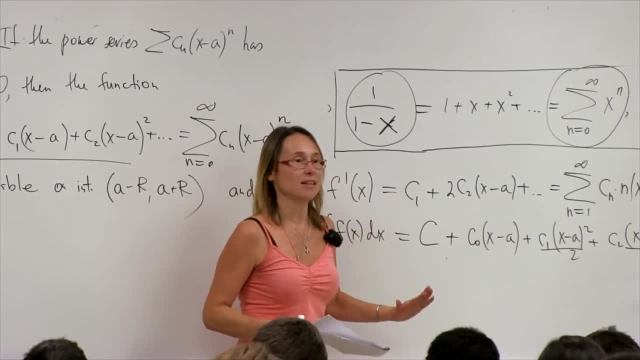 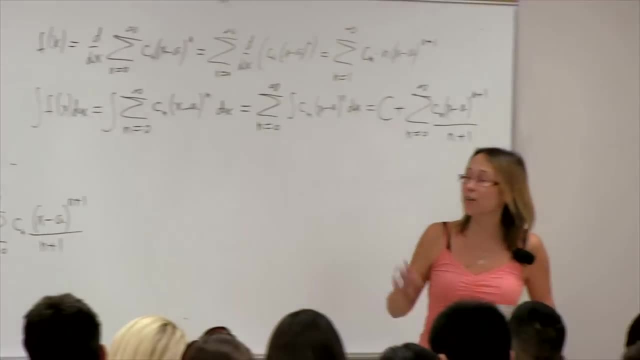 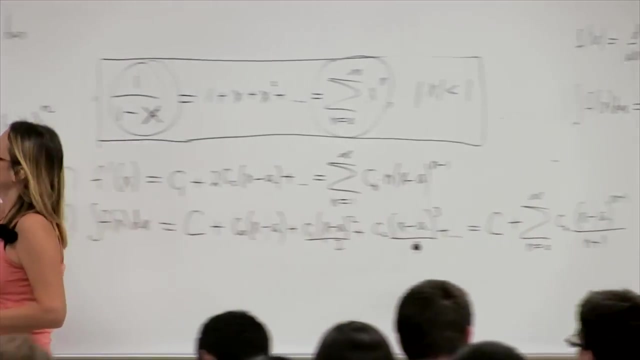 as a power series, I can integrate anything, because of course I can always integrate these power functions right. so this is a very powerful tool. as long as you know how to represent your given function as a series, then you can differentiate and integrate it, but only inside the radius of integration. 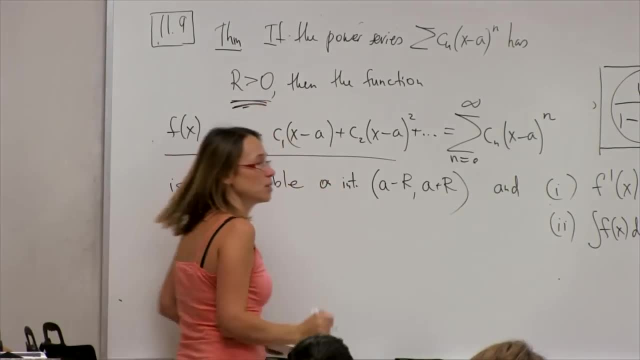 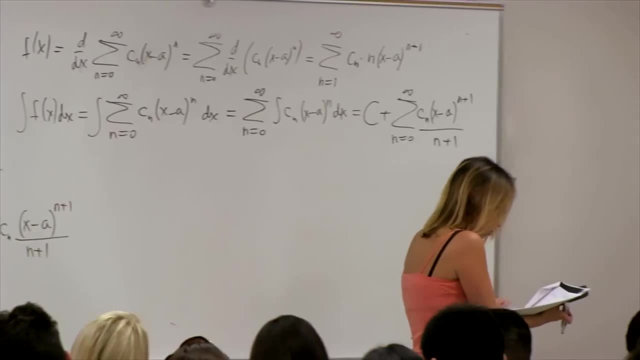 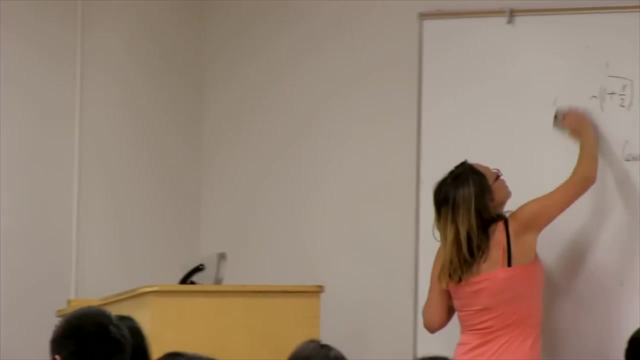 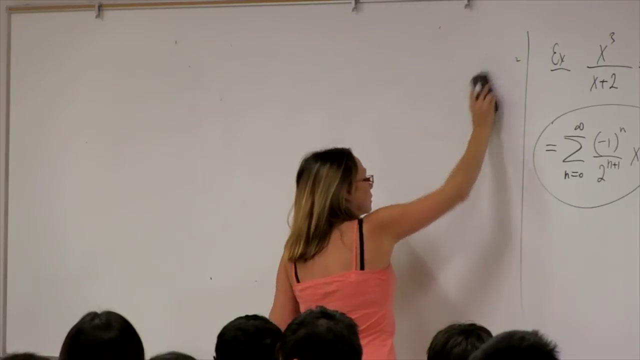 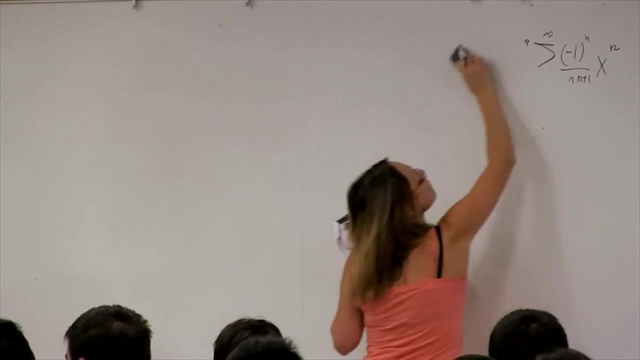 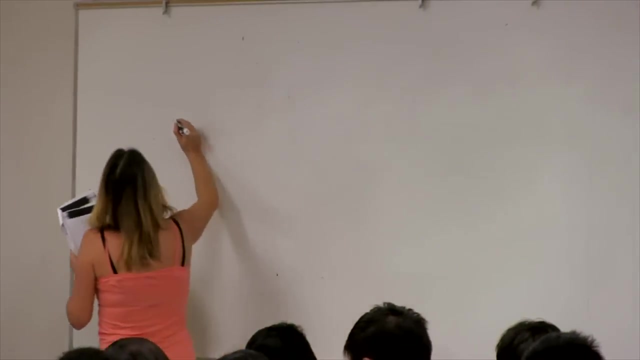 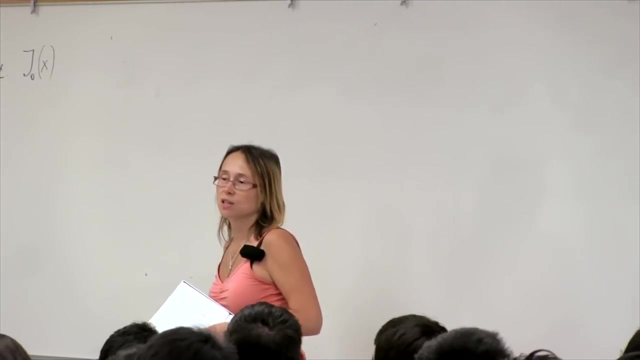 I'm sorry, only inside the radius of convergence. outside the radius of convergence, none of this works. so let me show you some examples. so the first example: remember the Bessel function, the shape of a hanging rope right. this is a special function and I drew you a picture of that function. 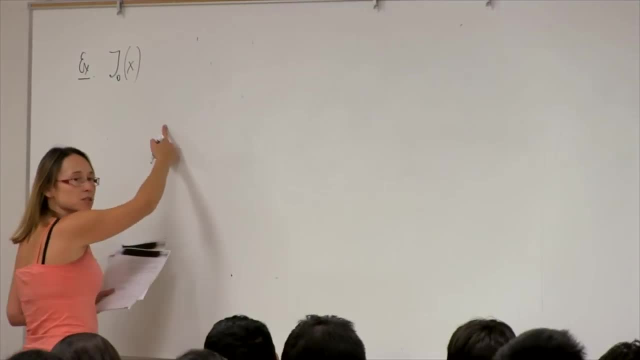 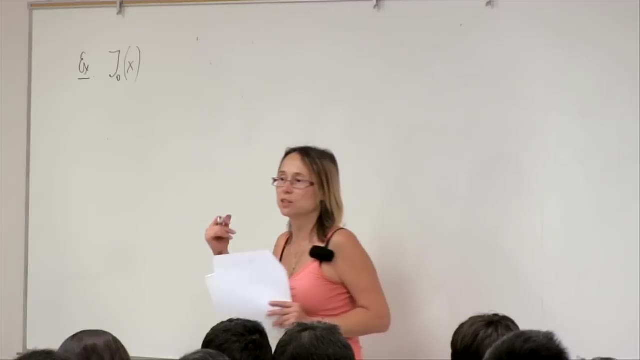 but of course we don't know what the derivative of that thing is. it's not like sine or cosine that are tabulated. we know everything about them. this is a more complex function and it's not clear how to differentiate it, but I know its power series representation. 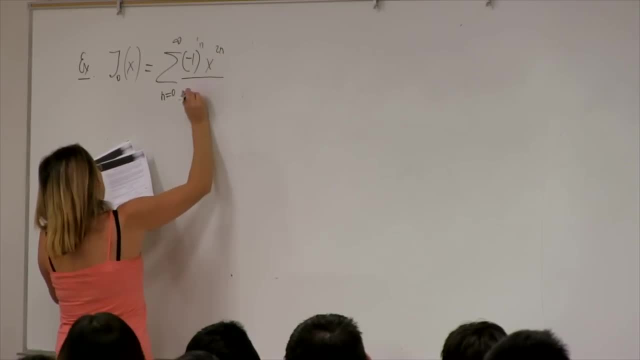 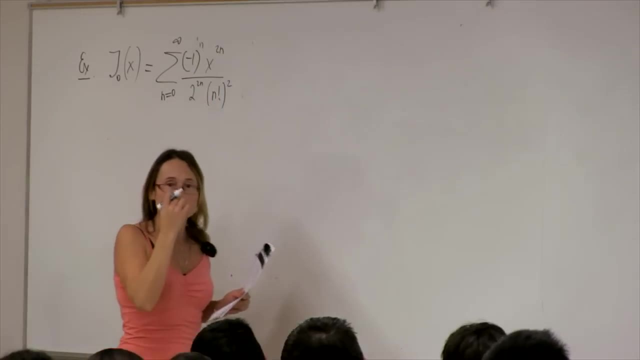 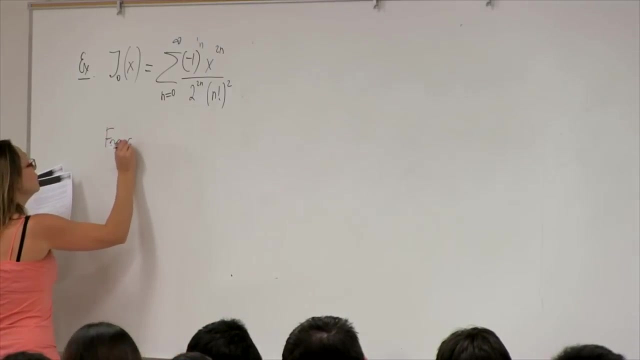 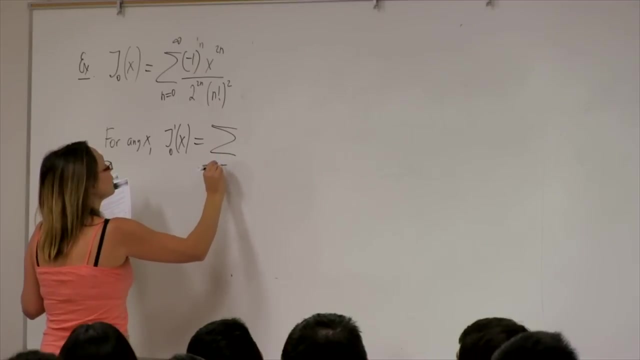 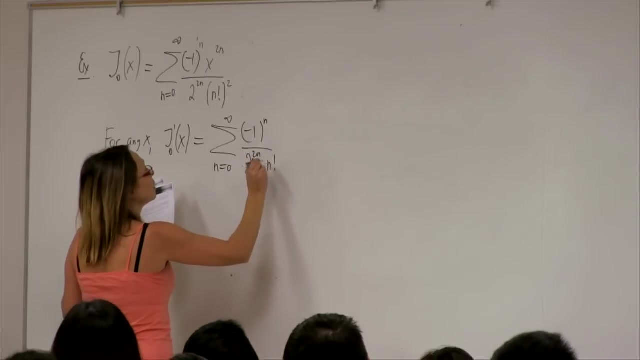 it's given by this and that gives me an ability to calculate its derivative. the radius of convergence is infinite, so for any x we can calculate the derivative by simply calculating the derivative of each of these terms. so constants stay exactly as they are as far as x is concerned, all of these are constants. 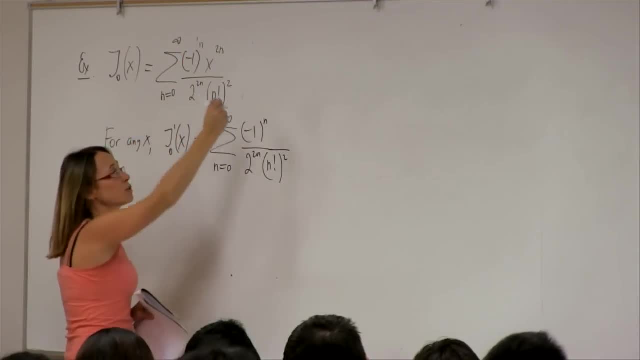 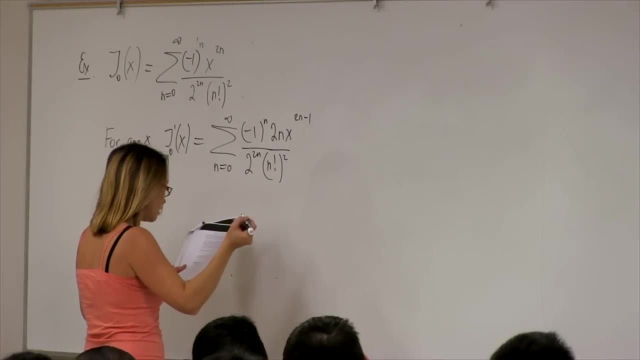 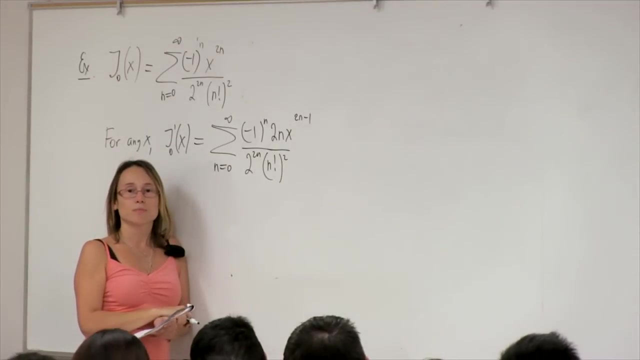 so we just need to differentiate x to the 2n. what's the derivative of that? it's 2n, x to 2n-1. very simple and that's it. there's nothing. so if I can add this up, I get the derivative. 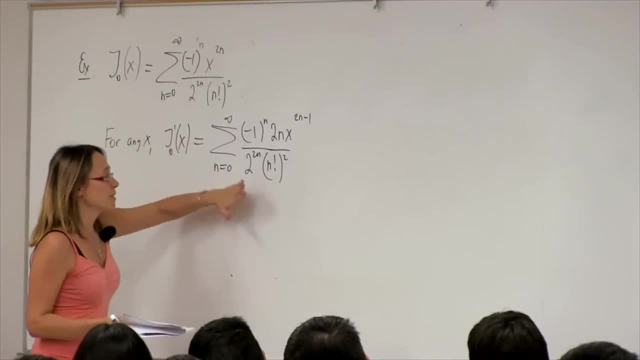 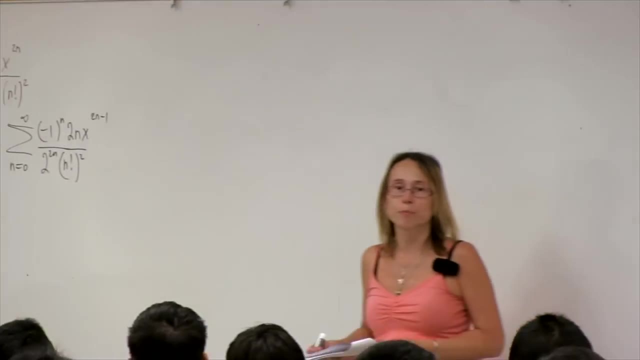 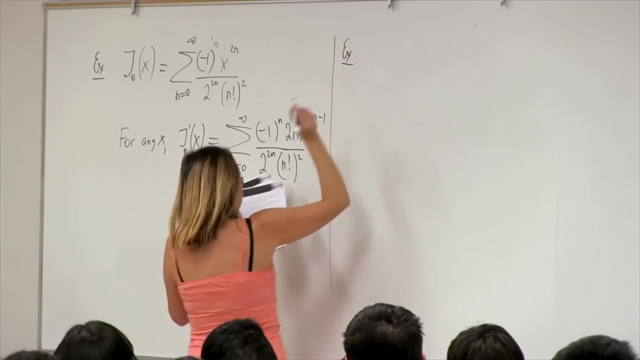 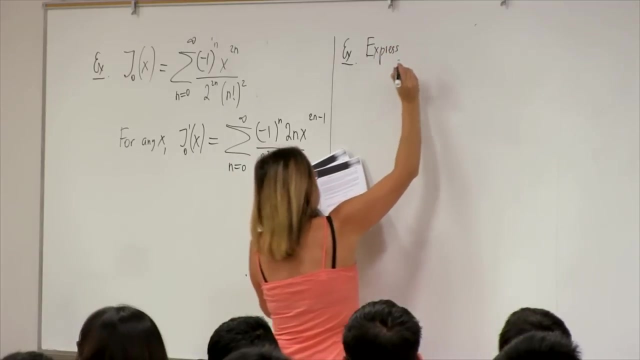 so this is an example of a function that we don't know how to differentiate, but our ability to represent it as a power series allows us to differentiate it, and we can integrate it too. it's just as simple. the next example is more creative, so express this function. 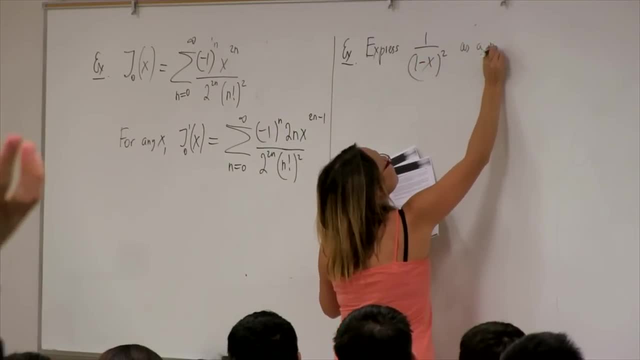 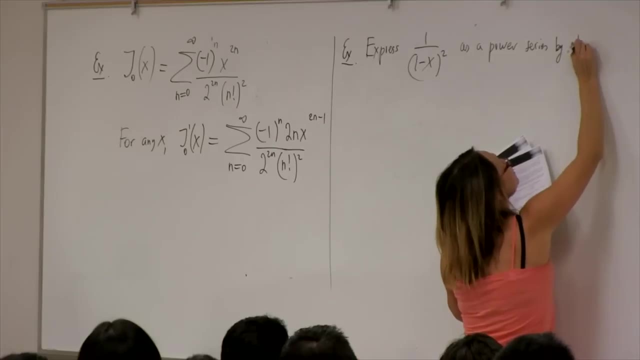 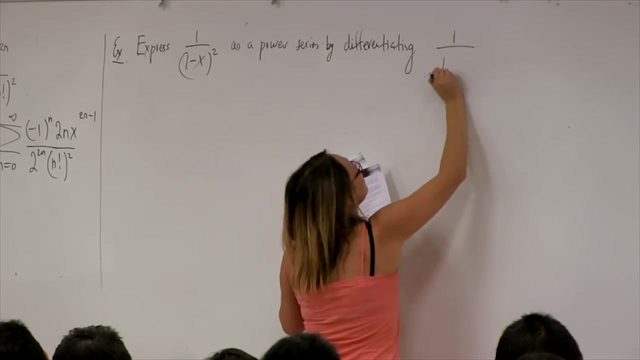 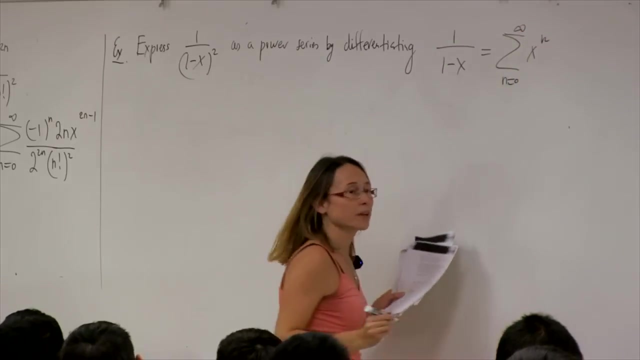 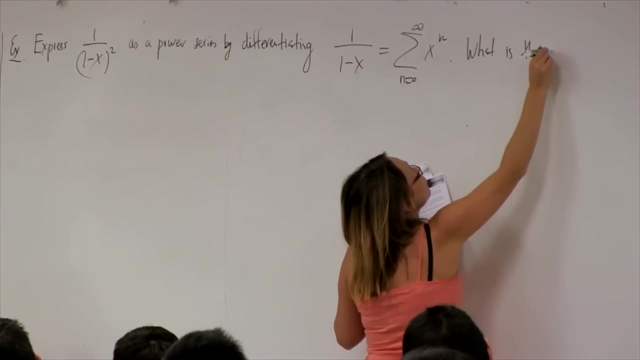 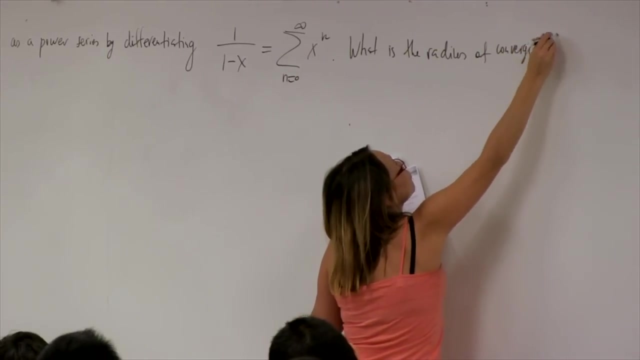 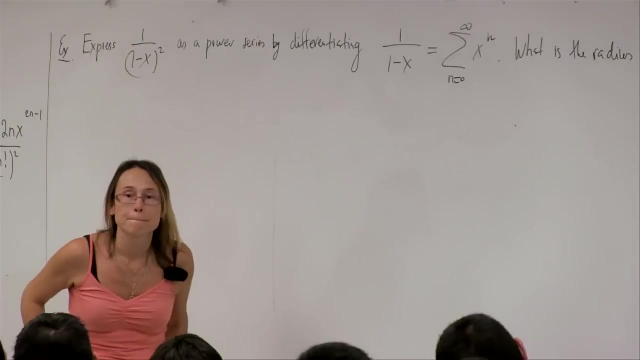 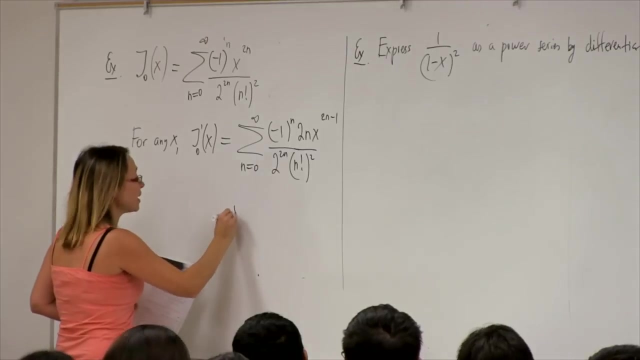 as a power series by differentiating our important equation. okay, what is the radius of convergence? so we are going to deal with this function question. for the second part of the question here, yes, why is it 2n-1?? so if you have x, 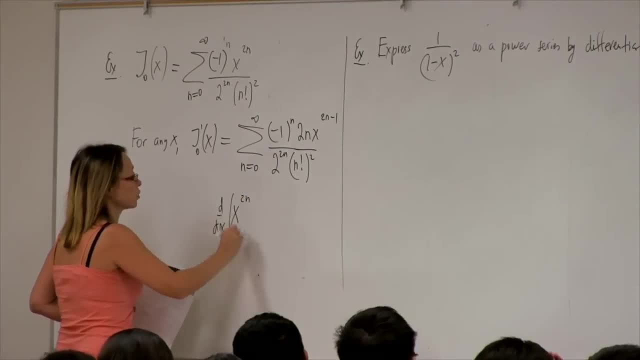 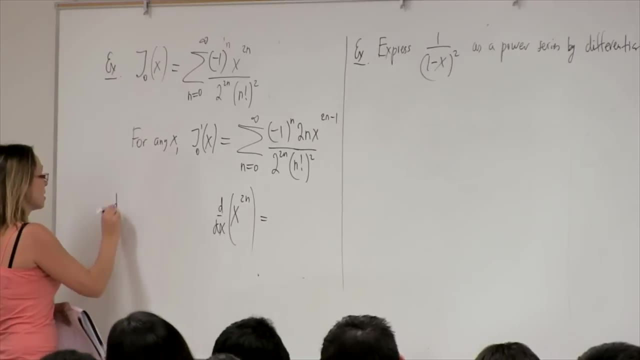 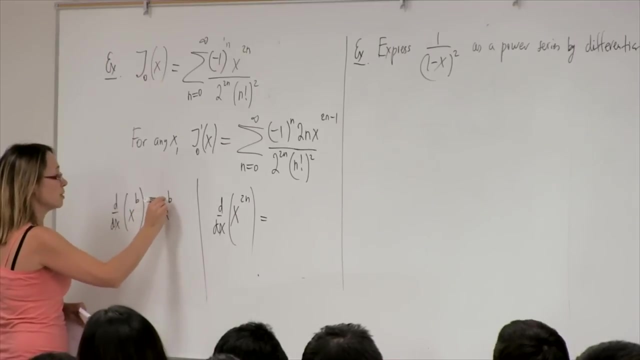 to the 2n and you have to differentiate it with respect to x. so, or, for instance, ddx of x to b, what's that equal to it's? b, x, b-1, right? so here, instead of b, I have 2n, so I have 2n. 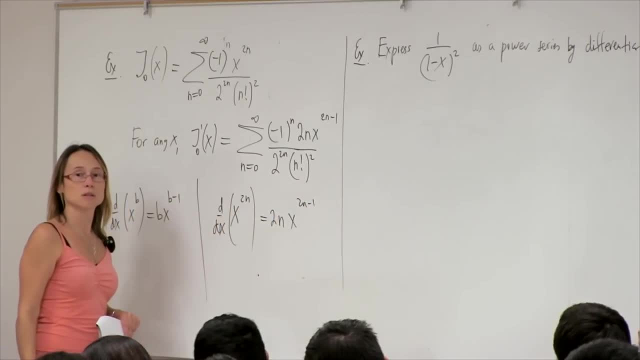 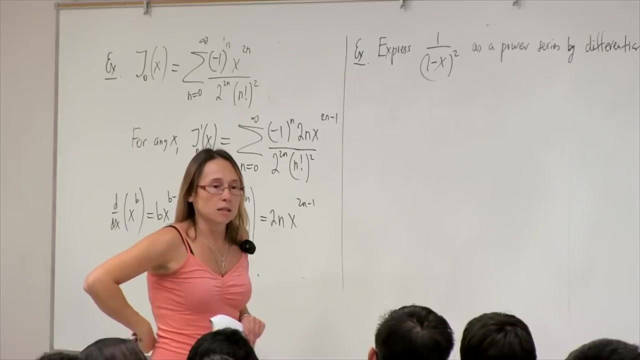 x 2n-1. so this: I just treat 2n as as some number b and use the power rule to differentiate. yes, okay question. so when you derive or integrate inside a power series, are you treating the n like a constant? yes, 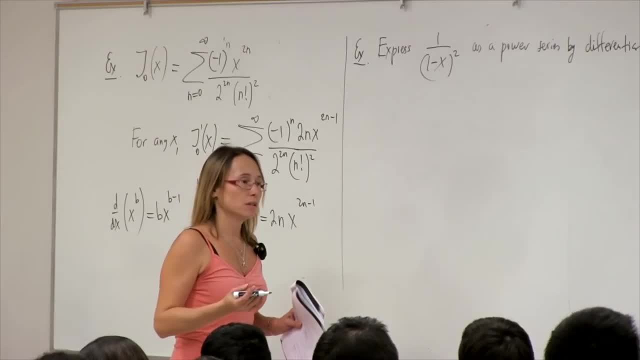 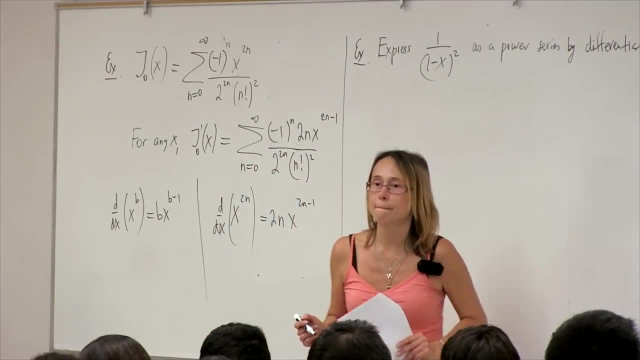 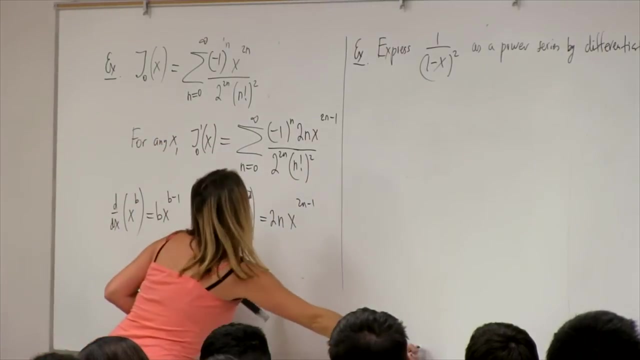 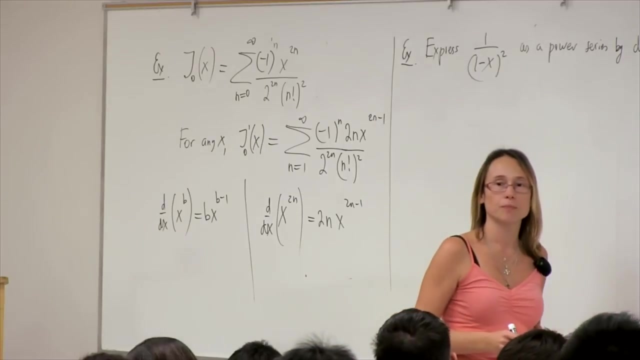 so x is my only variable and n. as far as x is concerned, n is a constant. it does not depend on x. question: should it be from 1 to infinity or 0?? this is from 1, you're right. very good, more questions. 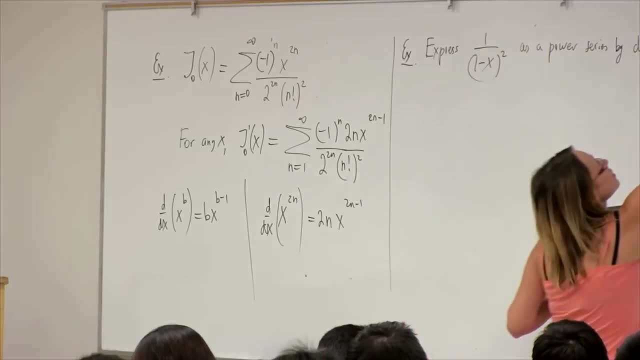 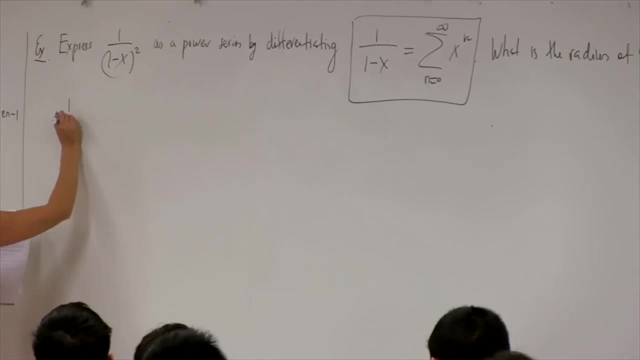 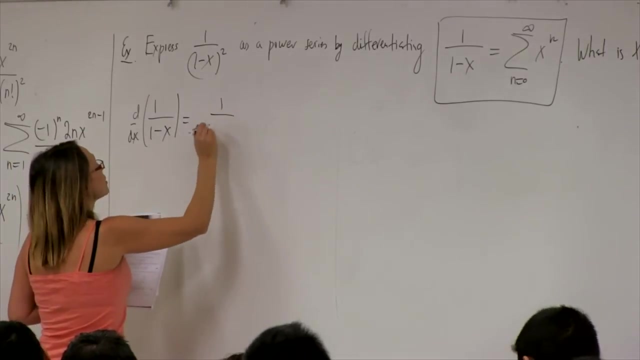 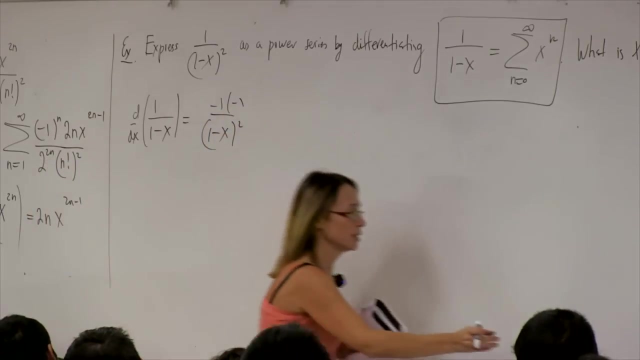 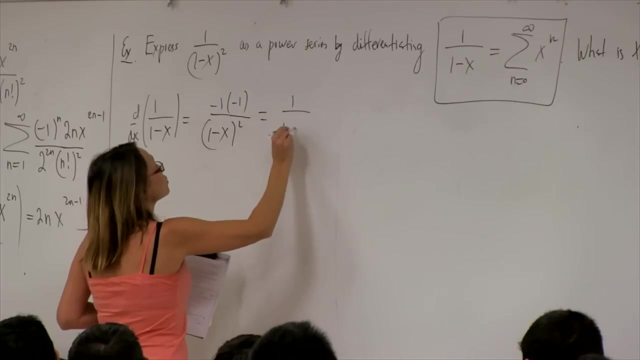 okay, so let's look at this expression and differentiate it both sides. so what's the derivative on the left ddx of this? so I have to use the chain rule. it's 1-x, squared with a minus sign, that is, minus 1, sorry, or I can simplify it to this: 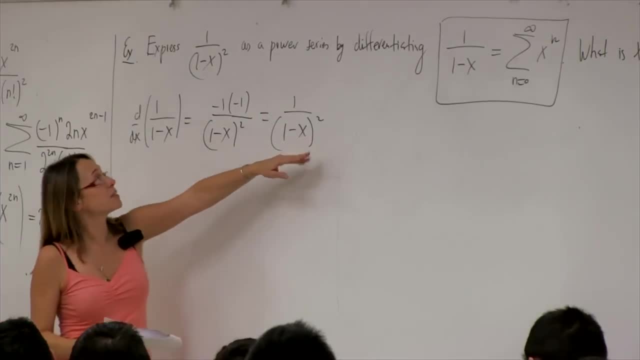 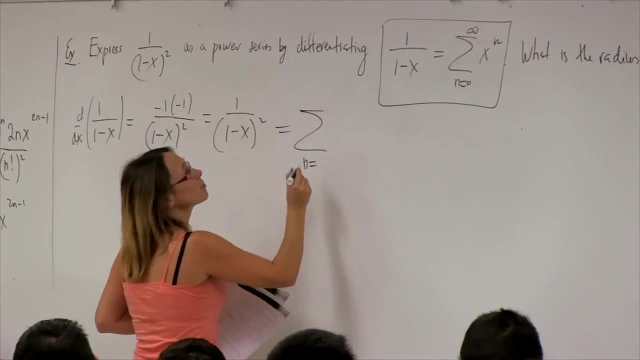 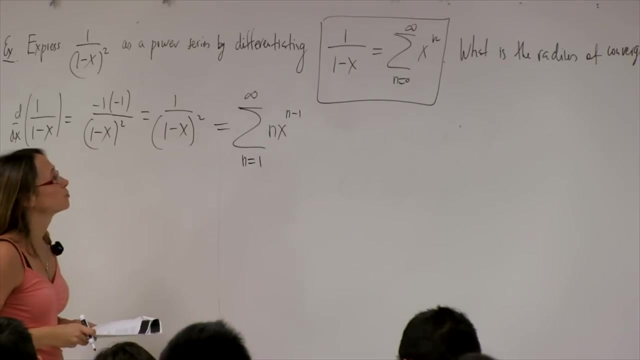 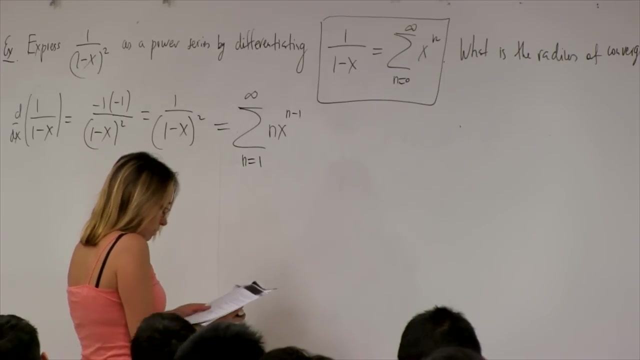 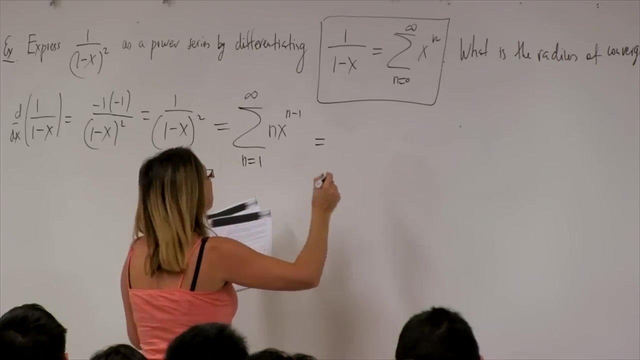 okay, so differentiating the left hand side gives me this function. okay, and now I have to differentiate the right hand side, so I'm going to start with 1 and x to the n-1, okay, so what's that equal to? oh, if we want to express it, 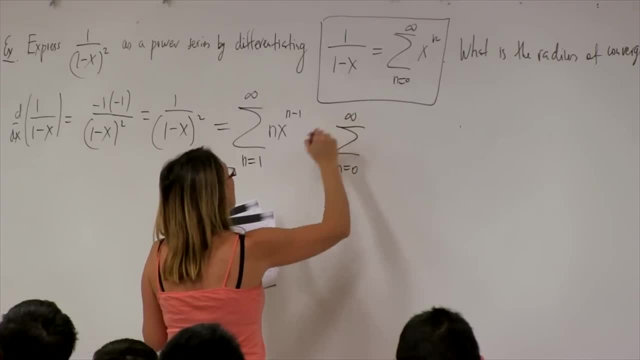 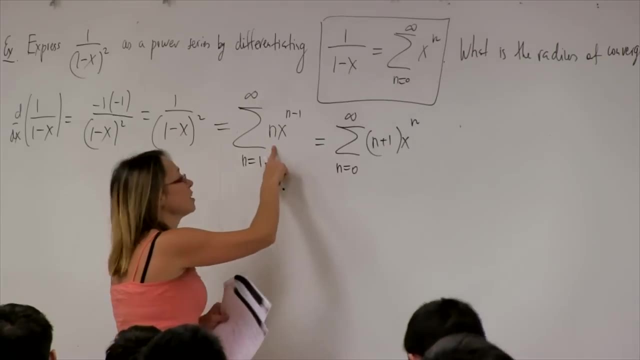 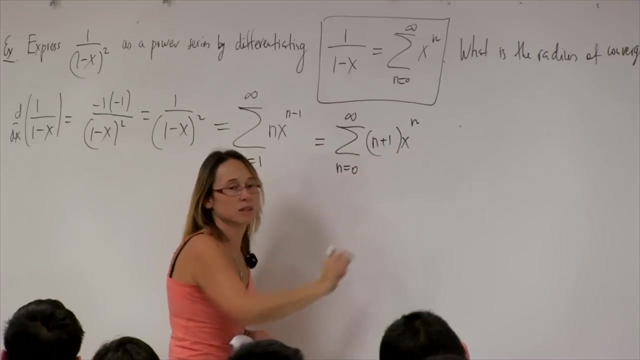 as a power series, starting from 0 actually. so we can say: this is n plus 1 x to the n. basically, I replace each n with n plus 1, then n starts from 0. this becomes n plus 1. n minus 1 becomes n. 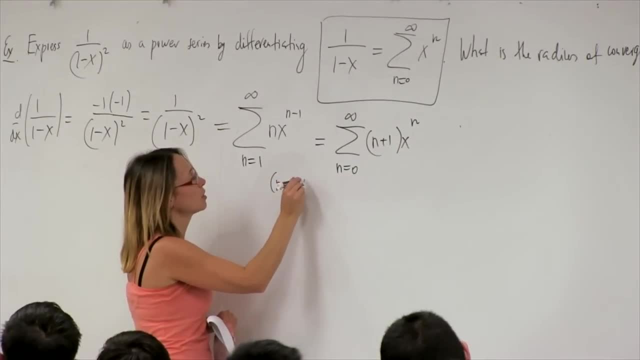 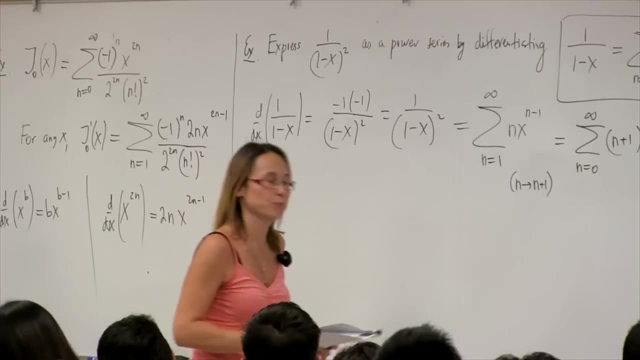 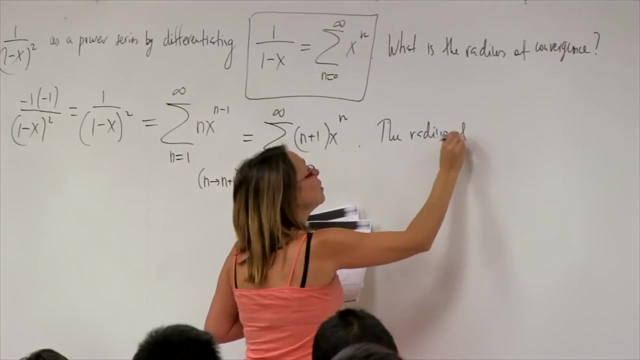 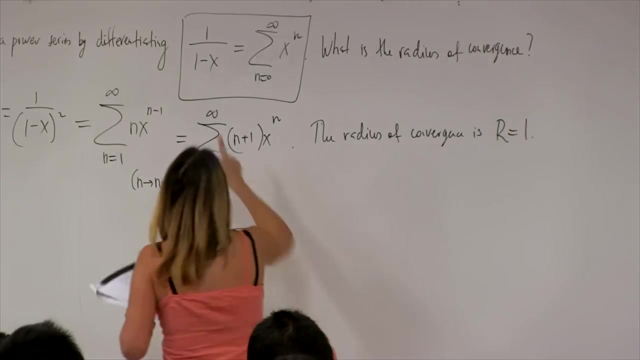 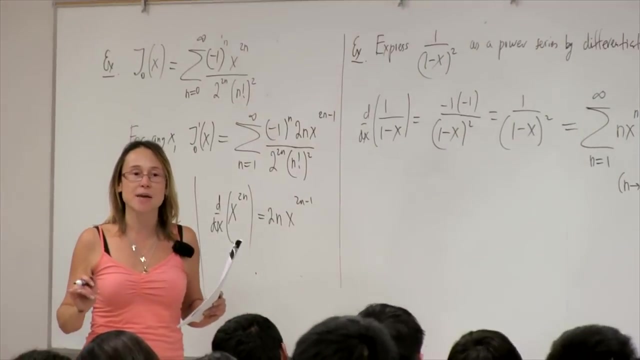 so here the operation is to go from n to n plus 1. these are the same. you can manipulate your series like this: and the radius of convergence? convergence is r equals 1. it's the same as this one. according to the theorem, once we differentiate, the radius of convergence stays the same. 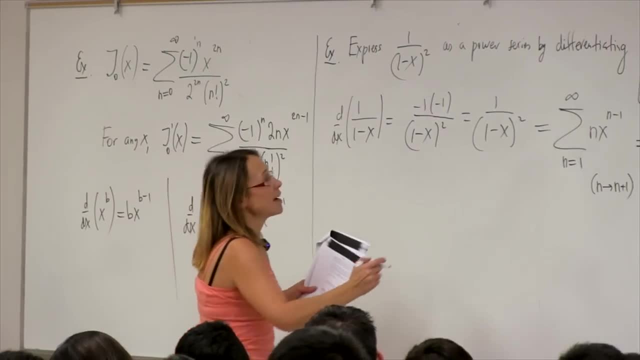 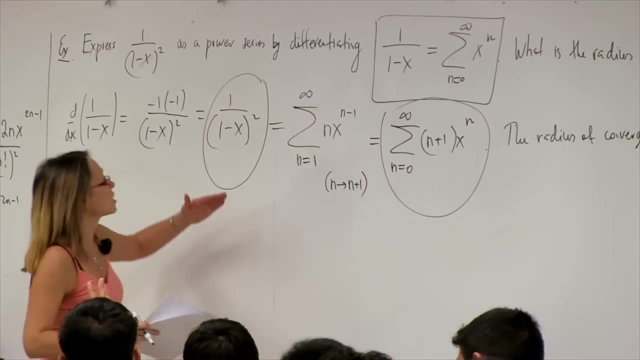 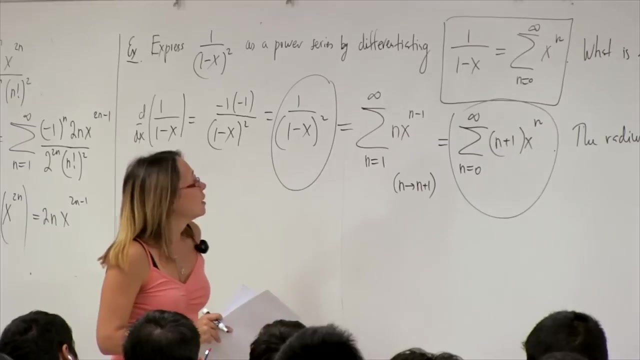 so what does this? what do I achieve by this? I achieve the following: I identify this guy with this representation, so I was able to create a power series representation of this guy by differentiating this question. the value of n is equal to n plus 1. 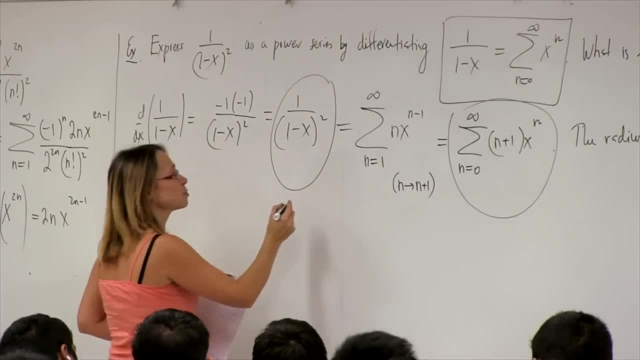 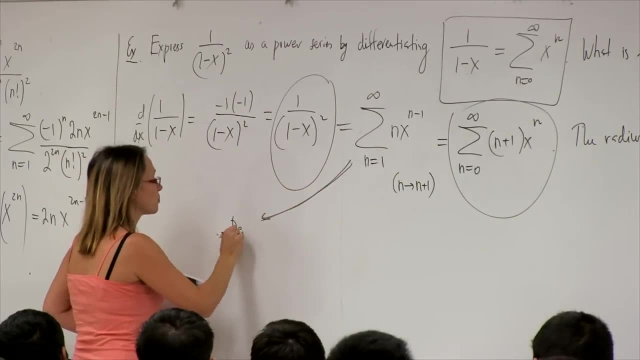 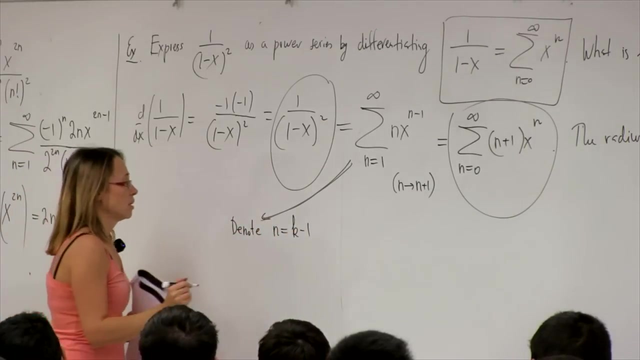 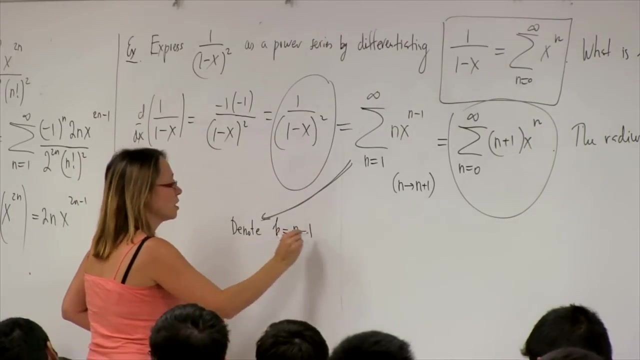 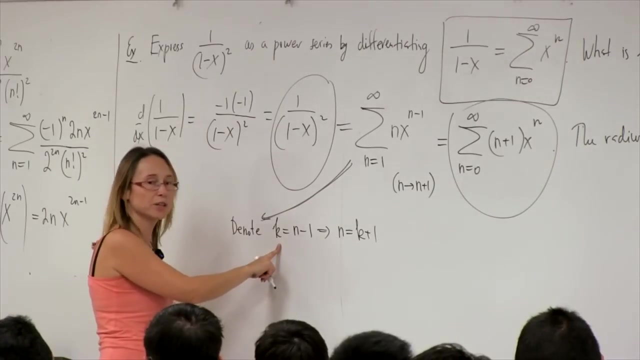 so let me explain this. so let me denote- I'm going to use this and denote: n equals k minus 1, I'm sorry, k. k equals n minus 1, which means that n equals k plus 1. I introduce a new integer number which is related to n, like this: 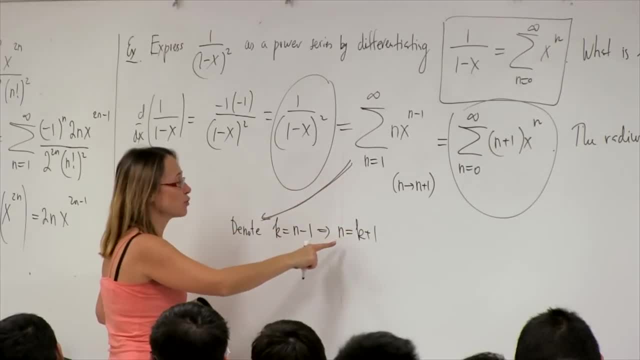 ok, and I'm going to rewrite this in terms of k. is that right? n minus 1. yes, so I'm going to use this expression and rewrite it in terms of k. so every time I see n, I replace it with k plus 1. every time I see n minus 1. 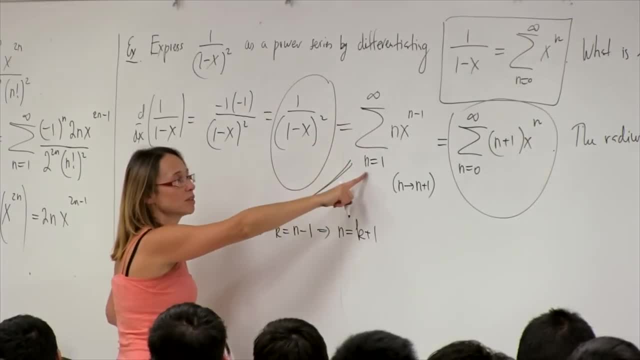 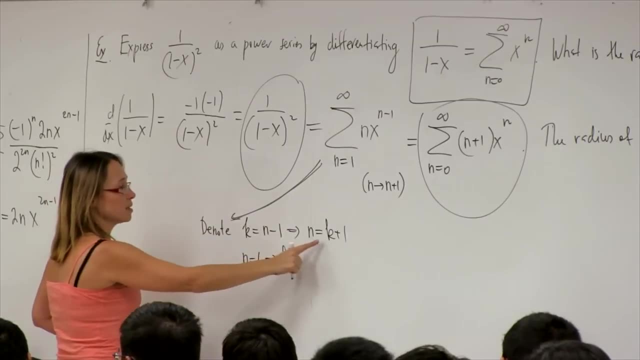 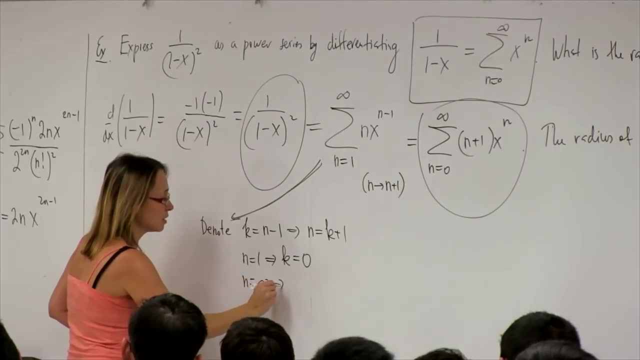 I replace it with k, so let's do that. I also need to deal with the limits. so if n equals 1, then k is equal to 0. if n is equal to infinity, k is also infinity. right question, it's a slightly different one. 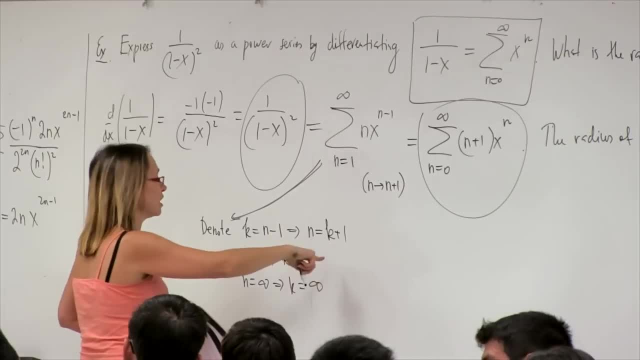 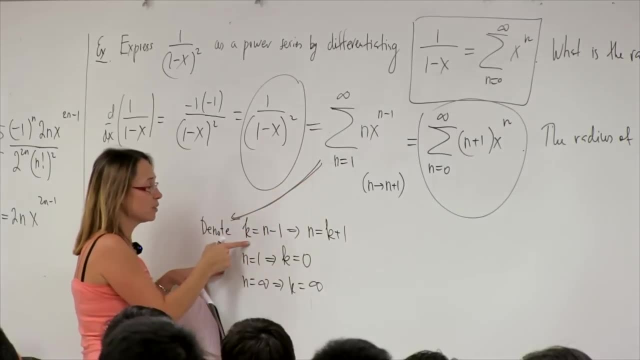 wait, wait. I haven't finished. who's this one, though? ok, so if it's unrelated, let me finish. ok, so this is my correspondence. I have integers n and I have integers k, and they differ by one unit, so I'm rewriting this expression in terms of k. 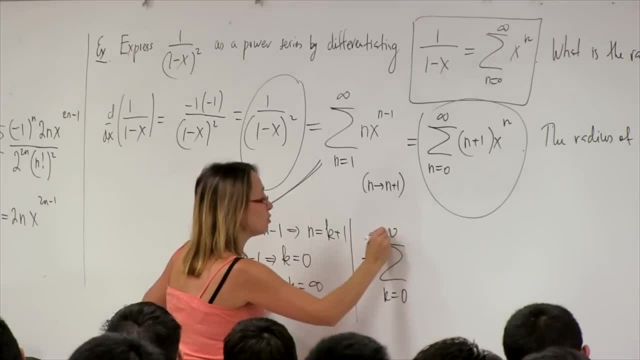 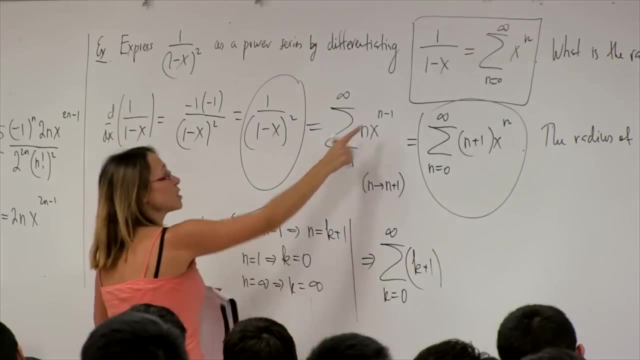 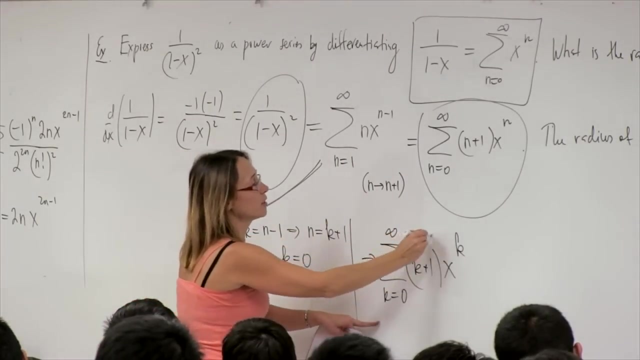 so k goes from 0 to infinity. so when I see n, I put k plus 1. when I see n minus 1, I put k. ok, so this is the same as this. and now I go here and I I can call it k or I can call it l. 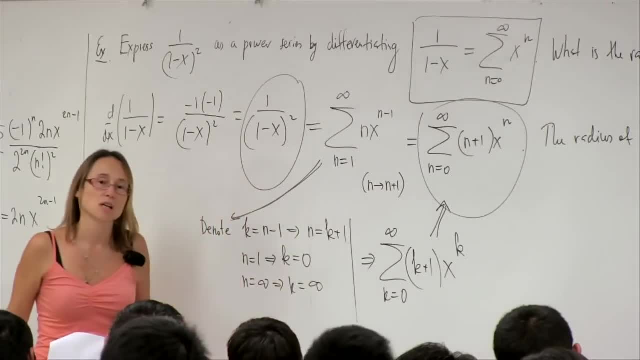 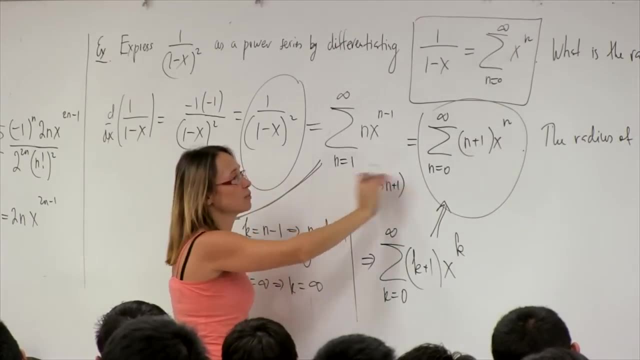 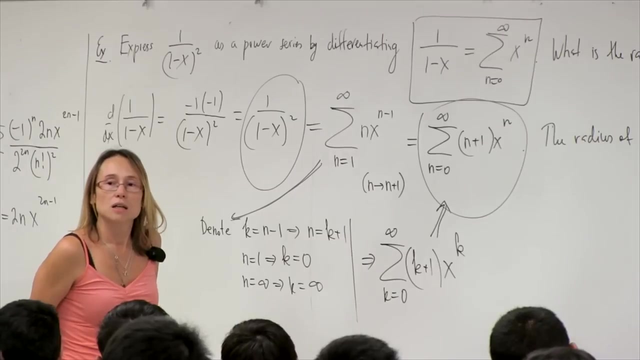 m any other letter, I go back to the n notation. ok, so this is how you can manipulate series. if you want to change the starting point, if you want to start from a different letter, you have to introduce a new letter. question, I'm sorry. what theorem dictated that? 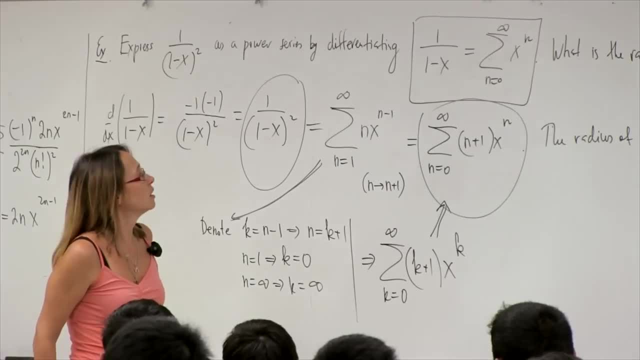 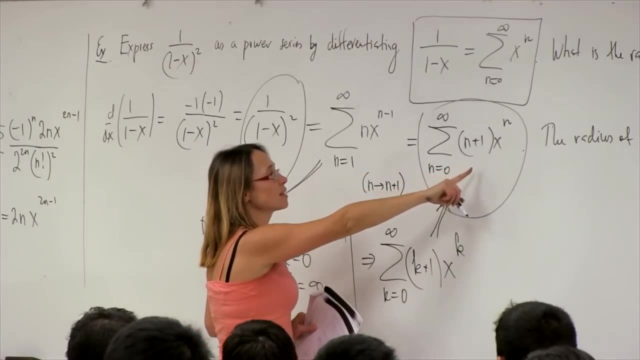 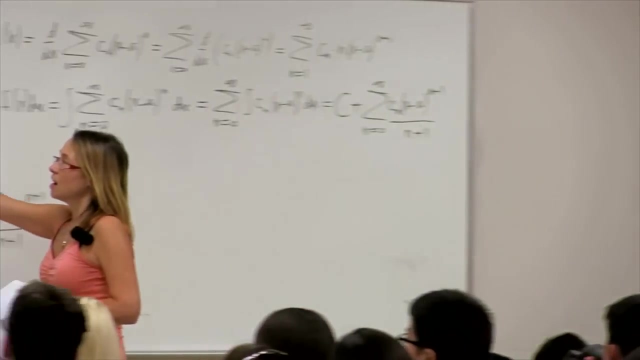 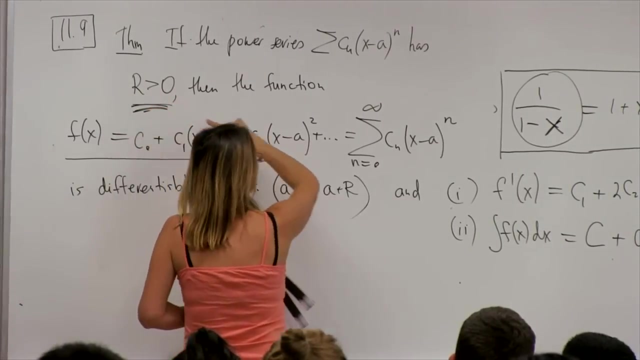 the sum of the series n plus 1 times x to the n converged. oh so this is dictated by this theorem, which states that if my given series converges with a given radius, then I can differentiate term by term and the radius of convergence persists. so it's a very powerful statement. 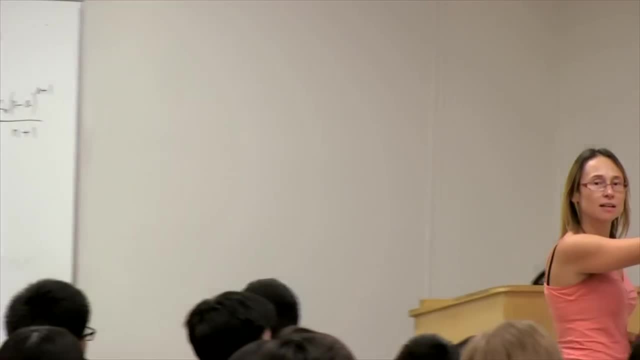 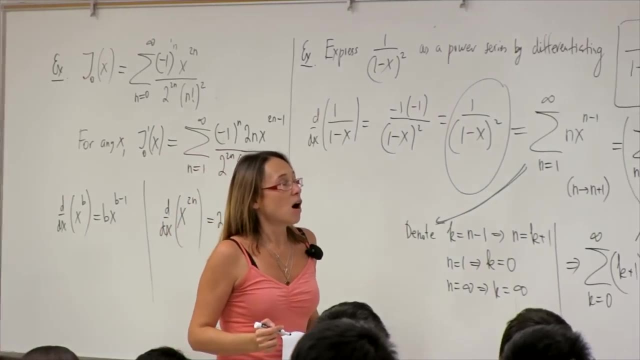 I don't even have to worry about it here. I could prove it directly, but I don't have to because of that theorem question: why is it equal to 1 and not less than 1?? oh, r is equal to 1. r equals to 1 is equivalent to this statement. 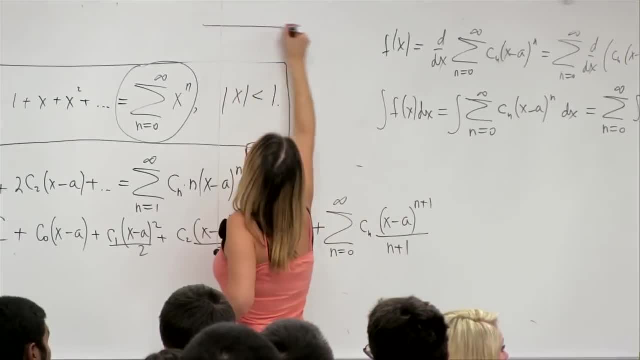 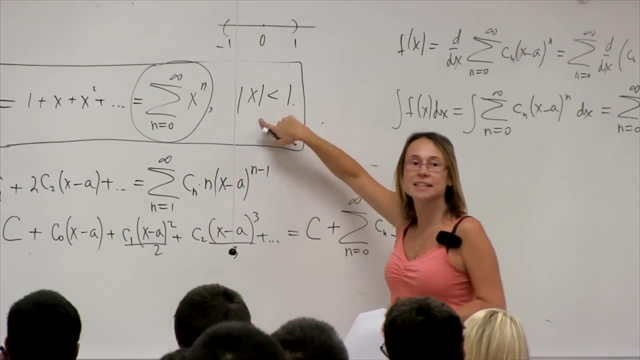 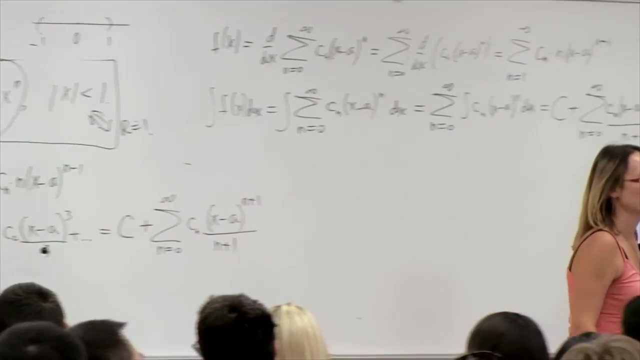 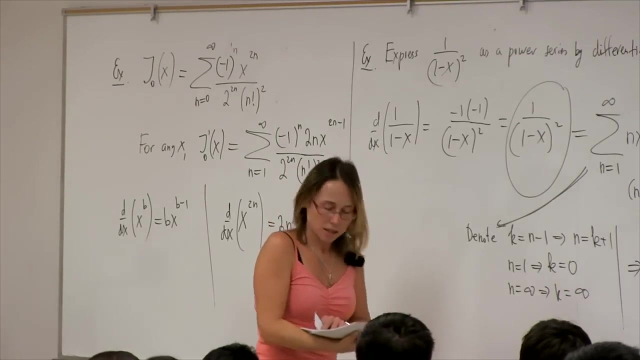 radius of convergence equaling 1 is equivalent to saying that it converges between minus 1 and 1, like this: it's the same thing as this. so I could say radius of convergence is 1. ok, fine, let me give you some more examples, so I'll do one with integration. 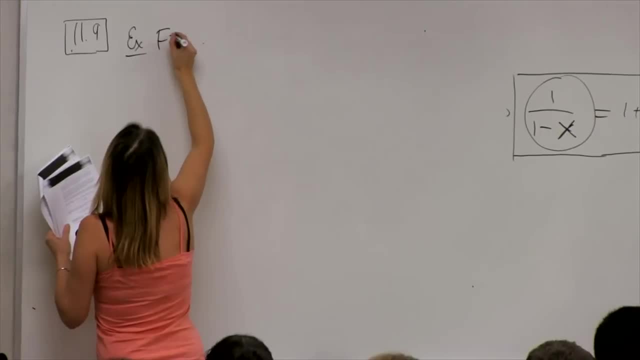 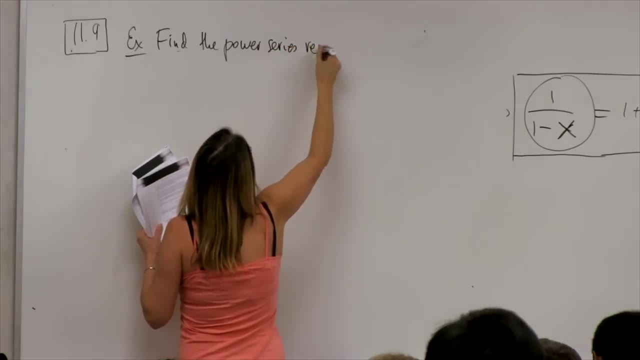 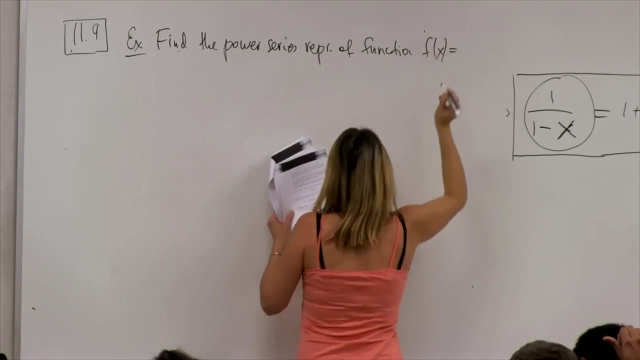 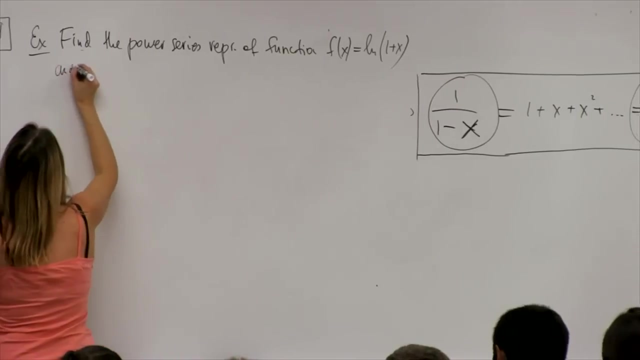 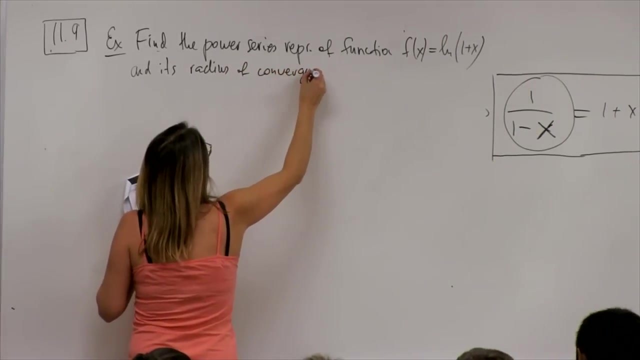 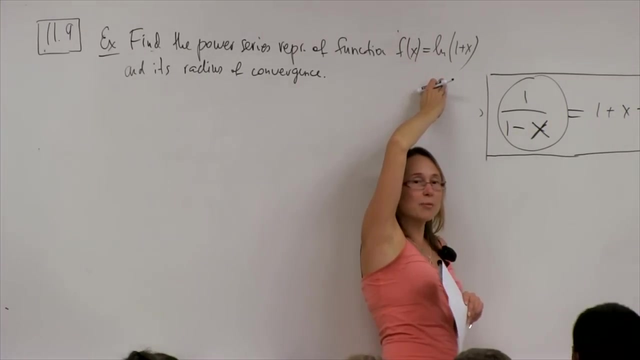 so let's find the power series representation of function f of x equals log of 1 plus x and its radius of convergence. ok, how can I represent the function log as a power series? it's absolutely not clear how to do it from first principles, right. 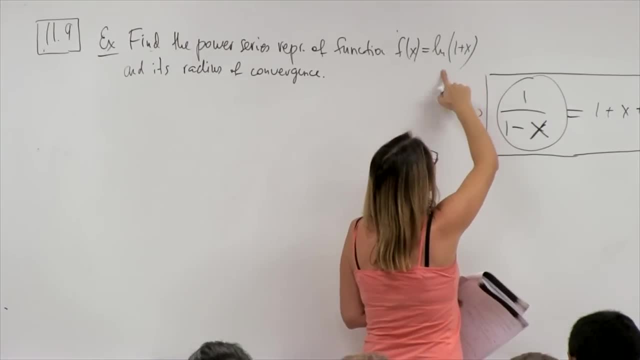 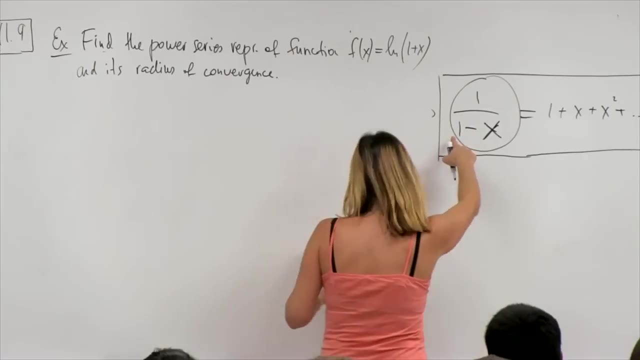 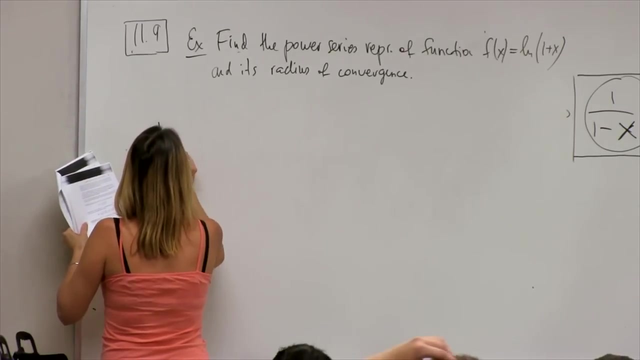 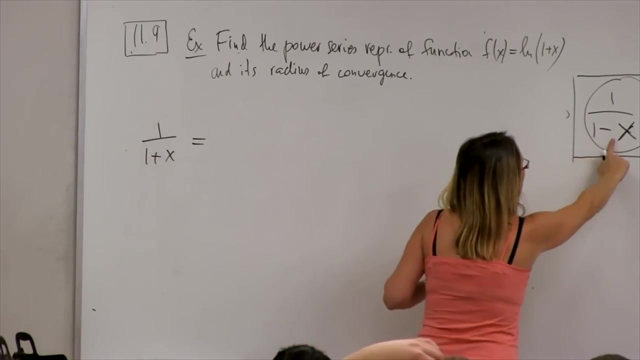 but I notice that this function is related to this function by the operation of taking the antiderivative. ok, so I take this expression. um, so let me first write: uh, it's not quite this, ok, so I want to look at this function: 1 over 1 plus x. 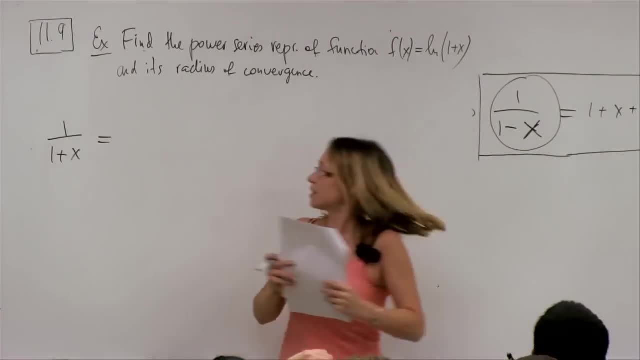 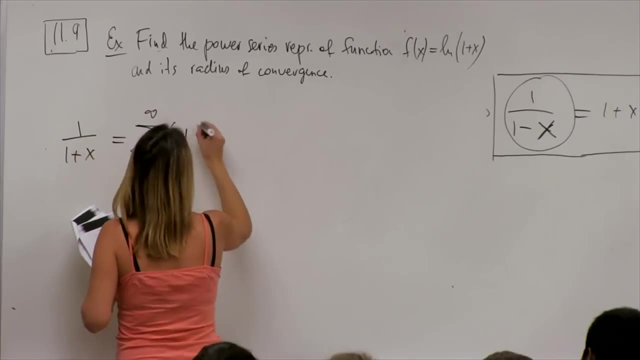 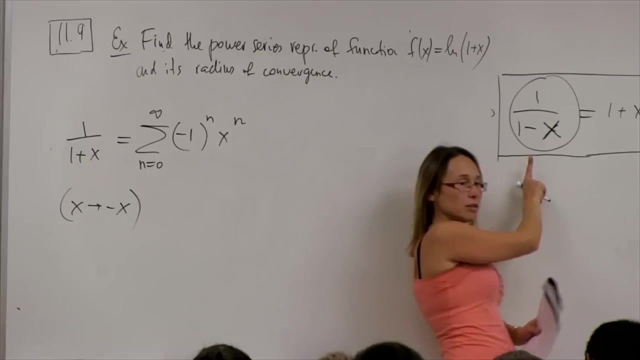 it's very much related to this one. if I replace x with minus x, so this is equal to minus x, minus 1 to the n, x to the n, right by the operation x to minus x. uh, implemented for my original power series. so this one is easy. 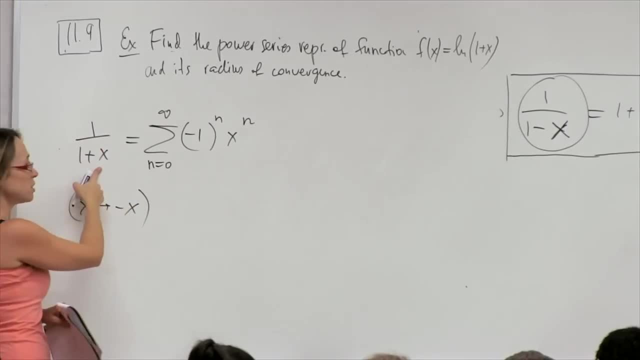 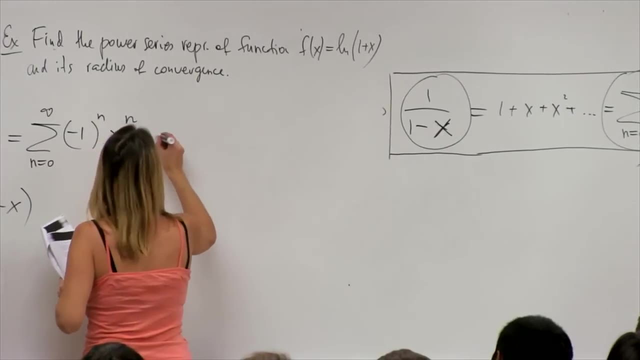 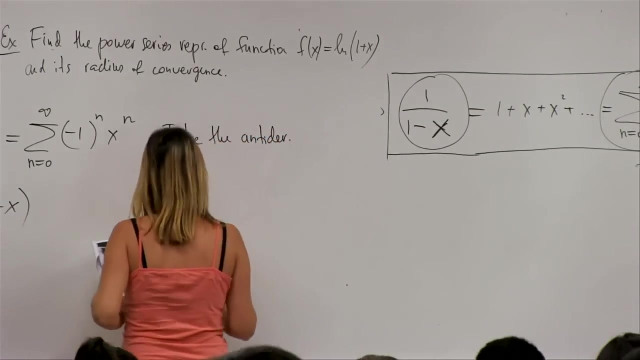 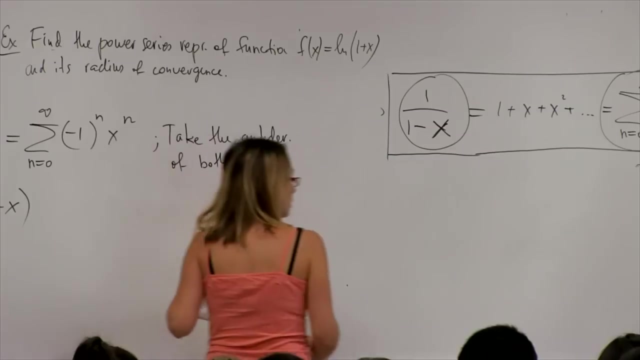 and now I notice that if I take the antiderivative of the left hand side, I get exactly this function. ok, so let's do that: take the antiderivative of both sides. so what do I get? so on the left, oh, and the radius of convergence here. 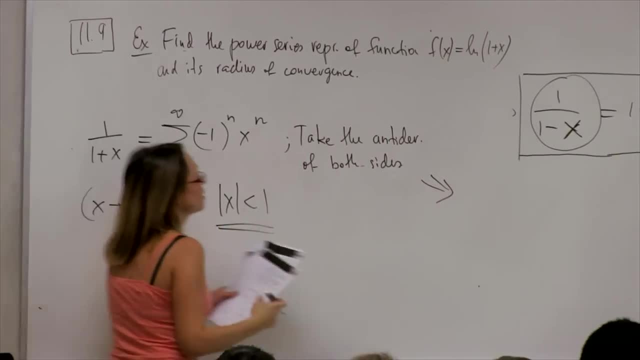 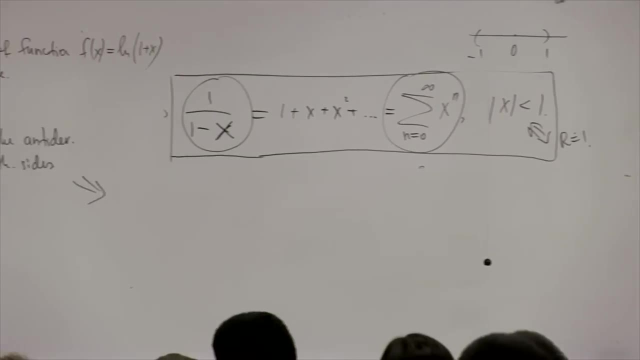 again is x is less than 1. it follows from the following fact: for this one, the radius of convergence is 1, the operation is x to minus x. the absolute value doesn't care, so it's the same radius of convergence. so I know everything about this one. 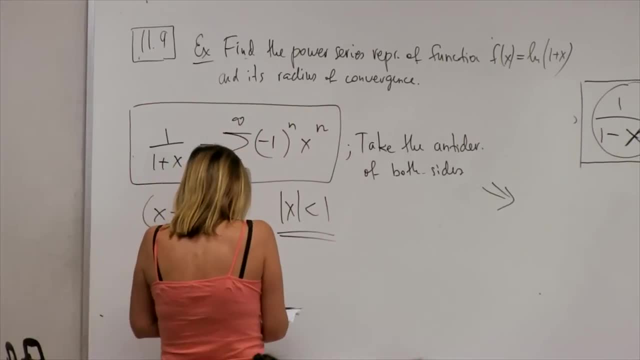 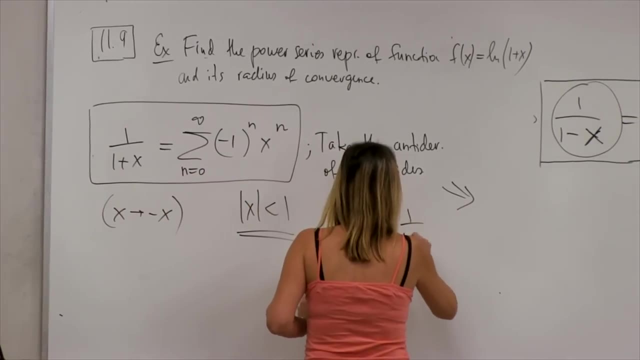 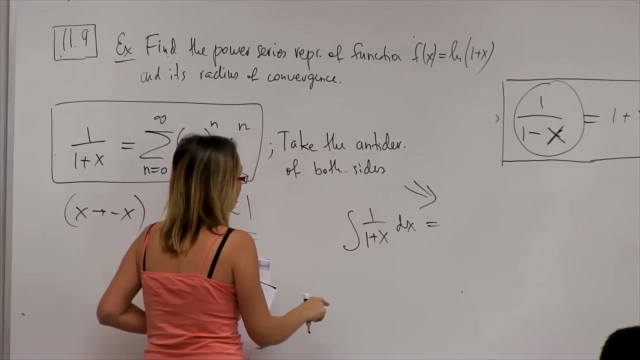 this is going to be my starting point. ok, uh, and let me take the antiderivative of both sides. so I have the antiderivative of 1 plus x, dx. uh, what's that? equal to what? when I um integrate that, what's the antiderivative? 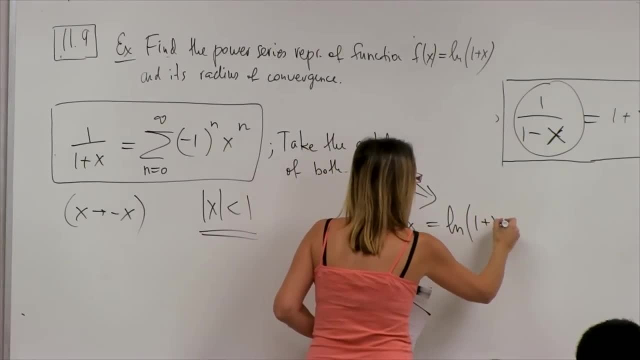 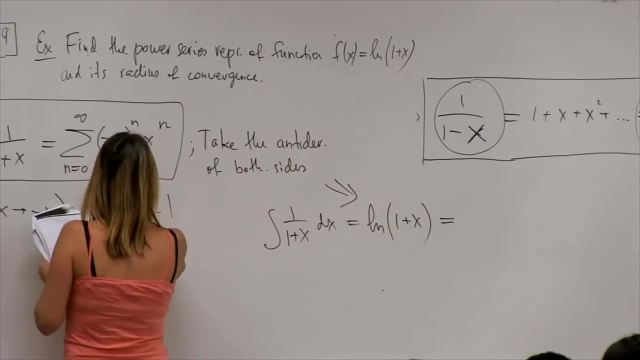 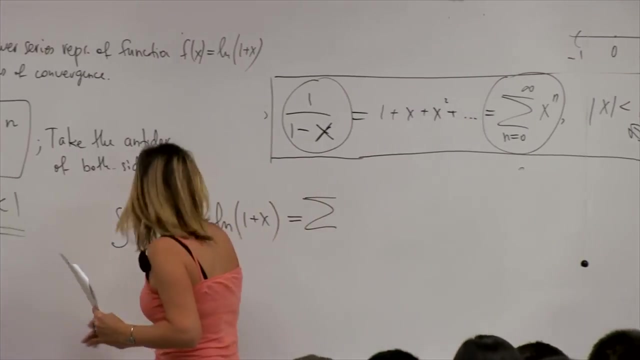 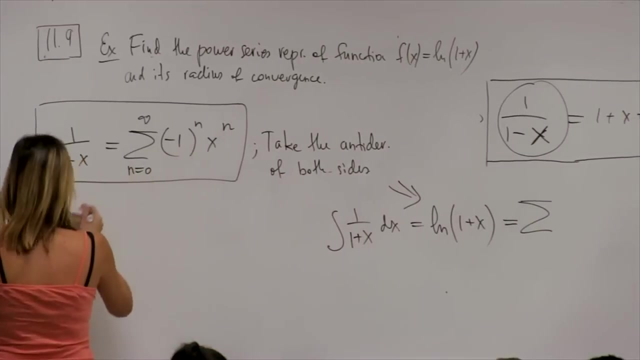 that's just log of 1 plus x. ok, um, and on the right, I'm going to take the integral of these things. so actually, for for clarity, let me write this down as, uh, a bunch of terms. so it's x minus x plus x squared, minus x cubed. 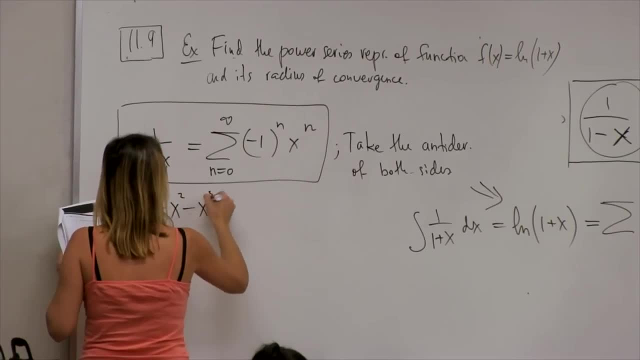 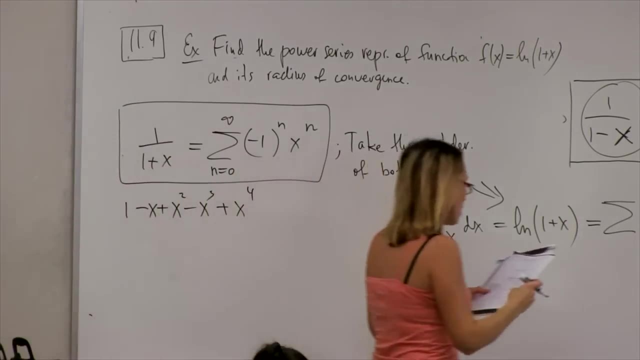 this is this alternating series, plus x to the fourth. so I'm going to take antiderivatives of these things. what are they? x minus x squared over 2 plus x to the fourth. so I'm going to take antiderivatives of these things. 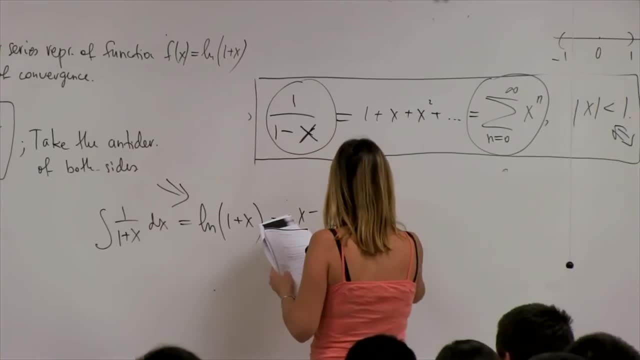 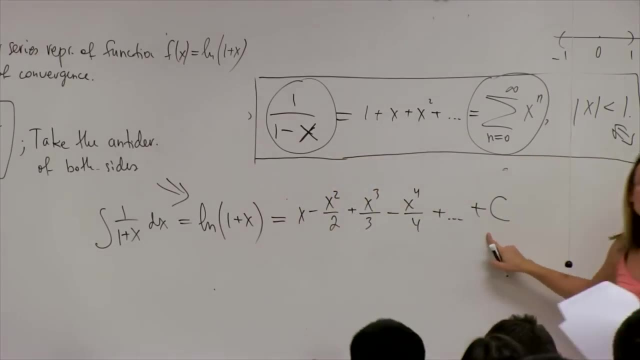 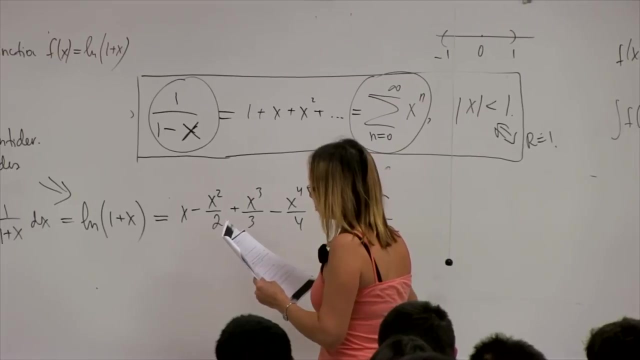 what are they? x minus 2 plus x cubed over 3, minus x 4 over 4. and don't forget plus c. right, we always have to have plus c. ok, so I'm almost done here because, uh, on the left I have. 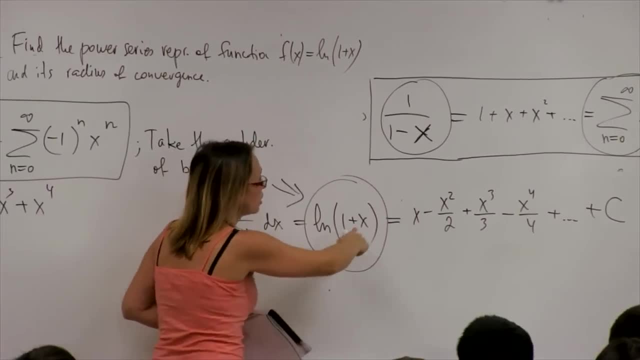 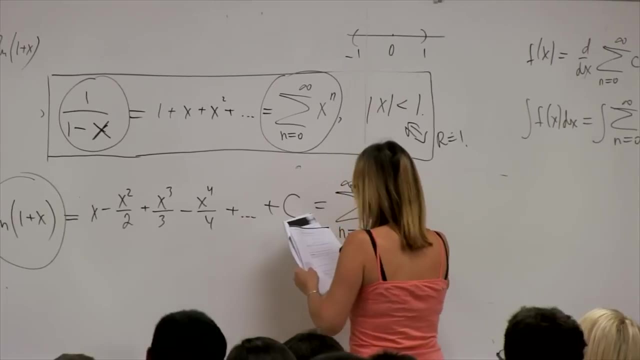 the desired function that they ask. they're asking for, and on the right I have something that looks like a power series. so let's, let's write it down as a power series. starting from 1, the power of minus 1 is n minus 1. x to the n. 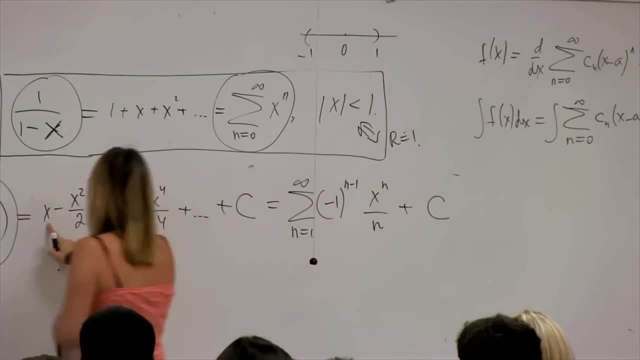 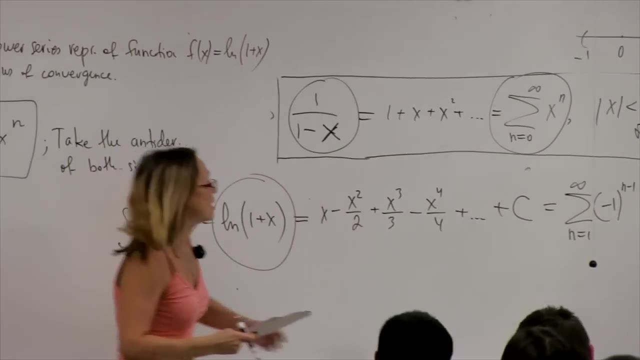 over n plus c. right, we have x to the n and I divide by n and I have to add c. so the last step is to find the constant of integration, and that's very easy. how can we find c? c should hold for any value of x. 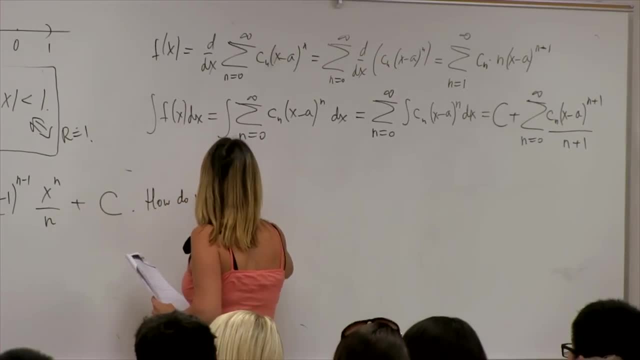 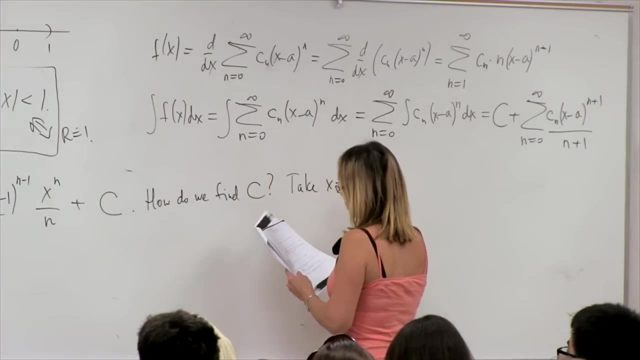 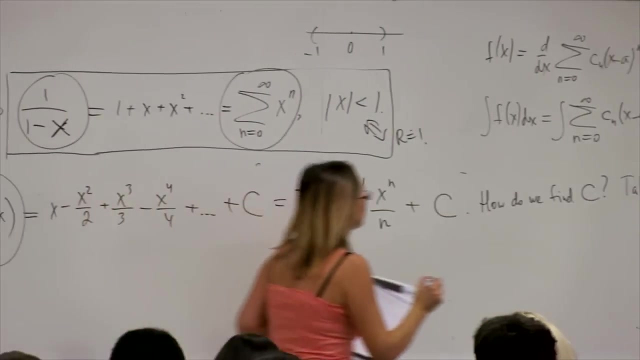 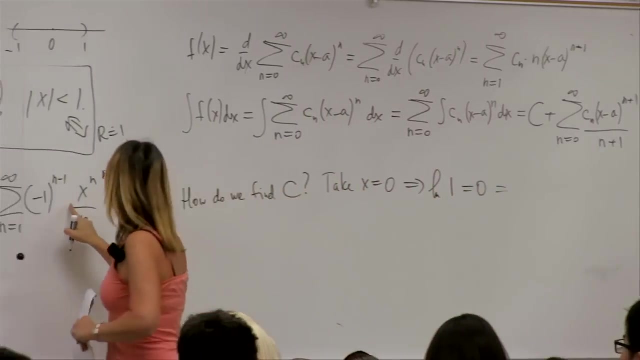 so take x to the n over n plus c, right, x to the n and I divide, x equals 0. so on the left I have the logarithm of 1, which is 0, and on the right, when I substitute x equals 0 all the terms. 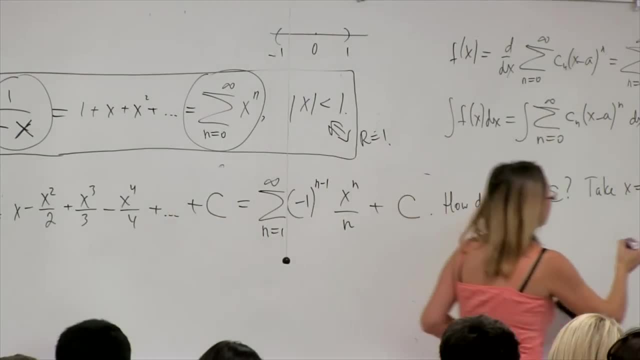 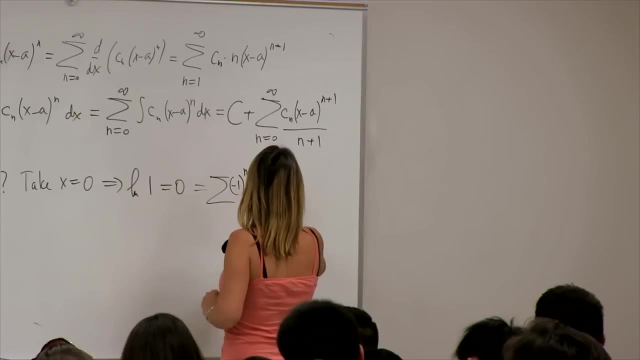 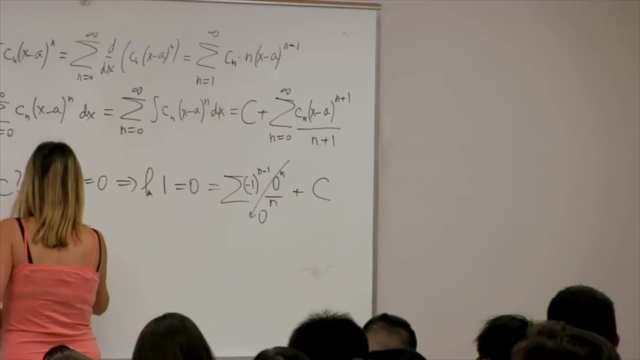 are equal to 0 and I just have c, so I have minus 1 n, minus 1, 0 to the n over n plus c, so this is 0. so I conclude that c equals 0. so let me write down the answer. I'll get rid of this. 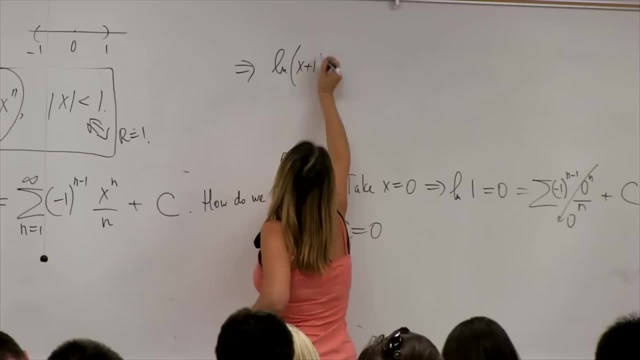 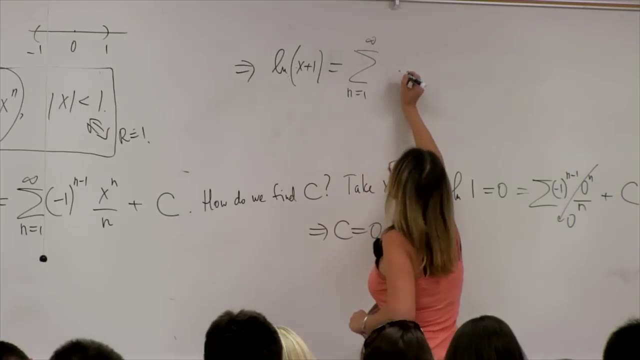 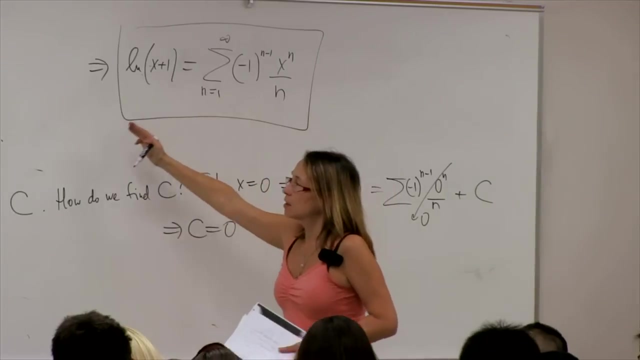 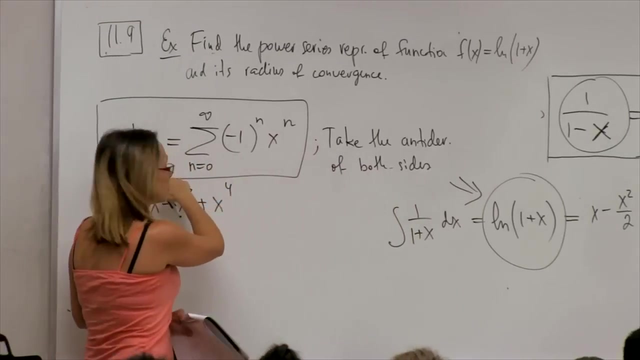 so the answer is: the function log of x plus 1 is given by the following power series, and this is something that we could never guess right. we were only able to obtain this result by taking the antiderivative of this, and we know a few things. 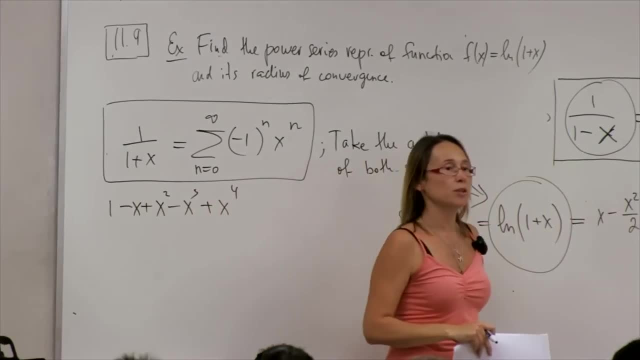 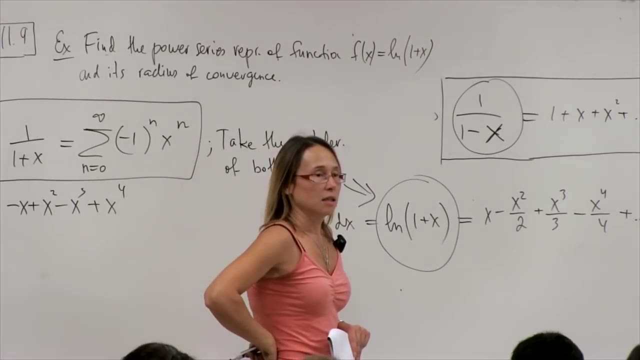 about this power series because it's very similar to the starting point. question um: the last time you did a problem, you used n as if it were a constant and then differentiate with respect to x. could you do the same thing with that power series with respect to x? 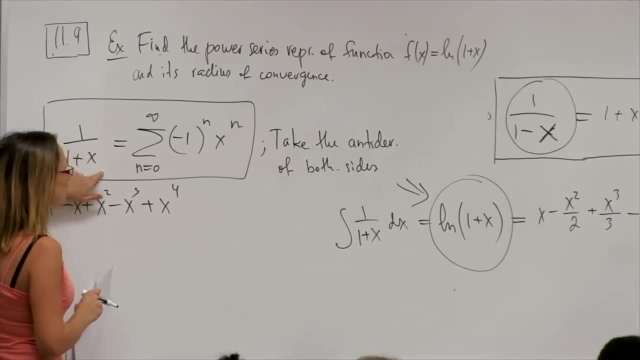 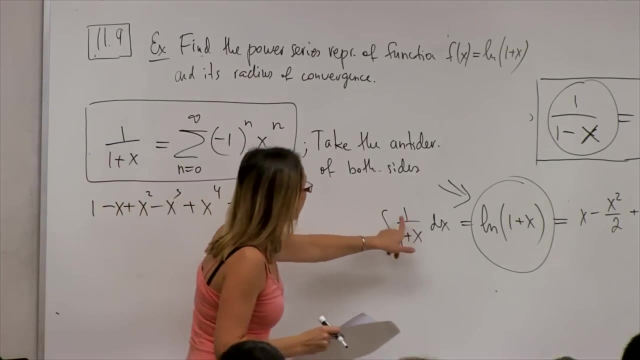 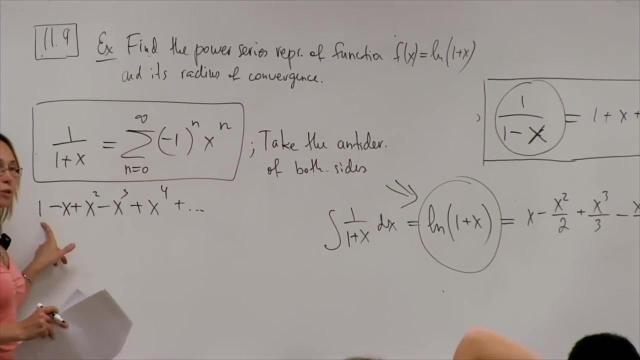 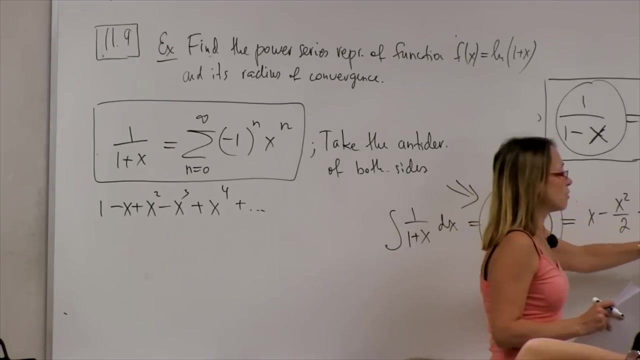 here. yes, I absolutely, I. uh. so I look at the left hand side and I integrate with respect to x, and then I integrate the right hand side, and then I integrate it with respect to x. I get x. this is minus x squared over 2 plus x cubed. 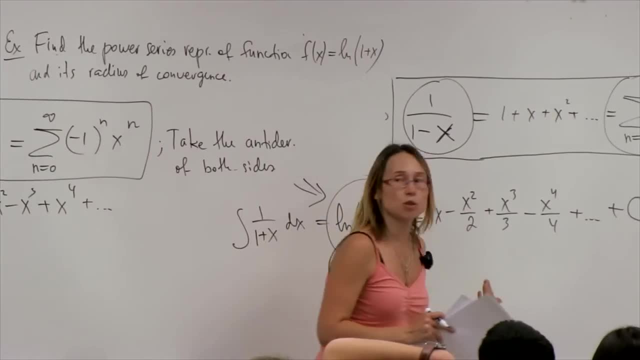 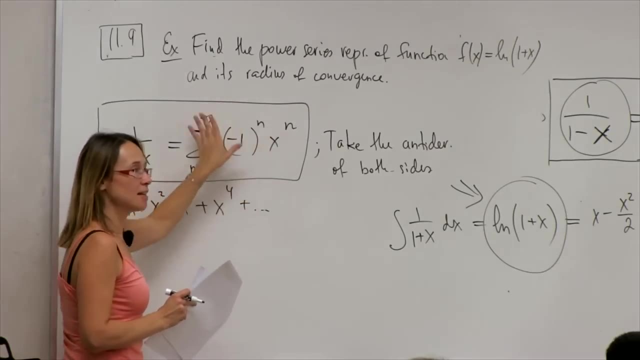 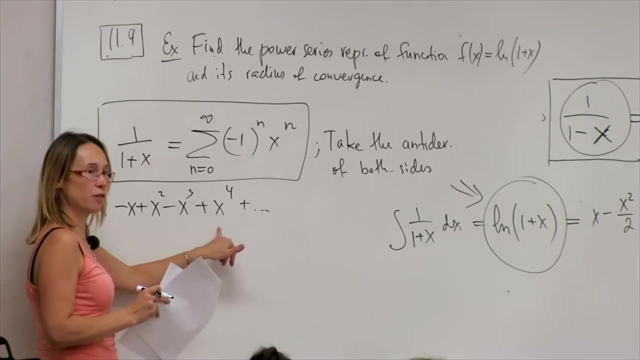 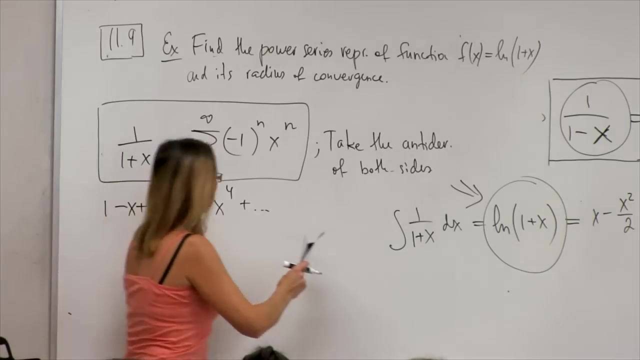 over 3 and so on. so, uh, don't let n confuse you. uh, n disappears completely as soon as you get rid of the sigma notation. right, if you, you have this very concise and nice sigma notation which contains n. you just uh, operate with x and then 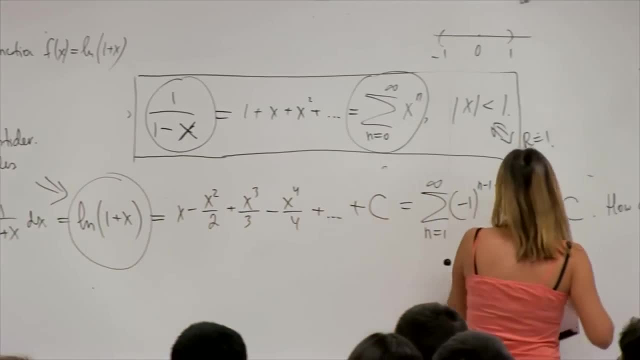 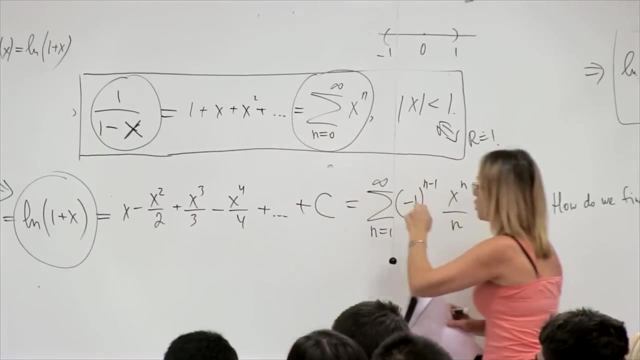 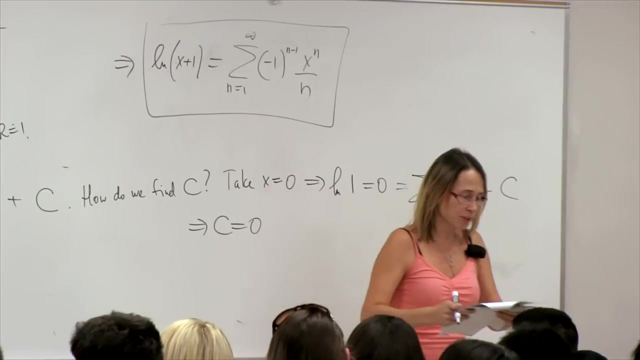 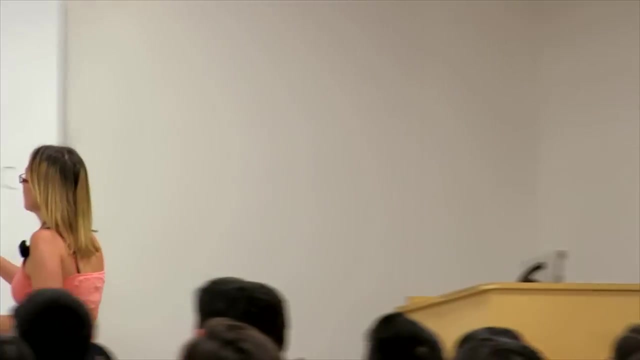 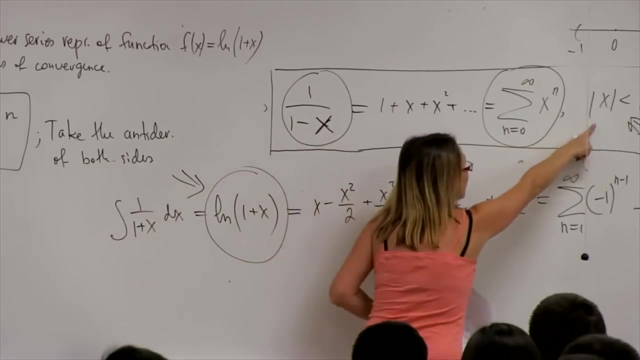 you can. so you take this, integrate it, and then you can rewrite this in terms of the power series. okay, by identifying what power of x corresponds to what coefficient, right, okay, so, uh, the radius of convergence again is one, because of the theory, the original radius of convergence. 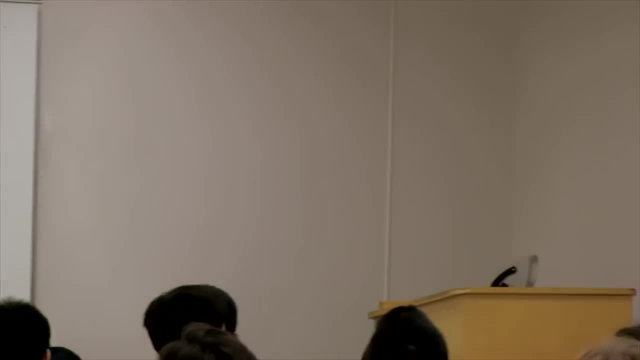 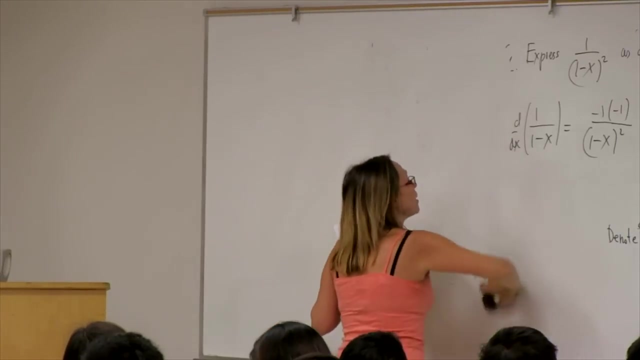 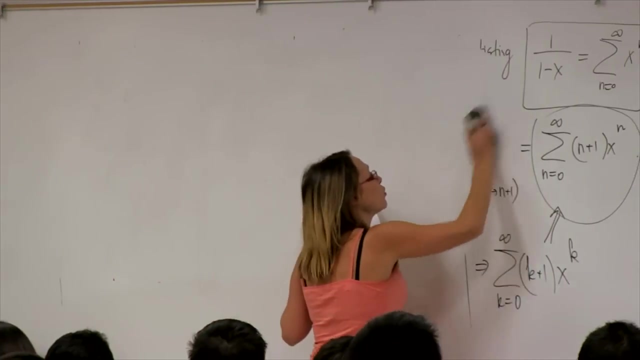 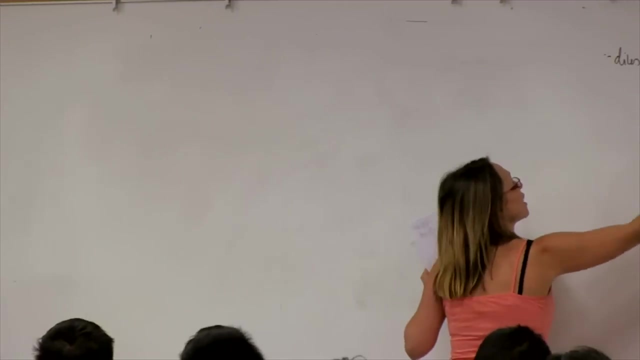 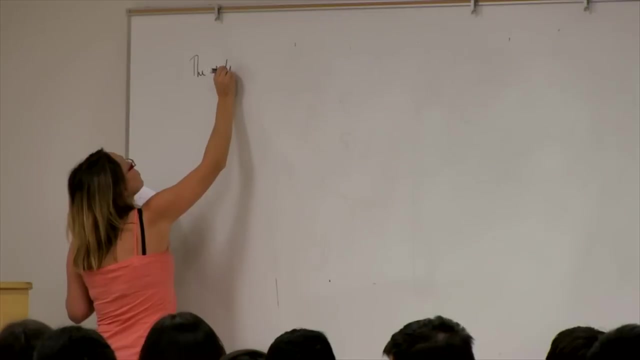 is one, and so is the radius of convergence of uh, the uh, integral. now let me make a very important statement. so radius of convergence is only part of the story, uh of convergence, and sometimes the interval of convergence can be different when we differentiate or integrate. so the radius 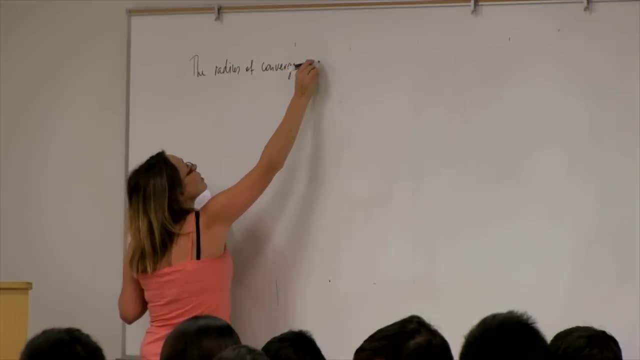 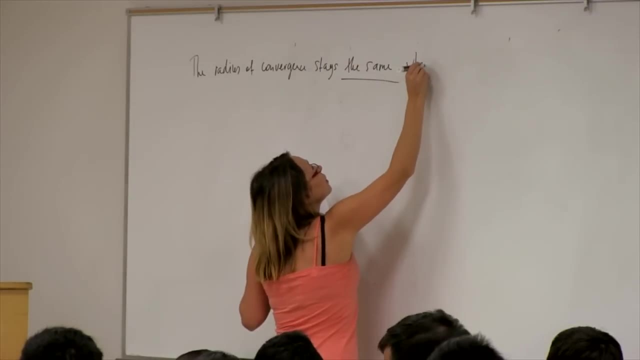 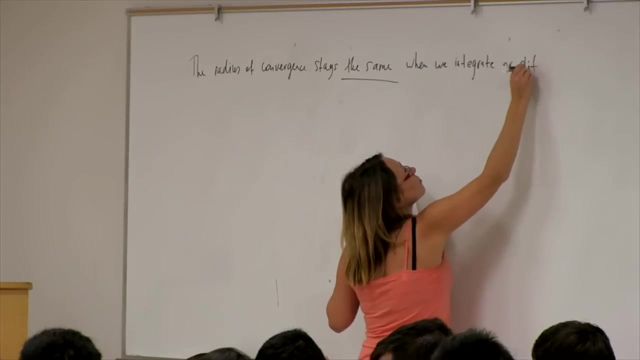 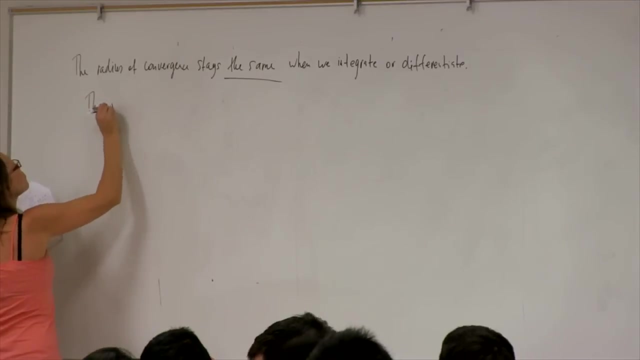 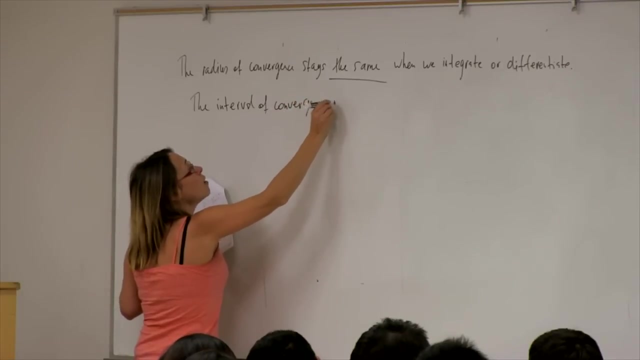 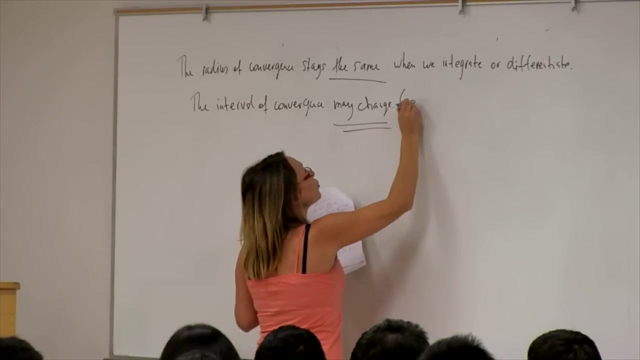 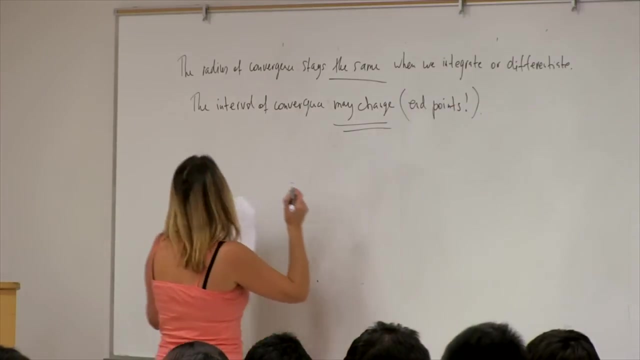 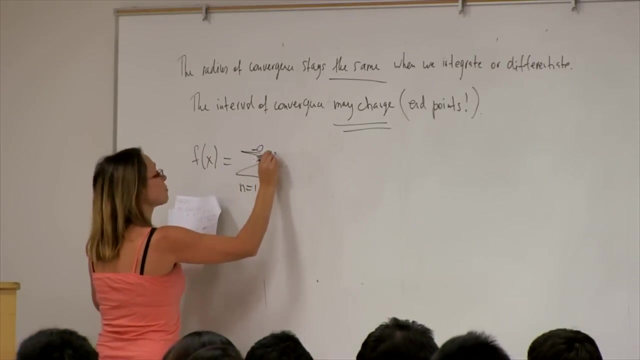 of convergence stays the same. when we integrate or differentiate, the interval of convergence of convergence may change, and here in brackets i put endpoints and the next example. so let's consider the function f given by the following power series: x to the n over n squared. okay, i define. 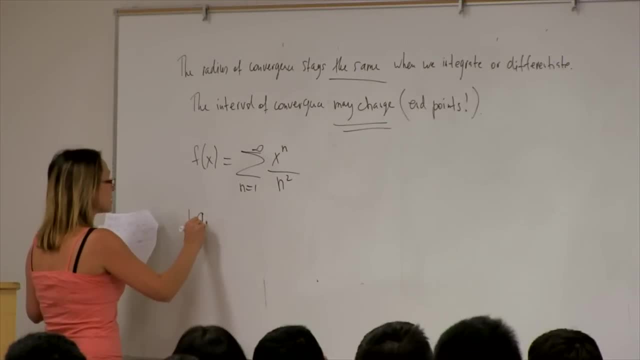 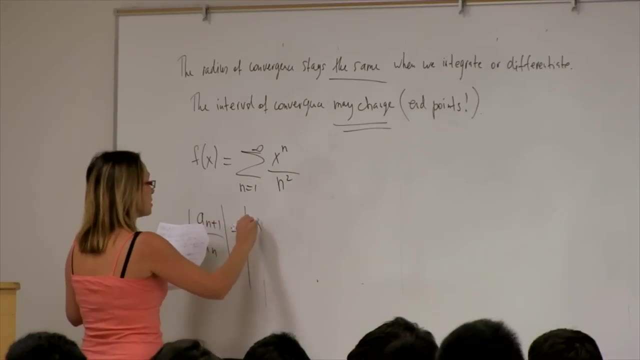 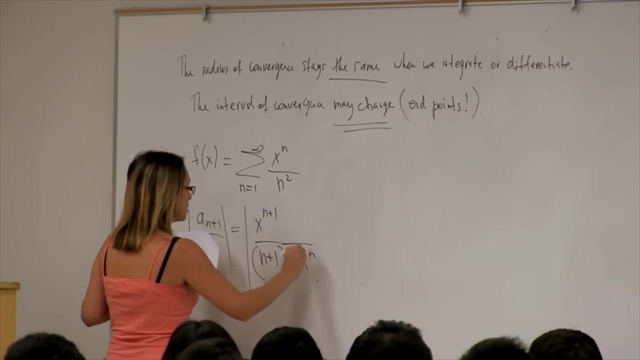 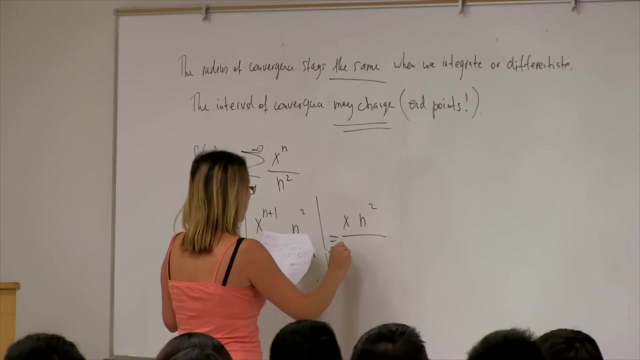 this function like this: uh, let's do the uh, let's investigate the convergence of this uh thing by using the ratio test, so x n plus 1 divided by x n n squared. i can simplify a little bit: x n squared, n plus 1 squared as n. 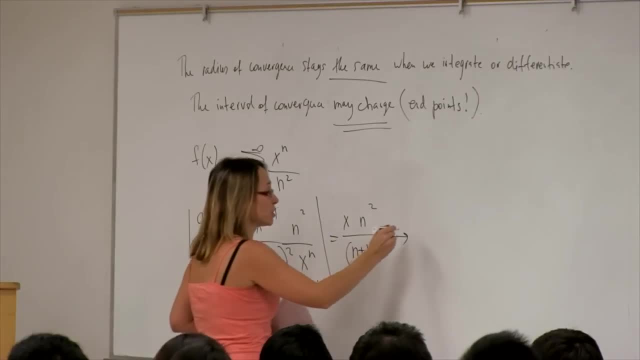 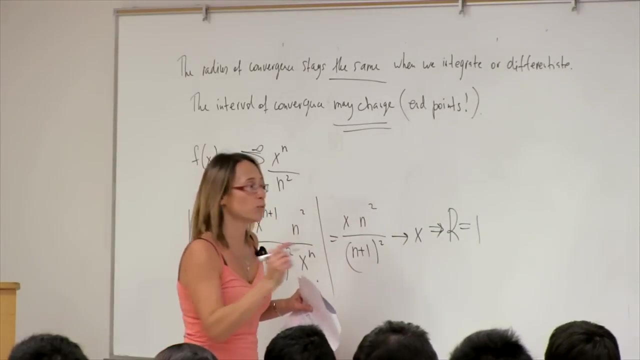 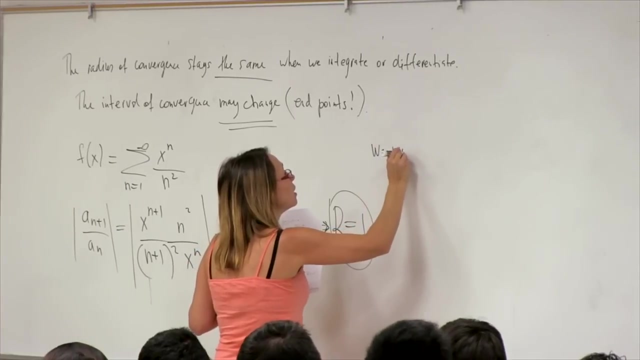 goes to infinity. you can see that the power of n is the same for both, so this tends to x. therefore, the radius, uh, its absolute value is less than 1, so that gives me the radius of convergence 1. how about the interval of convergence we need? 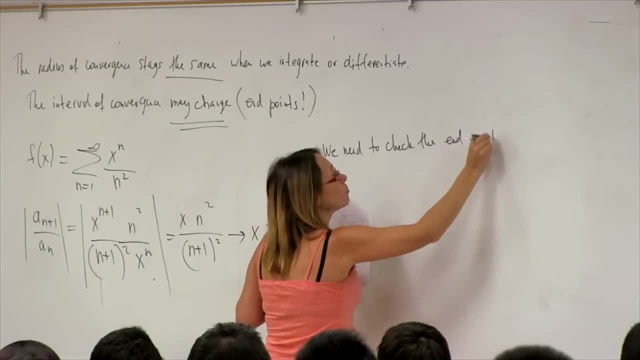 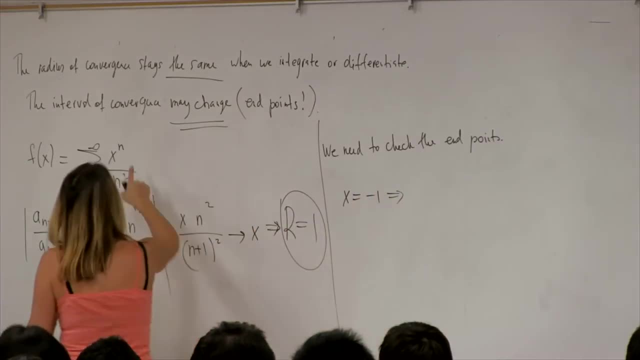 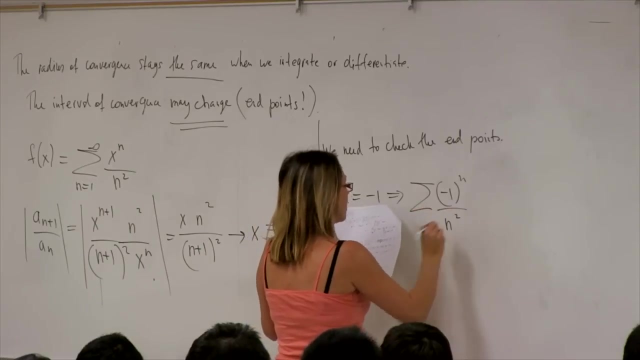 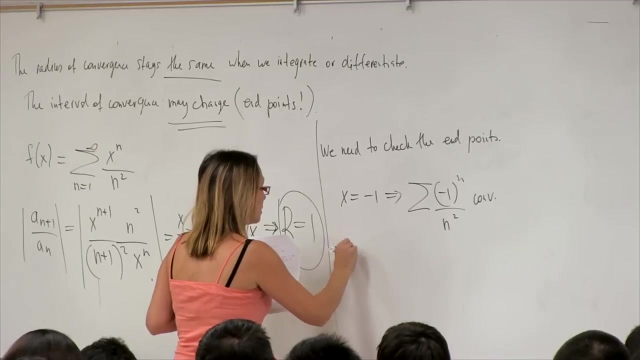 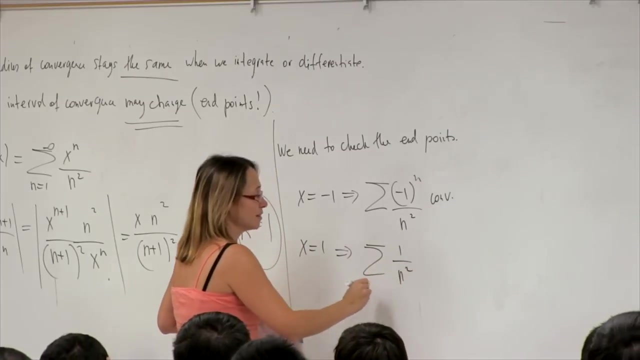 to check. we need to check the endpoints. so the first we take x, uh equals minus 1. we simply substitute it here n squared. this converges by the test for alternating series. x equals 1, uh, we have 1 over n squared, uh, does this converge? 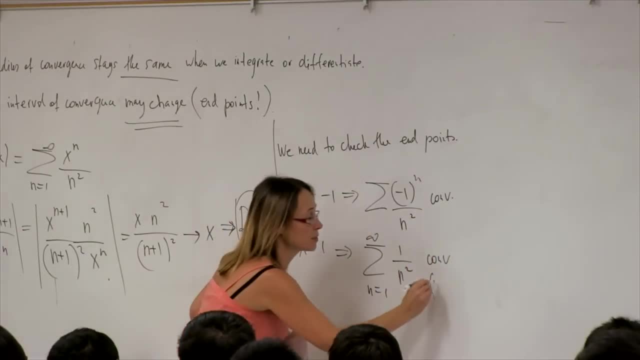 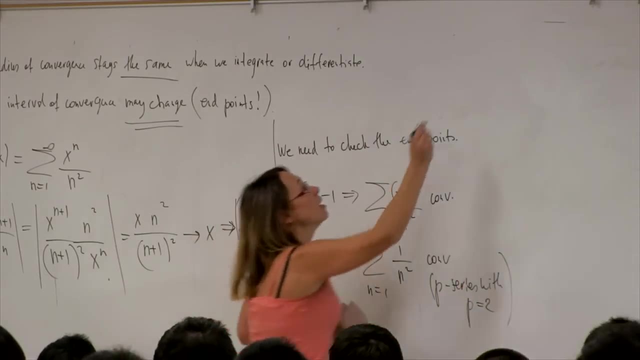 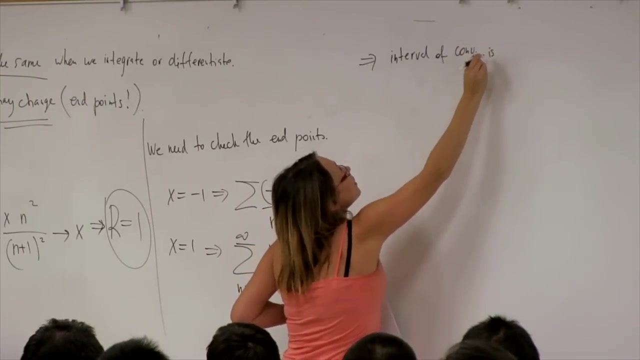 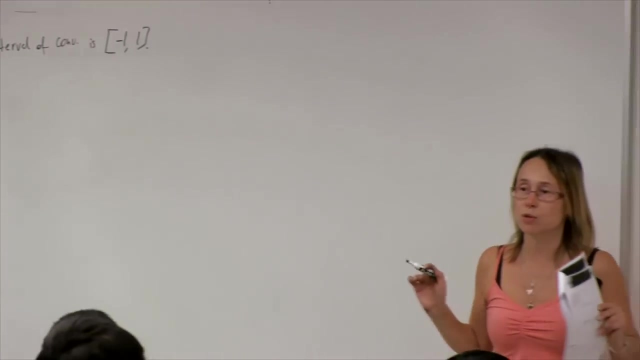 uh also converges because it's a p series. p series with p equals 2, so the interval of convergence is minus 1, 1 inclusive. it converges, uh, between minus 1 and 1 because of the radius of convergence, but also the two endpoints. 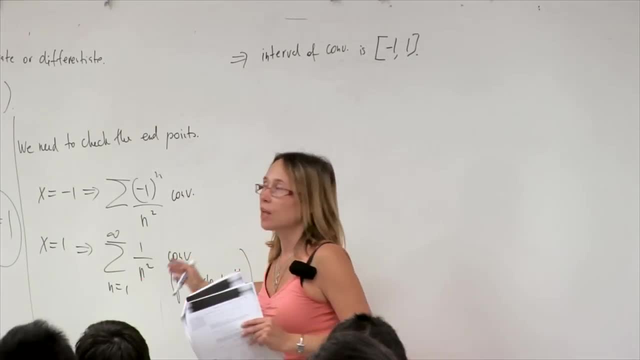 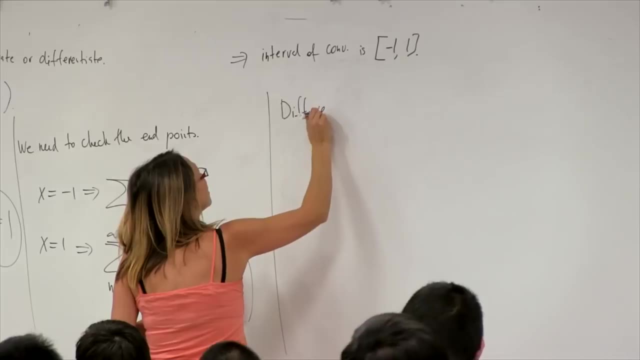 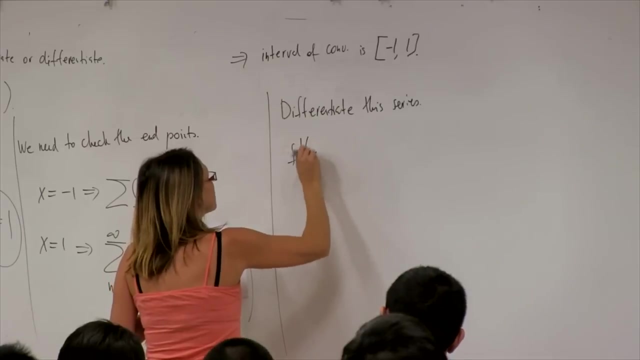 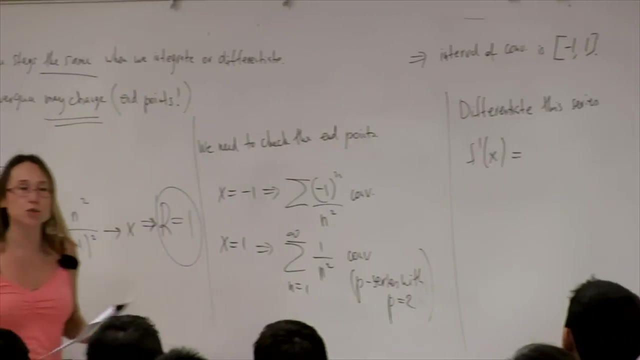 are included. we just proved separately. we made a special deal for them and, yes, it converges. now i'm going to show you what happens when you divide this series. so f prime of x. we are going to calculate f prime of this. uh, we can differentiate term. 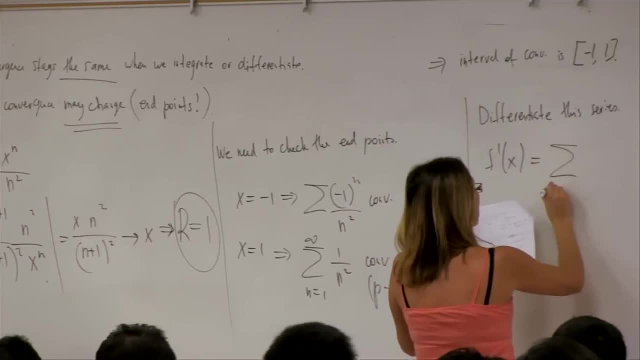 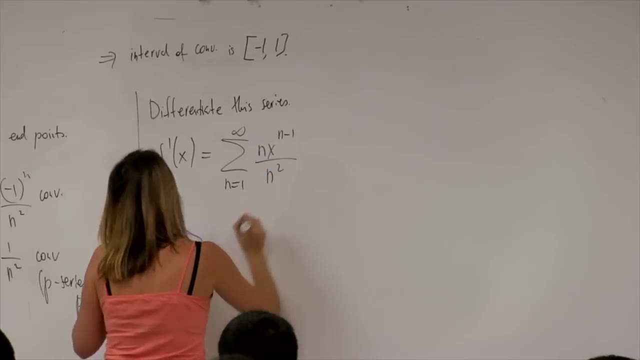 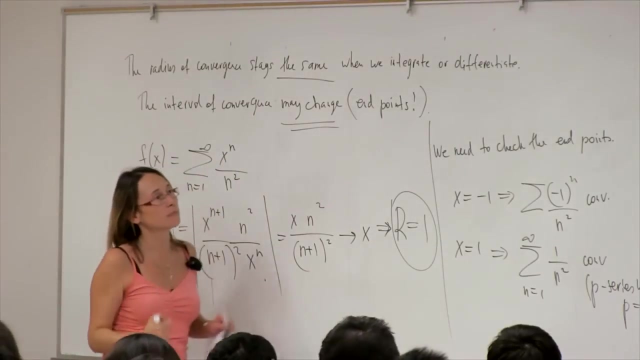 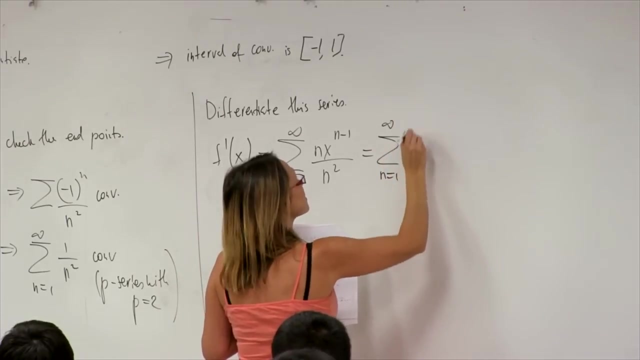 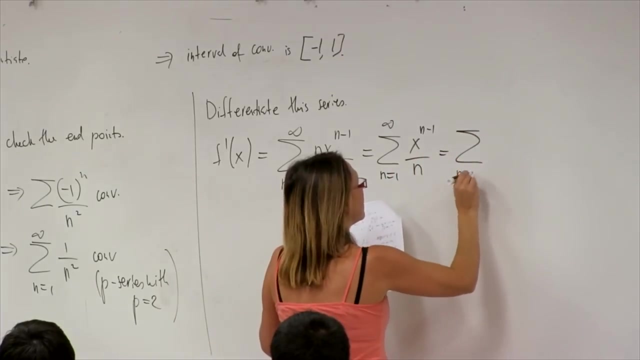 by term uh, inside the interval of convergence. so from n, uh, from 1 to infinity, n, x, n minus 1. we get n, x, n minus 1 by the power rule and n actually cancels. we get a simpler expression which is x- n minus 1. 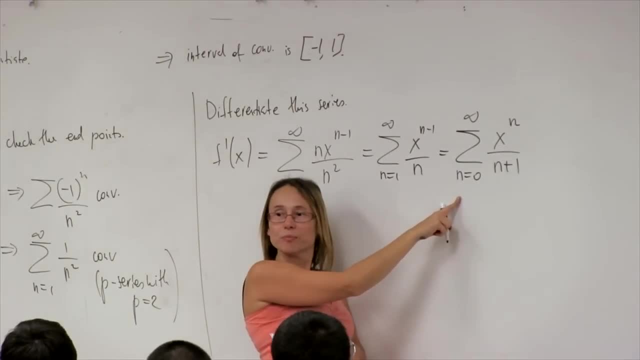 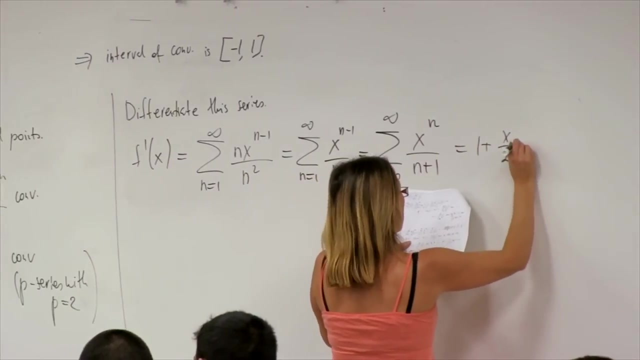 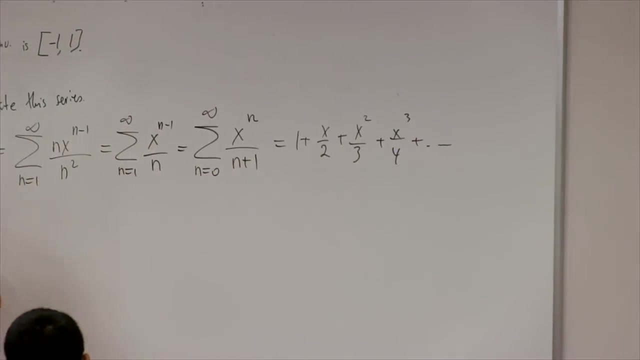 over n, or i can start from: n equals 0 x and then change everything and it it, uh, and then ends up looking like this: so this guy is equal to 1 plus x over 2 plus x squared over 3 plus x cubed over 4. 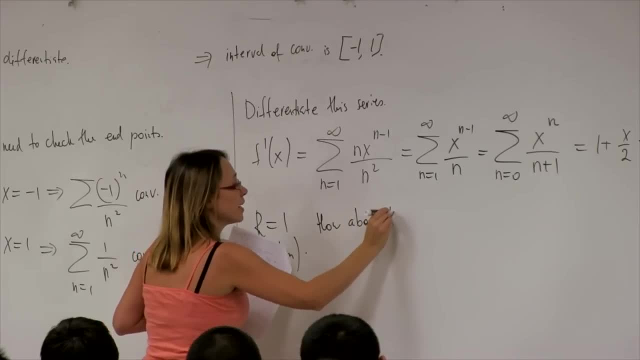 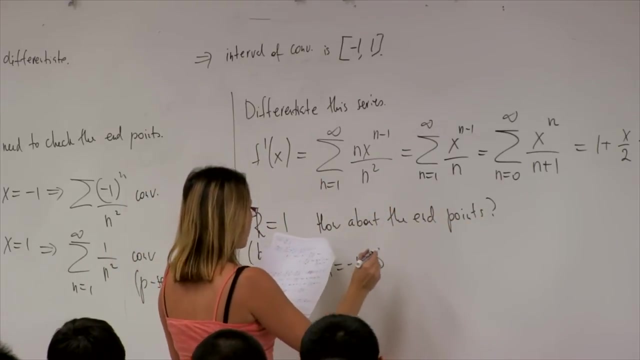 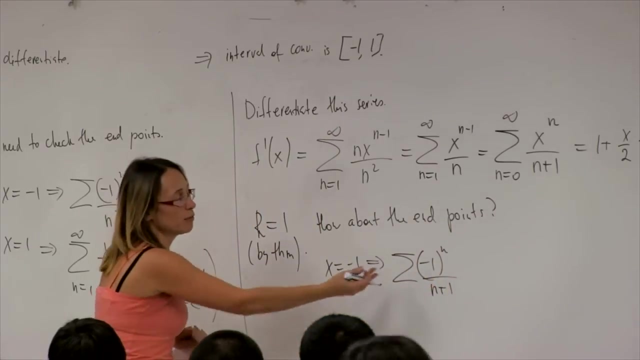 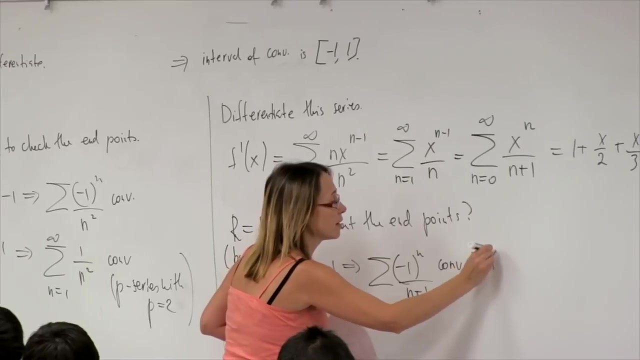 and so on. so i know by theorem that the radius is equal to 1. so first we check: x equals minus 1. so we take this power series and substitute minus 1 instead of x. okay, so we have this nice series which actually converges, uh. 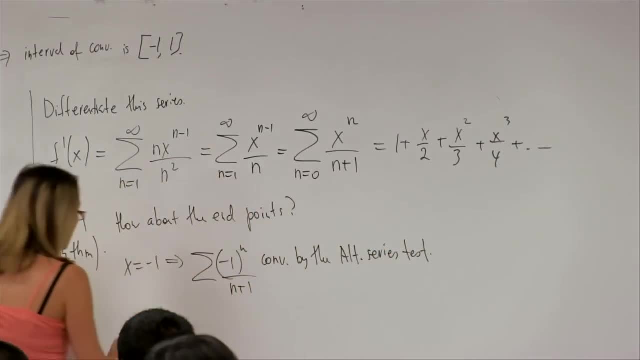 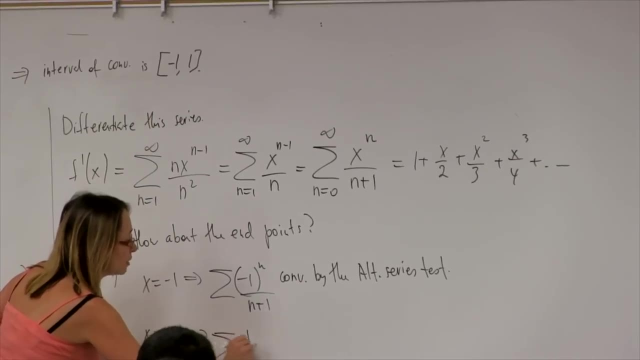 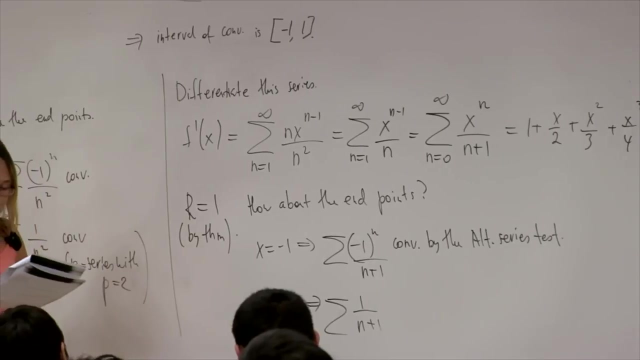 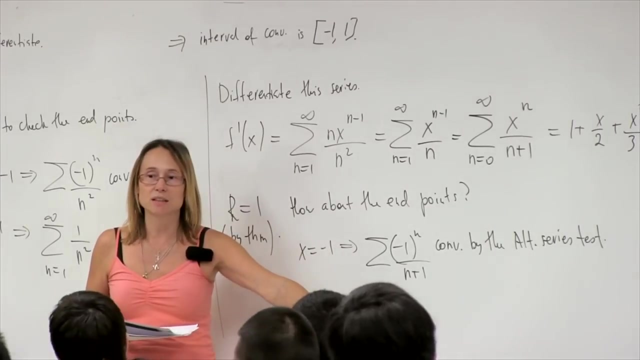 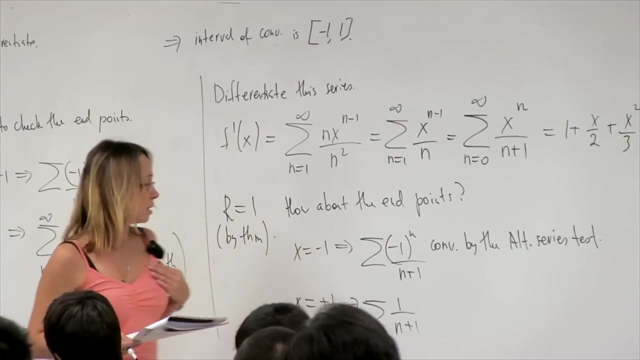 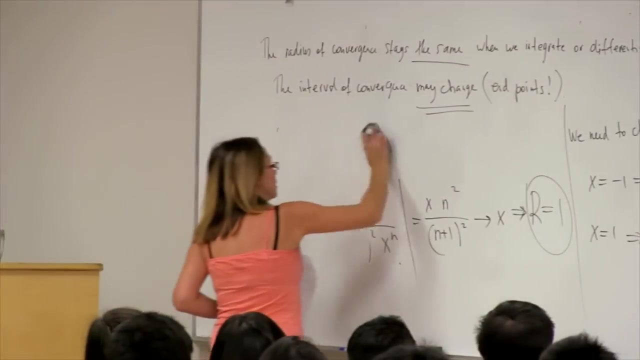 converges test. finally, we check: x equals plus 1 and that gives me 1 over n plus 1. does this converge? does this converge? so there is a few, there are a few ways to check that you. oh, i'm sorry, so what was it? oh, 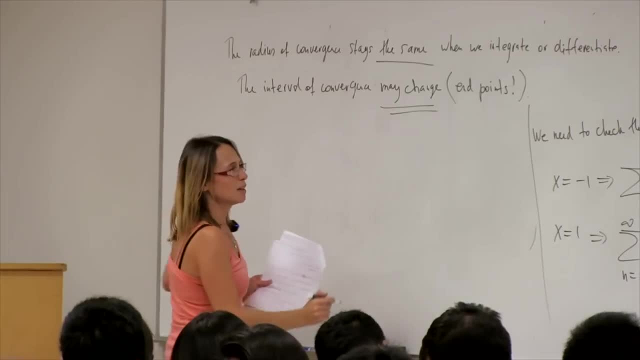 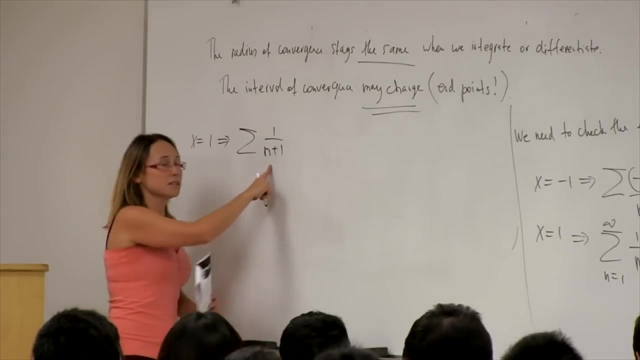 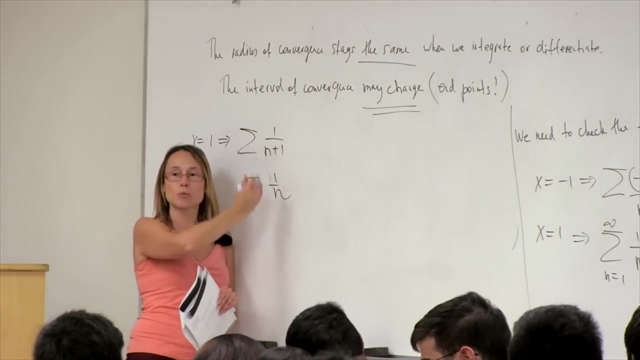 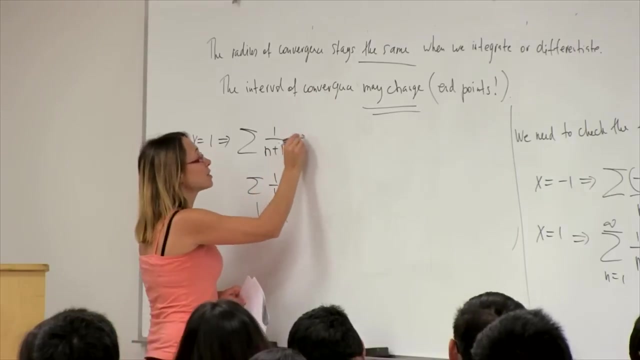 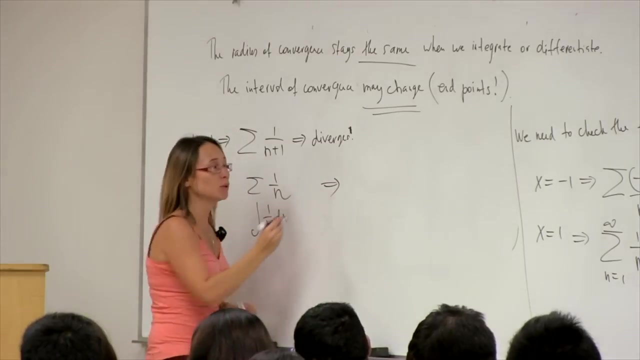 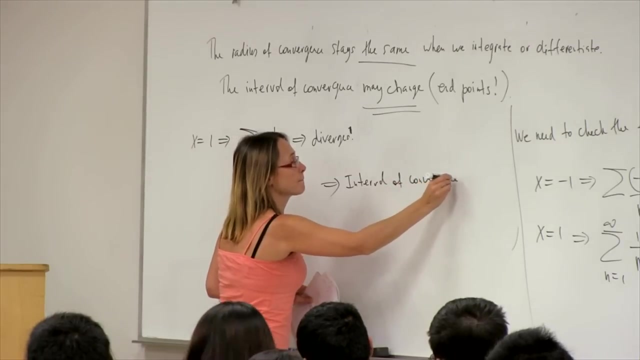 x equals 1. i have 1 over n plus 1. this is very similar to 1 over n, and you can use an integral test for 1 over x dx either. i will tell you that this diverges. so what is the interval of convergence?